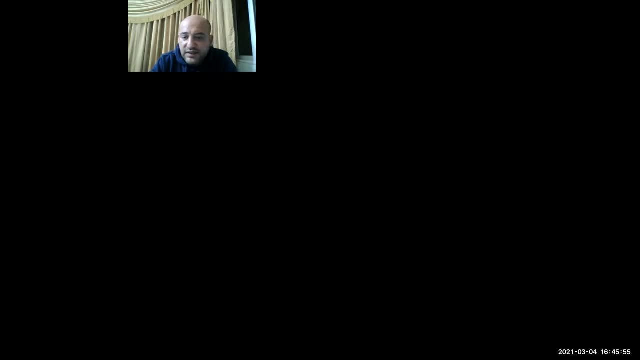 The remaining part is easier And I believe we will finish earlier than schedule, earlier than schedule. So let's see, So let's start. You'll receive the class note number seven And the handouts. also, I put handout, I believe, six, seven and eight today. 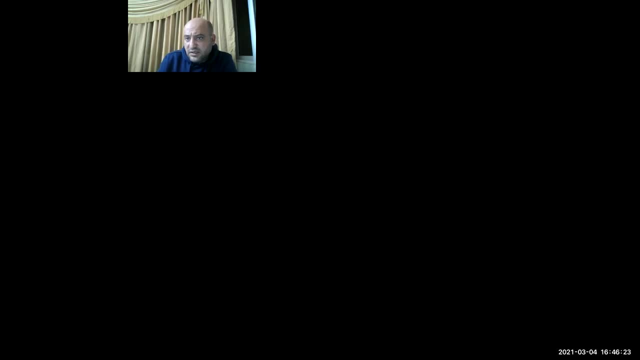 So we are in good standing. Let's see what's here. I had a question regarding the presentation My group is presenting next Thursday, Yet we have not received any information on what the presentation should be. Okay should include what we expect the instruction to be released. 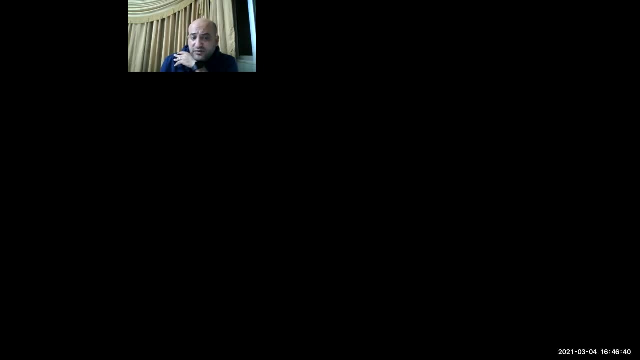 Also the instruction of writing the report. The report should have certain format. No, it's not unfair. It's not unfair Because, as I told you, you will be marked on what you are presenting And, on the other hand, the report. 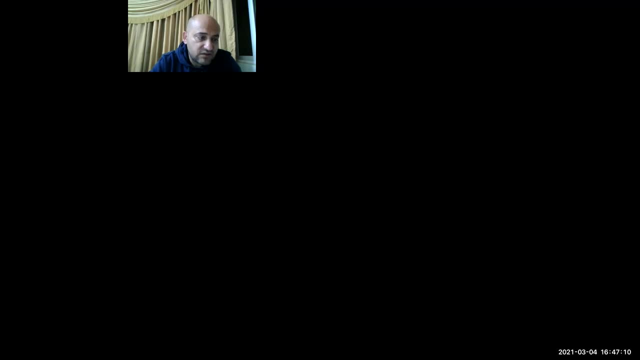 it has the same deadline for all students And the most weight is in the report For a presentation. you have a topic. You have to talk about the parts of your topic. You have to talk about the parts of your topic Each student should present. 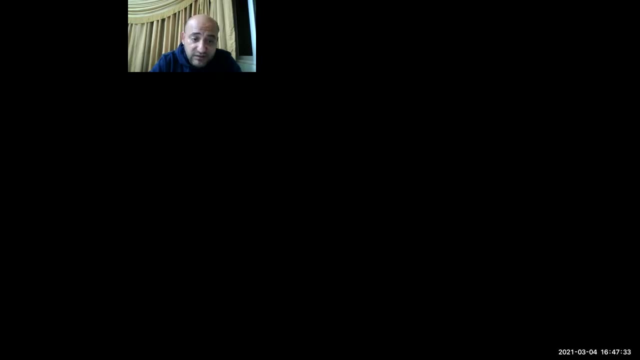 Each student should present. The presentation will be recorded. The presentations will be recorded. However, it will not be released due to because I need the camera to be open, But due to privacy. it will be kept for the course record only. 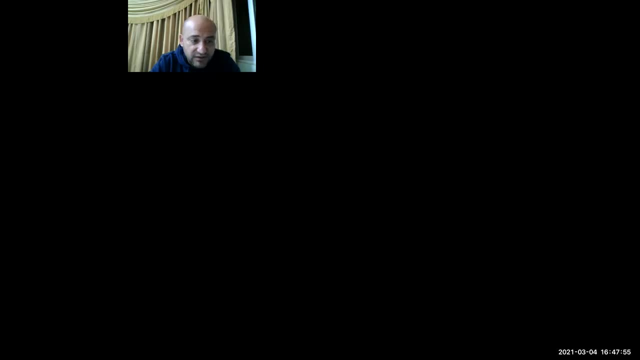 So it will be confidential data. It will not be released to any other party Or it will not be posted on YouTube. I didn't say there is instructions for the presentation guys. I clarified this. since the class one Each student should present. 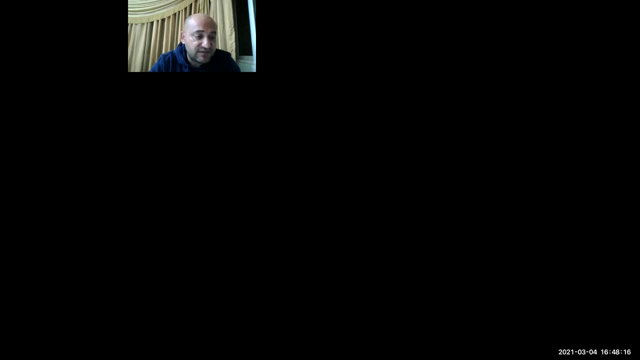 I don't want to like X to present half of the presentation and the remaining present like the other half. It should be equally Like. we have a four group member and we have four topics. Each one will talk about his topic. Each one will talk about his topic with a limited time, with equal time, to be fair with each other and the other instruction. 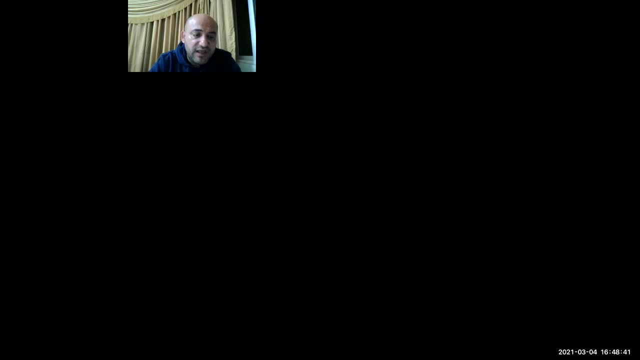 Also- I mentioned it a lot- that each member of the group should be able to answer any question about what you are presenting. So I'm not expecting, for example, for the first group who is presenting to present every single deep details about that topic. 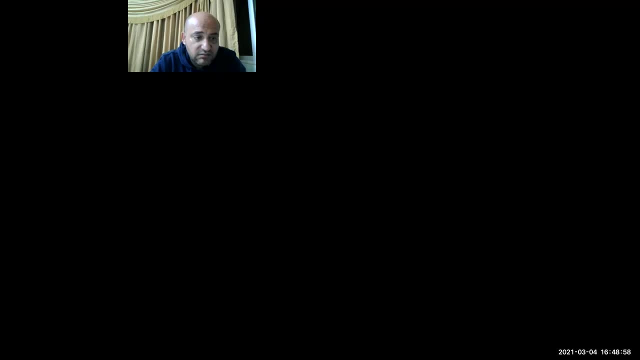 So I'm not expecting, for example, for the first group who is presenting, to present every single deep details about that topic. Whatever you read about the topic, Whatever you read about the topic, Whatever we reach to this point- and we need to present what we reach at- 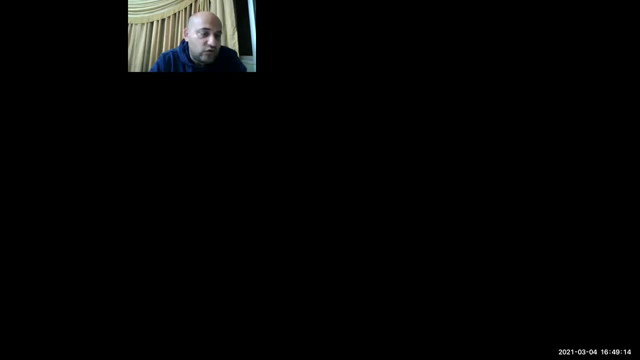 Yes, yes, And to make the thing easier for you guys, I chose to pick from your curriculum. I didn't choose a very high advanced topic. I go to the course outline and pick the topic from your course outline. I didn't ask for anything. 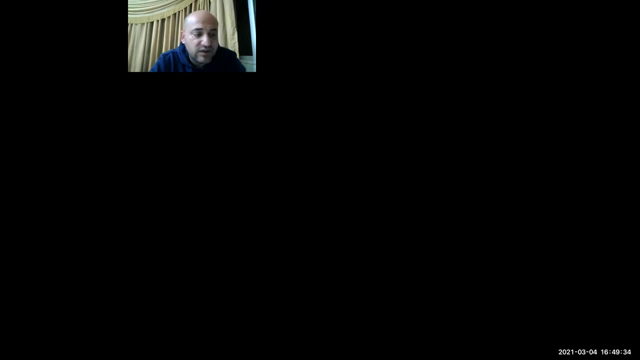 You will not be Totally during this course, for first group will represent next week, for for first group you will do whatever you reach at. Our topic is talking about this one. We plan to Investigate, explore 1234.. However we reach at this point. 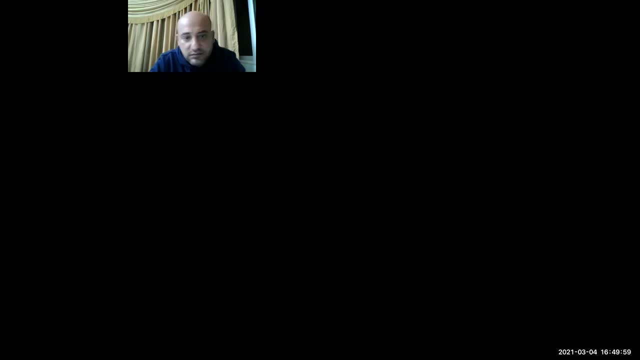 X will present this. Why would it present this? And I will. And I will ask you about the point you are reaching at. So don't tell me it's unfair, Is that clear guys? I'm not asking you to fulfill all the topic. 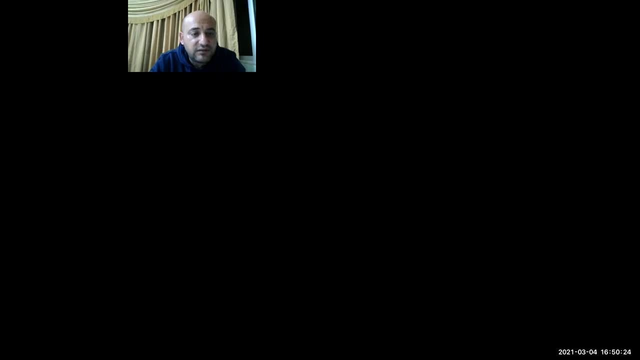 I need the whole topic to be Covered in your report, Not in the presentation. But those are groups. Who's near the end of the chair? You should be almost complete. I'm not saying fully completed because you have to The due date in April. 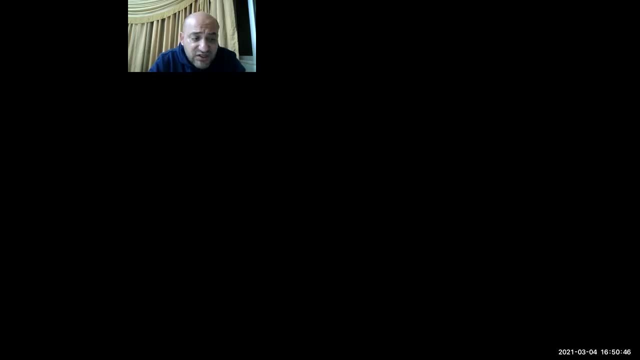 In the report. I need you to do that for the instruction of the report. It will be a formatted question, A format instructions. What is the phone? How is the format, How to write your report? That's it, But for the topic you. 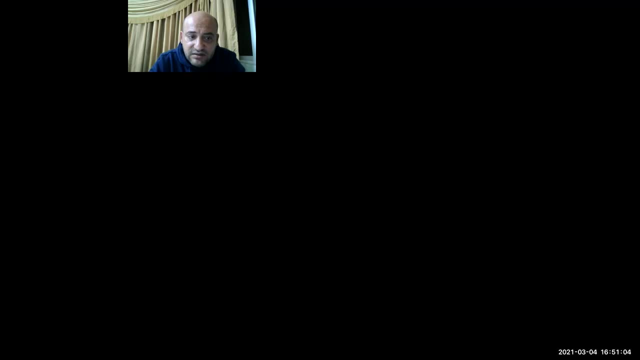 Have a topic from your curriculum At least. At least You have to cover what we have in the class. At least you will have To cover the topics that we will have in our course outlines. If you are at extra, that would be a bonus. 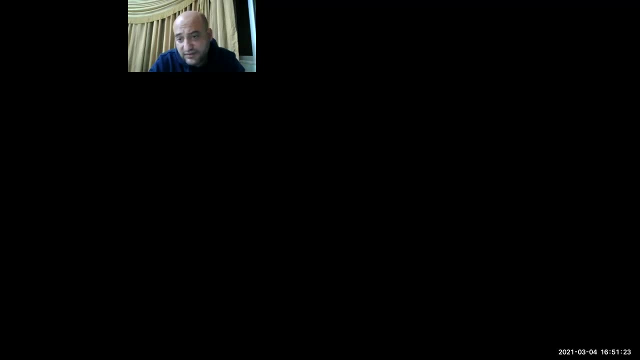 So the minimum requirement is what we are taking in the course outlines. This is the minimum requirement. Let's say To get 80 to 90 mark. You will do whatever in our course outline. You do extra, You will move to the nineties. 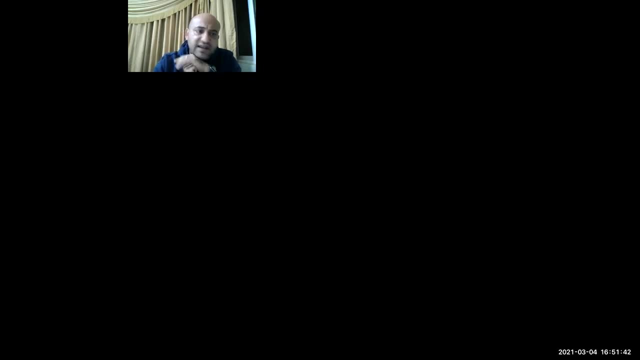 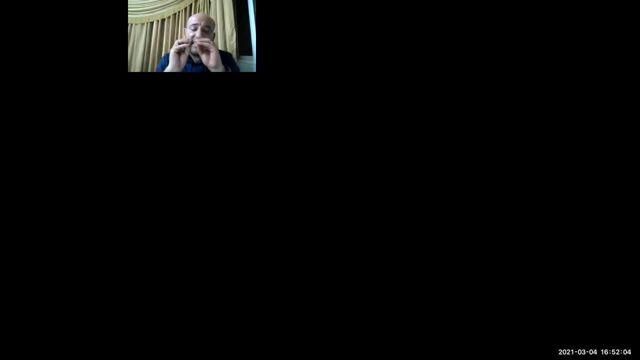 They try to like make it like an English literature presentation. They try to like make it like an English literature presentation. No, simple language, straightforward So everybody can understand. And the main component: I need to know that- That the student in the group they understand the topic. 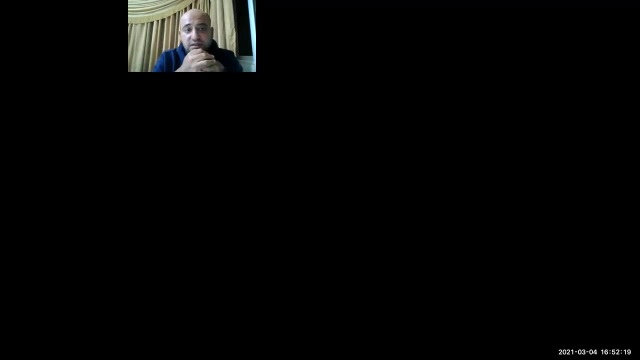 And they can transfer their knowledge to their colleagues. So I'm looking for the benefit of the presentation, of the presentation content itself. Don't make it complicated, Okay. So I believe this is a clear. So I believe this is a clear. So I believe this is a clear. 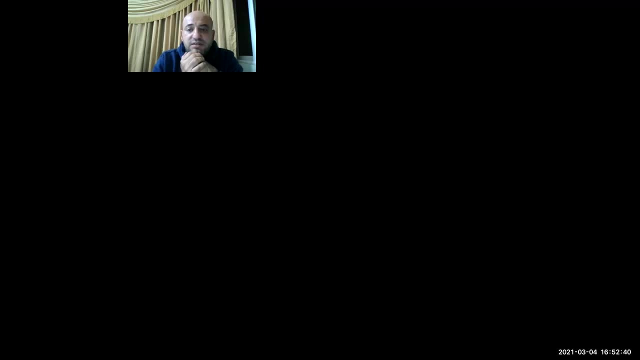 Any other question? The presentations that will start next week For the arranging, We'll start first to second. I leave it for that. I don't go to that deep details. I leave it to the group. You are a mature student. 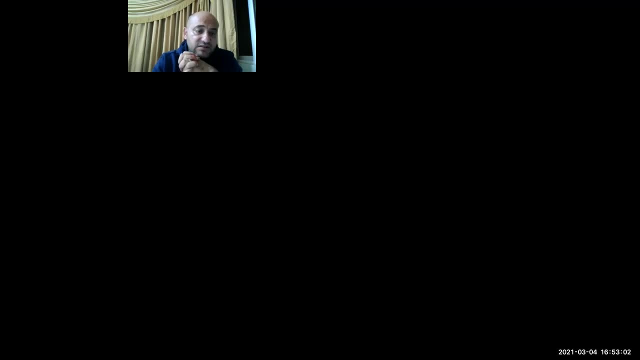 And you know how to organize your solo. And you know how to organize your solo And you know how to organize your solo, organize yourself. and it's a kind of an experience that if you have a group presentation at the work site later on after graduation- hopefully next year or the year after for those who 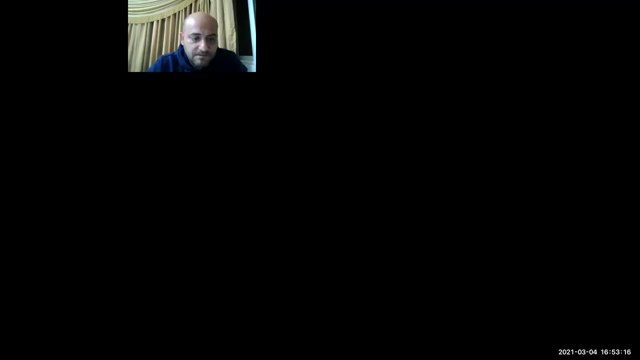 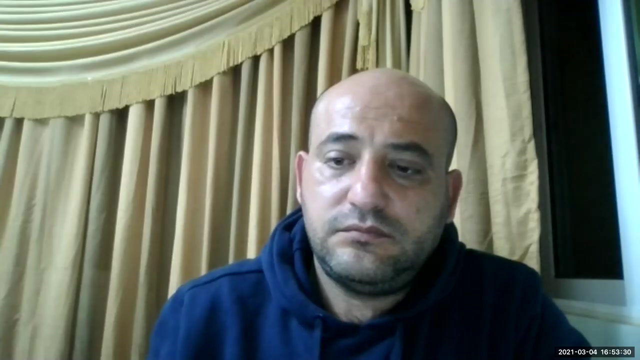 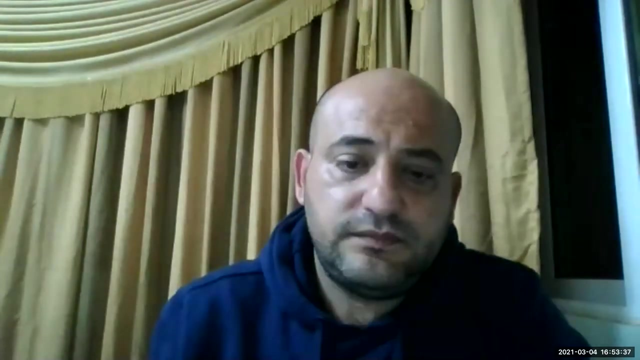 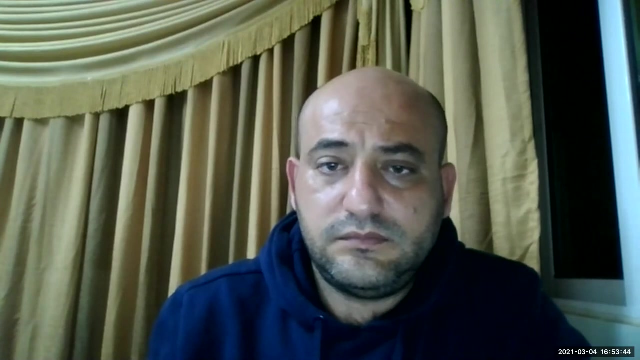 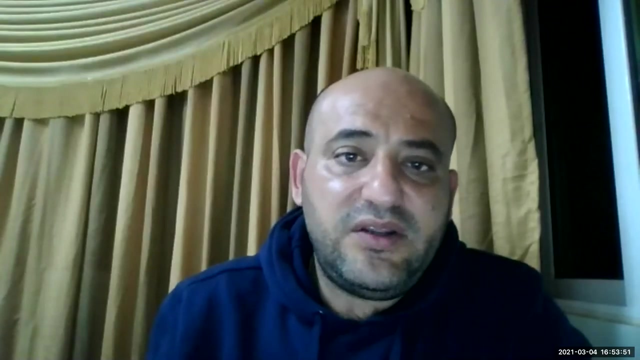 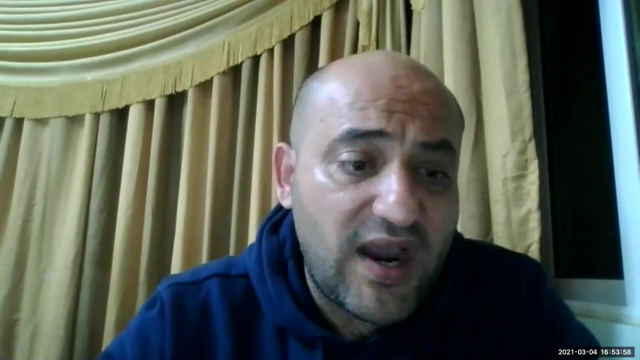 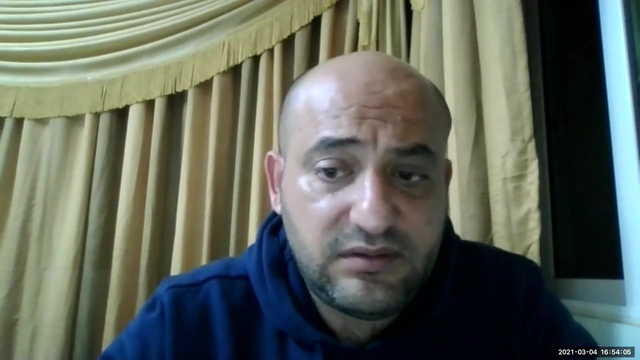 will go for internship for one year. clear guys. great, Sean. you sent an email to the TA. I just explained that. at the beginning of the class, Sean, I said the mark you are seeing is the multiple choice mark for the second question. it's not mark yet. it will be a hand marking and your mark will be updated. I just mentioned that at the beginning. 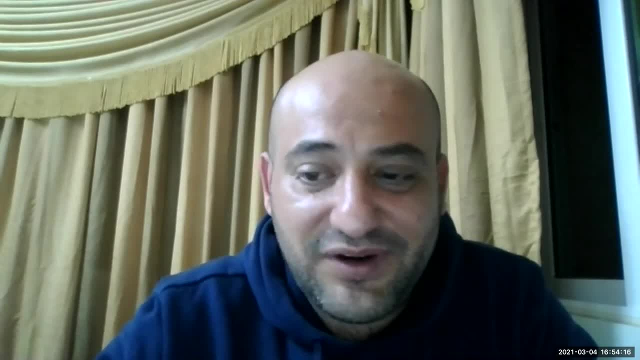 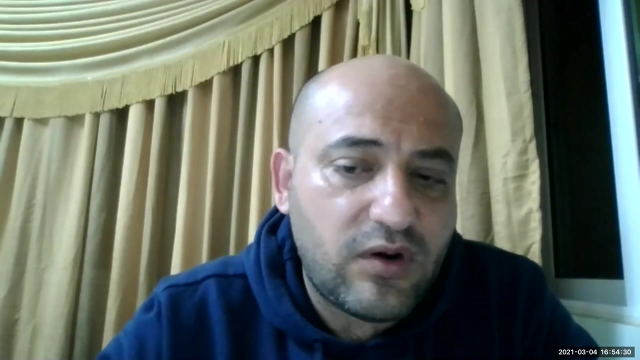 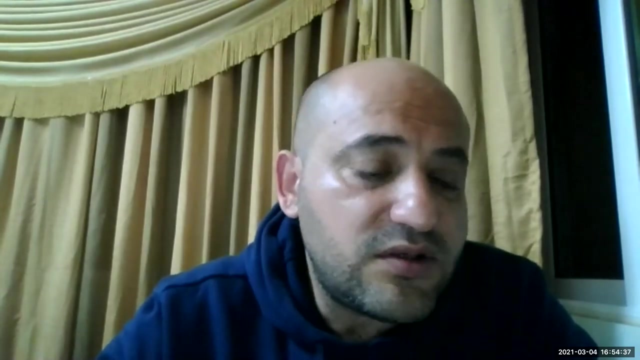 of the class. I just received your email. okay, I understand. also, I mentioned that in the quiz during the quiz. maybe you were busy or don't hear that. so the mark you see in your grade book again, for all students, the mark you see in the grade book is the multiple choice mark, because I put the right answer in owl so I will mark. 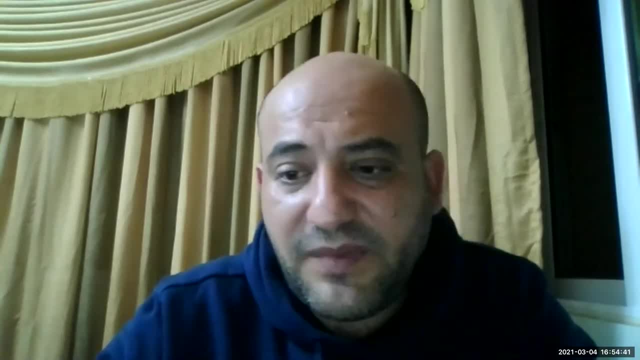 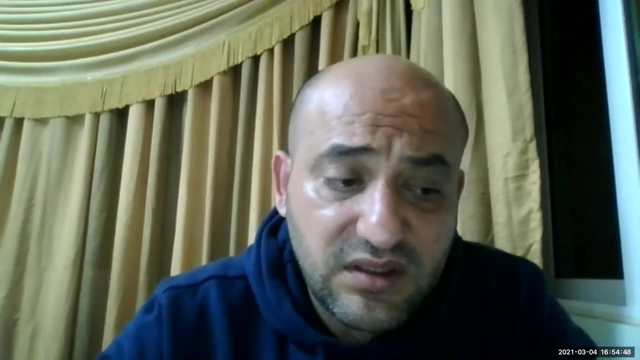 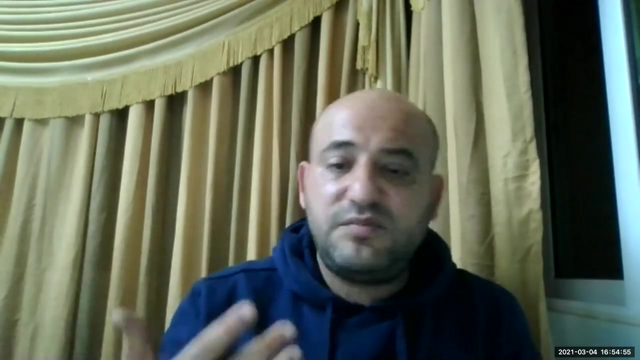 your multiple choice. for the second question. it will be marked manually as of next week because, as I told, we have some technical issues, some students, we have for them two answers, some of the students make a couple of submissions, so this version, like for multiple choice, could be merged and I need from our technical team to send me the both answers. 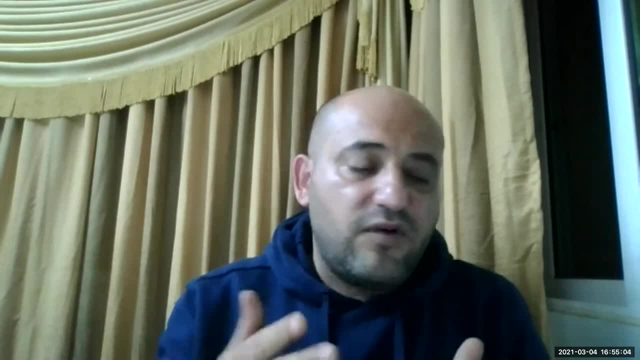 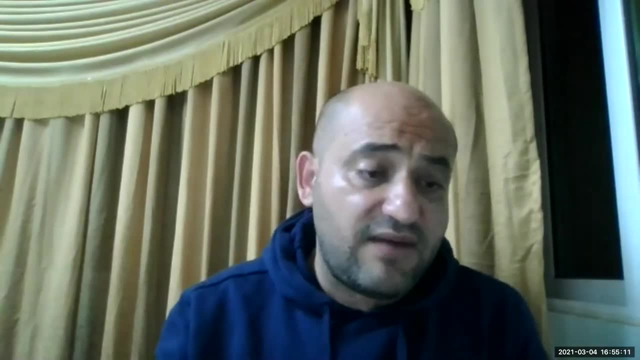 for those who answer twice or for those who do a couple of submission and that their longer question answer it's in their first submission. I don't have it, this version, So they promised to send it to me as soon as they can. Everything is recorded, don't worry. 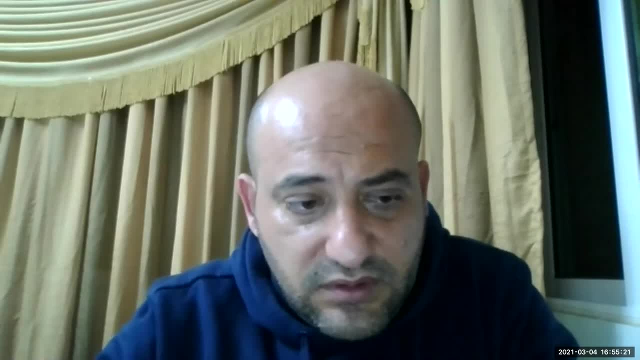 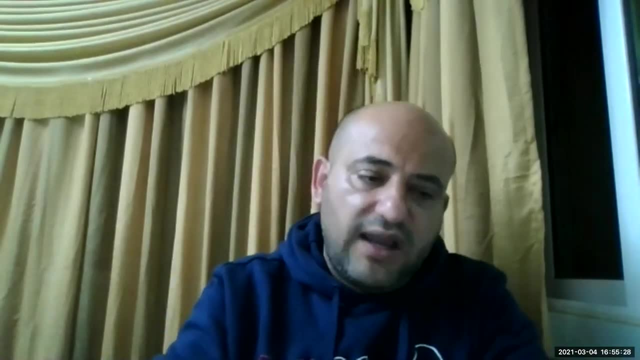 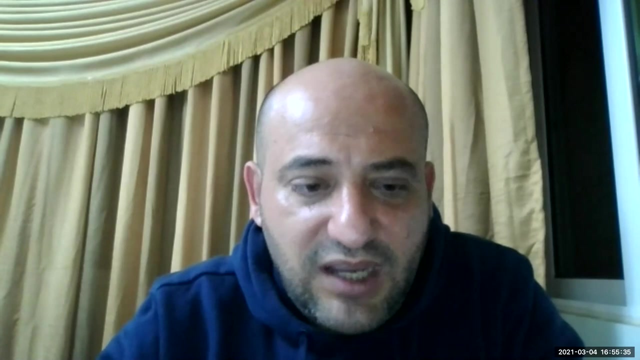 You will not miss any single letter you wrote And if we found that technical problem, still some students- it was unfair for some students. I can make a makeup longer question or do something to recover what they missed. So don't worry guys. 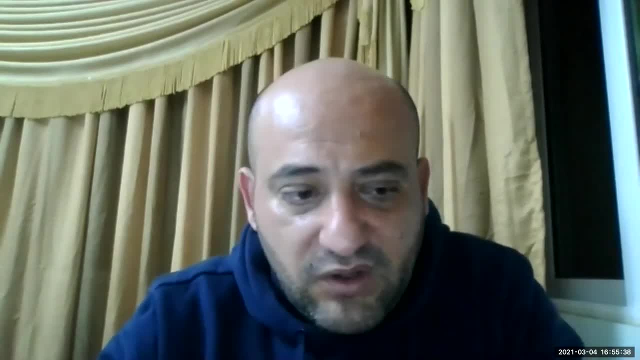 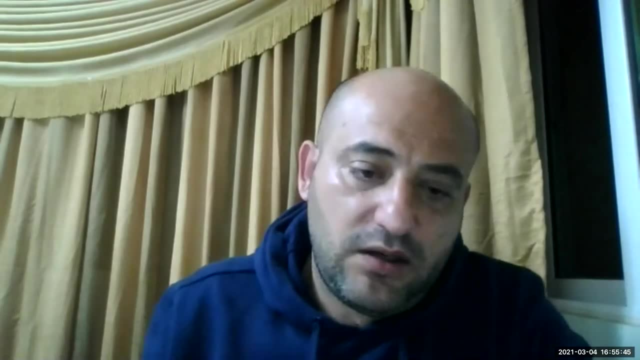 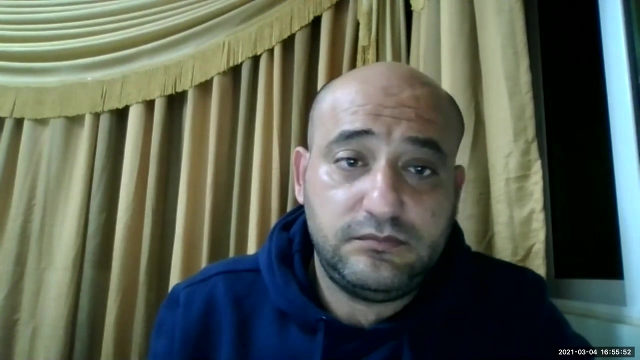 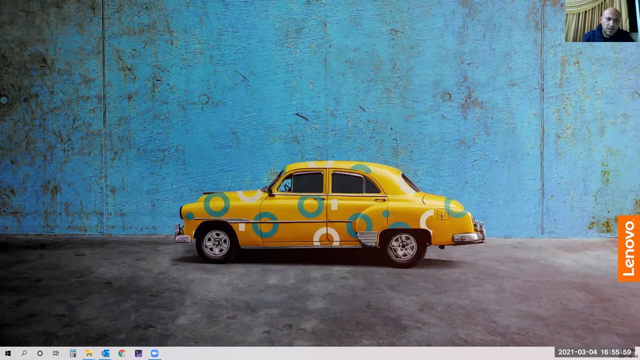 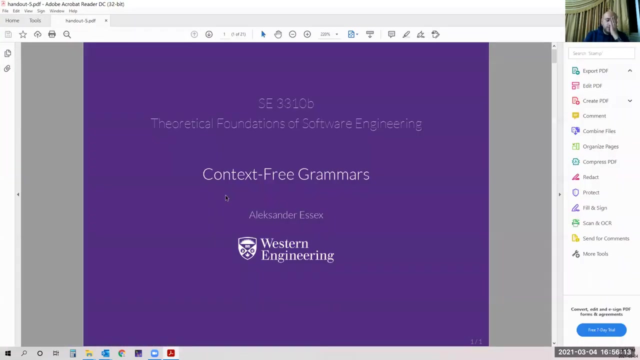 I'm not here to reduce your mark, I'm here to help you, okay, So let's start. Okay, So let's open the handout number five. Okay, today we are talking about a larger class of computational models, We talk about the finite automata. 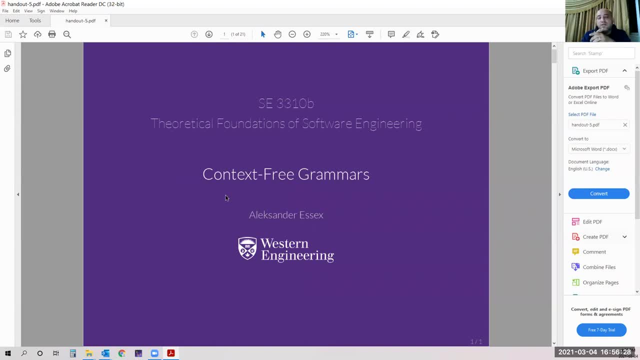 at the first part of this course, which include deterministic and non-deterministic, finite, automata, regular expression, and we prove that there are some exceptions that are not regular using the pumping lemma- And today we talk about the linear information- we go wider to have another model. 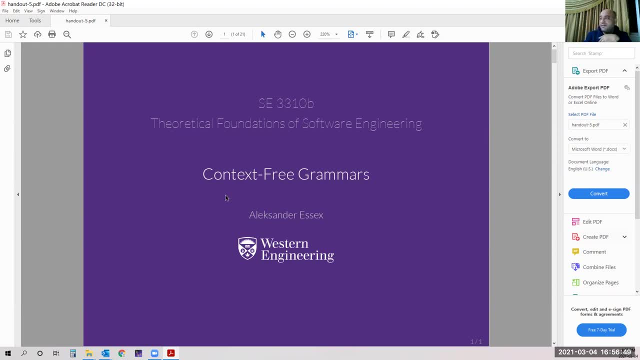 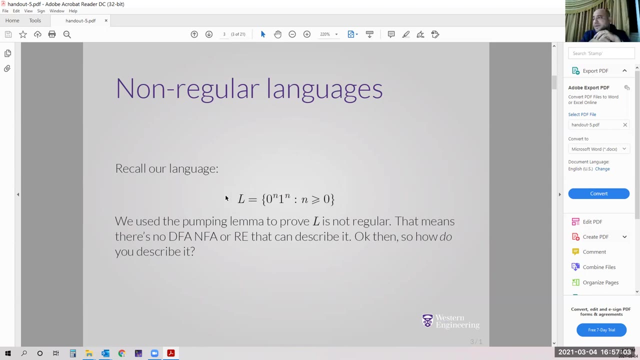 which we call it context-free grammars, context-free grammars. At the beginning, we'll talk about context-free languages. context-free languages, If you remember or if you recap from previous classes, that we call our example zero to the power n. 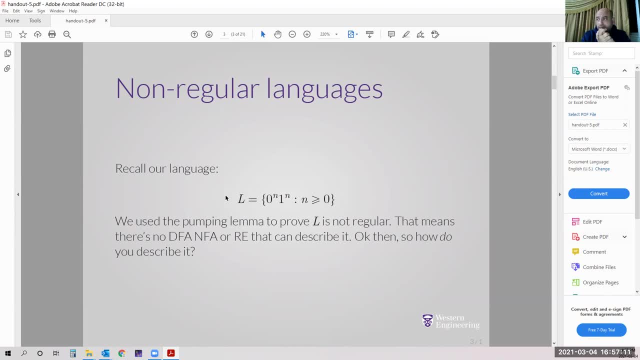 one to the power n where greater or equal to zero using the pumping lemma. and we prove that this language is not regular. That means there is no DFA or NFA or regular expression that can be described or be accept this language. So how we can describe this language? 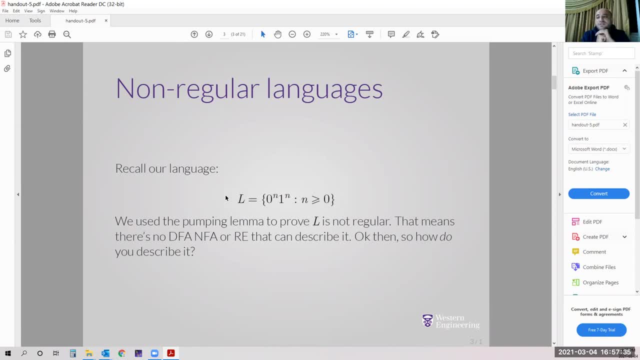 We know that the main objective of using computers or the computation system or computational model is to help humans to do sophisticated tasks as much as we can. So how we can expand the computational model to include these non-regular languages, How we can do that. 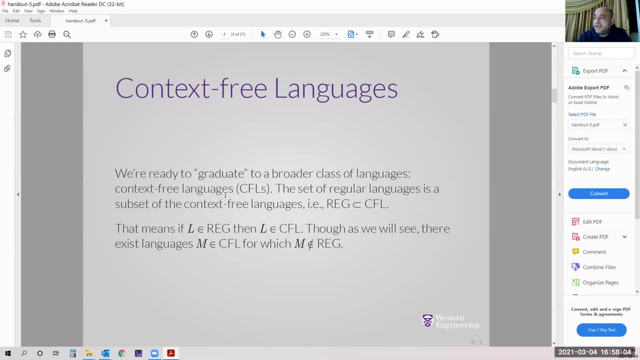 We use what we call context-free language. We're ready to graduate to a broader class, broader class of languages which we call it context-free languages, CFLs. the set of regular language is a subset of the context free language, So regular language are eg we used to call it before. 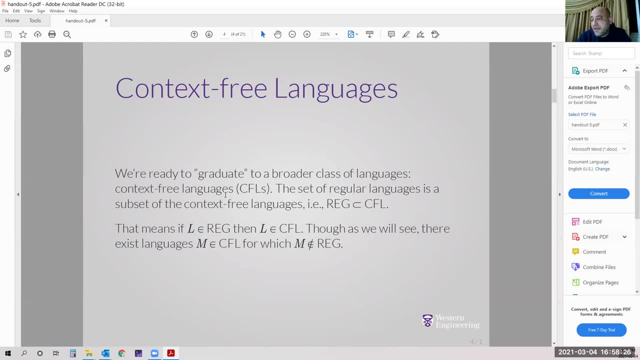 is a subset or included in the context. free languages That mean I'll belong to regular language. then I'll belong to context-free languages though, as we will. the that means you will be in contact for something else will see. there is exist language. m belong to cfl, for which m is not belong to regular language, and 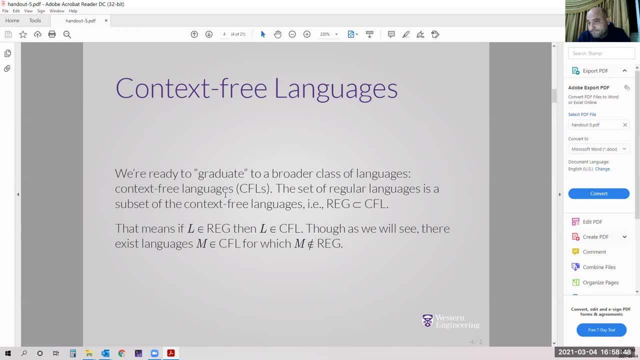 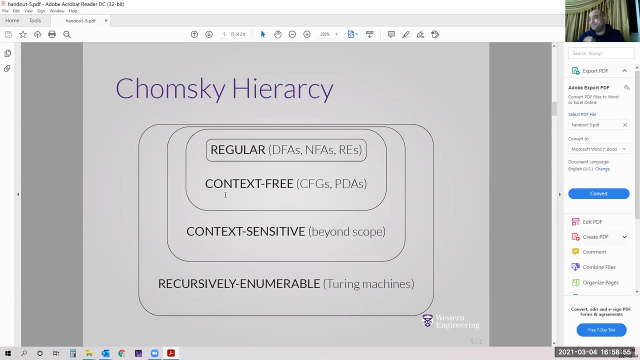 we call these languages non-regular languages and we used to prove that these languages are not regular using the pumping lemma in the previous classes. so here a small diagram and the simple diagram that show how we are limited and how we can expand the computational models to contains more sophisticated classes. so with regular language, 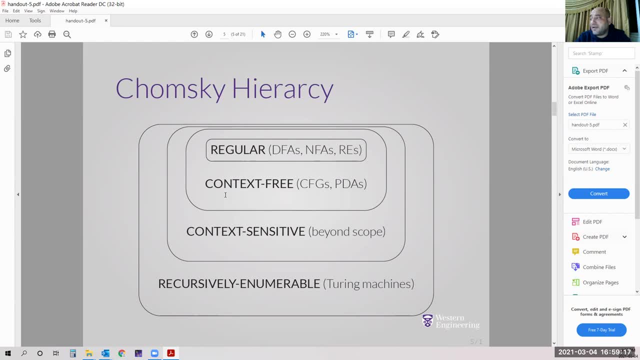 we studies the dfas, nfas and regular expressions with context-free grammars. we will study context-free grammars and push down automators, which is a very good example of how we can expand the computational models to contain more sophisticated languages, which is that broader class. then we have what we call it. 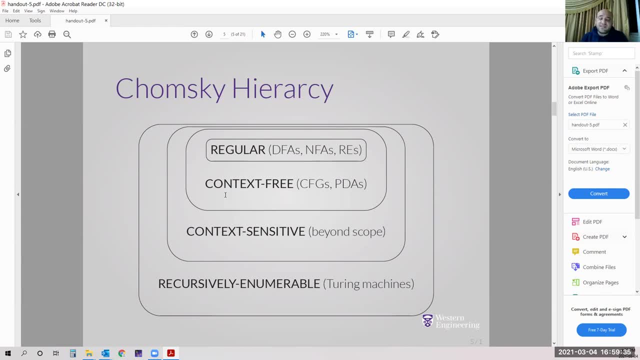 context sensitive model, but this is beyond our course scope. then we will study one model of the recursively enumerable model, computational model. we will study one model which is the toring machine. which is the toring machine then will be done and will move to the complexity part. 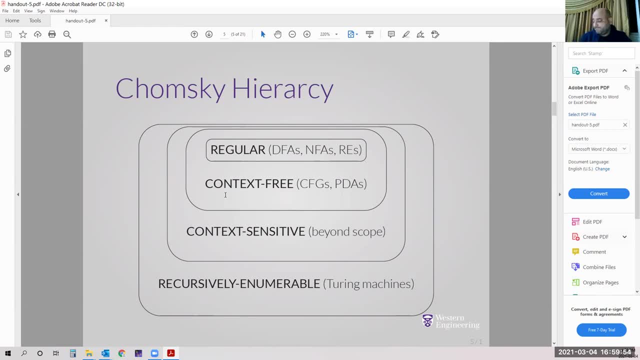 and decidability of the languages. so once we think about this, now we are going to show how the language is. the language is cuincentrico. it's very important to understand how the language is, how the language is, and sorry i didn't mention it, because it's very important for people to understand. 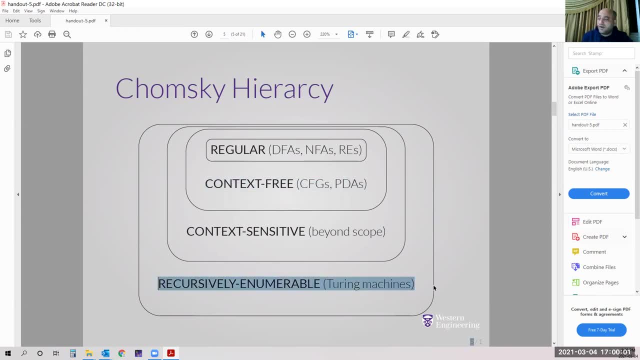 so once we think about it, let's go to the next slide. so first we're going to look at the last various, finish this one. we still have one more model, which is the Turing machine, which we will be studying. Today we'll talk about part of it and tomorrow we'll try to continue. 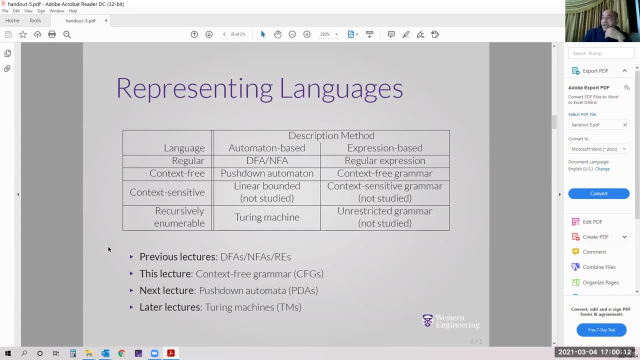 this model Representing languages. So the language: it's automaton-based or expression-based? If the language is automaton-based, it either could be automaton-based or expression-based. If the language is, so, we'll talk about the language. is it automaton-based or expression-based? 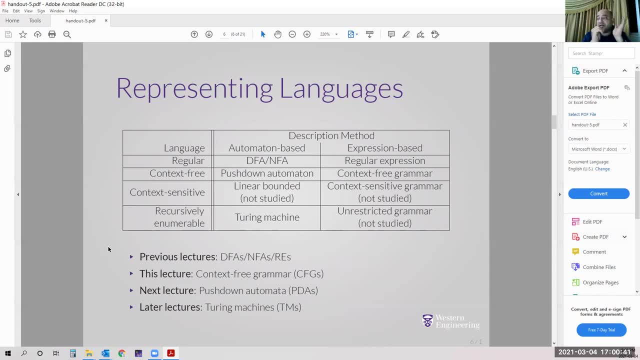 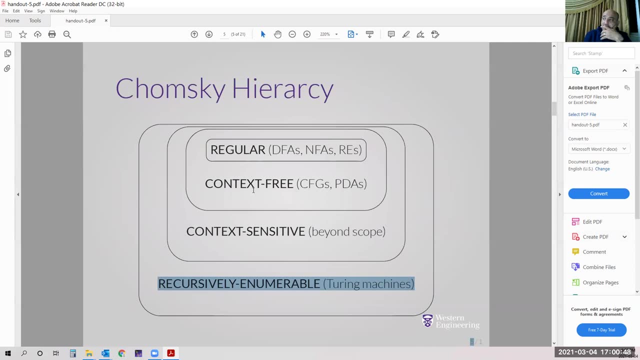 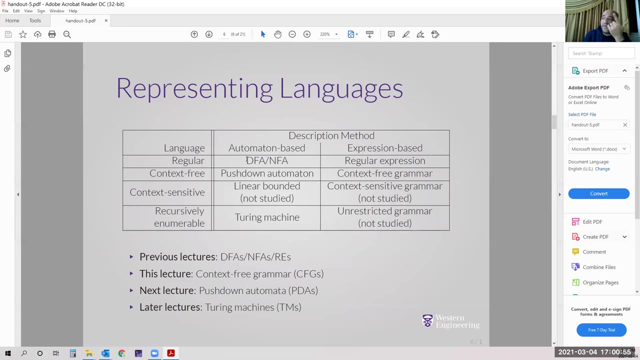 Is it regular or context-free, or context-sensitive or recursively enumerable? These are the models that we have here: Regular, context-free, context-sensitive and recursively enumerable. So if the language is regular, as automaton-based, we have the DFA and the NFA. 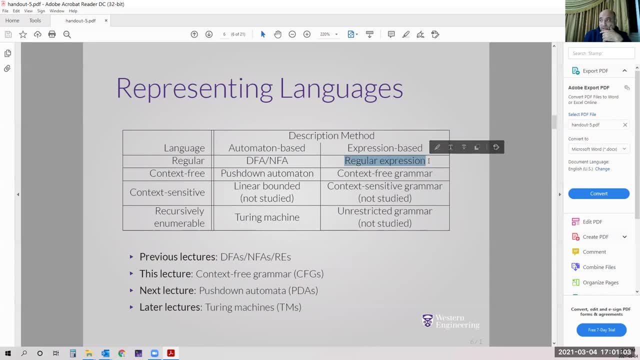 Exception-level. we have regular expression. If we talk about context-free grammar, we'll talk about push-down automaton and we go to context-free grammar, which is the depends on the expression. Context-sensitive. we have linear-bounded, not studied, and context-sensitive grammar. 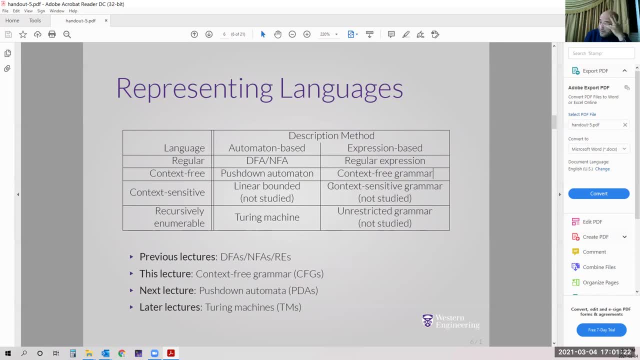 which is not studied, and beyond This one, if you study a math and programming languages, you have to take the advanced computational theory, and this topic will be covered there. Recursively enumerable, we will have the Turing machine and unrestricted grammar, which is 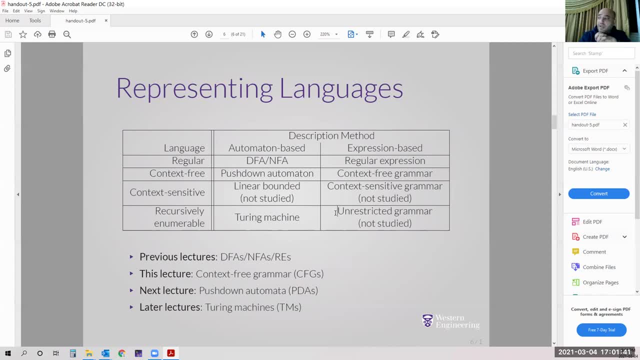 also beyond. it's a complicated and sophisticated topic which is beyond our discourse scope. So in the previous lectures we studied DFA's, NFA's and regular expression. This lecture and Part of today's lecture also, that's why we extend it and tomorrow's lecture we will 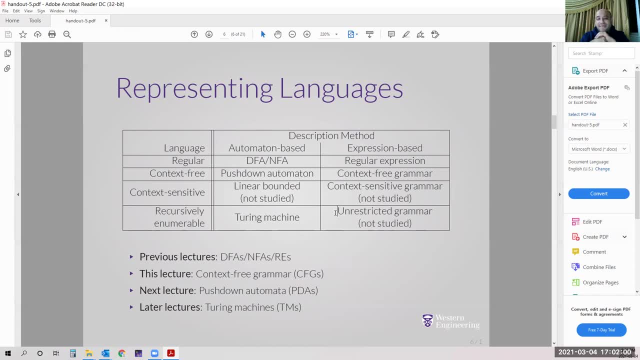 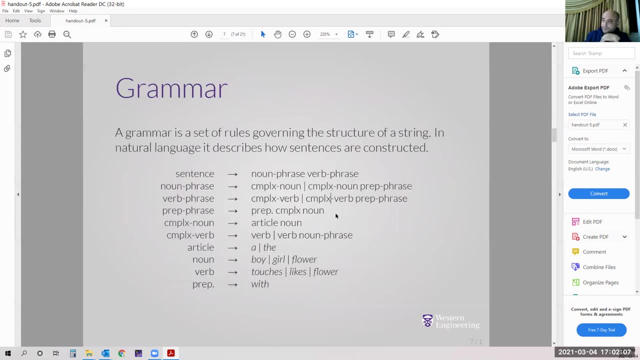 study the push-down automaton and the Turing machine And at that point we are done with computational model. then we'll talk about some complexity thing: Grammar. A grammar is a set of rules governing the structure of the string in a natural language. 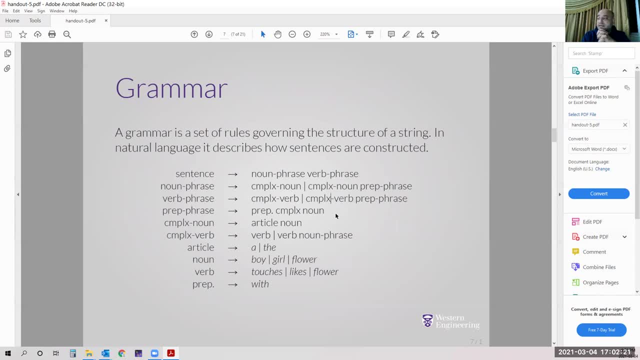 It describes how sentences are constructed. If we have a sentence- Noun, Phrase, Verb, Phrase- If it's noun and phrase, then we'll say either it's a complex noun or complex noun followed by prep phrase. If it's a verb phrase, it will be a complex verb alone or a complex verb followed by. 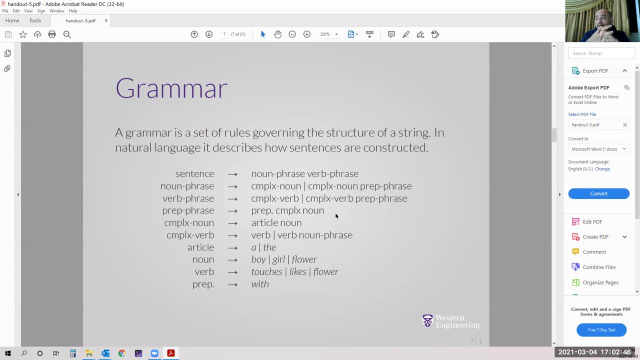 prep phrase. What is the prep phrase? It is the prep complex noun. Complex noun: it's article noun. Complex verb is a verb or a noun or phrase. Article, a letter A or the Noun is boy, girl, flower, etc. 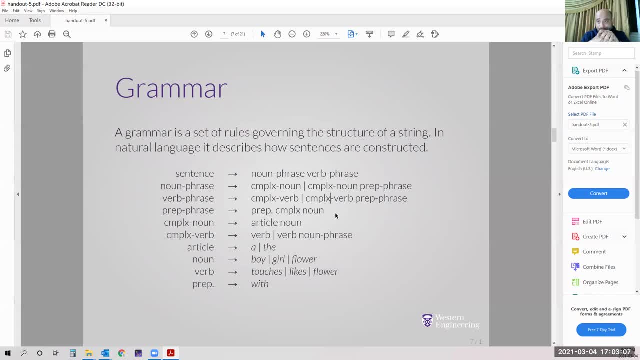 Verb touches likes flower, whatever prep with. So this is the kind of a grammar. If we are talking about natural language or the normal English, either the sentence could be consist of noun or phrase or verb, followed by verb phrase. 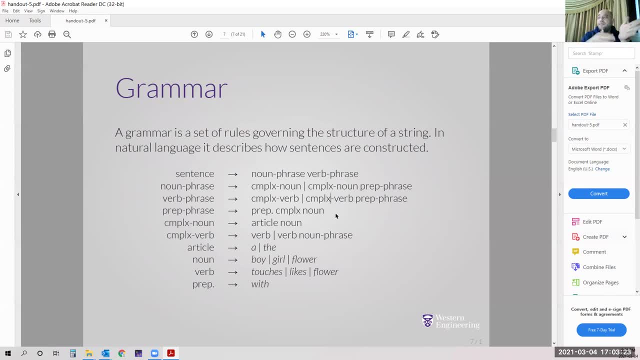 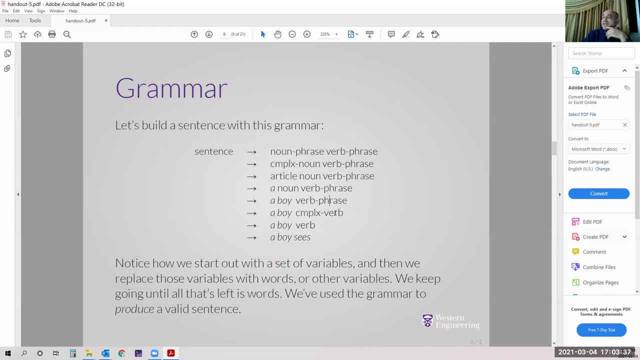 The noun or phrase could be one, two, three, the verb phrase, etc. So this is the way that we put the rules of the grammar. So we'll follow the same model to talk about context-free languages. Let's build the sentence with this grammar. 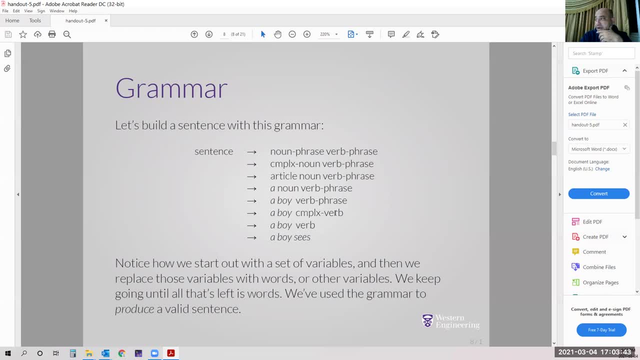 Noun phrase verb phrase: complex noun verb phrase. article noun verb phrase: a noun verb phrase. So we replace the article with a Then a boy, which is the noun verb phrase. a boy, complex verb. a boy verb: a boy sees. 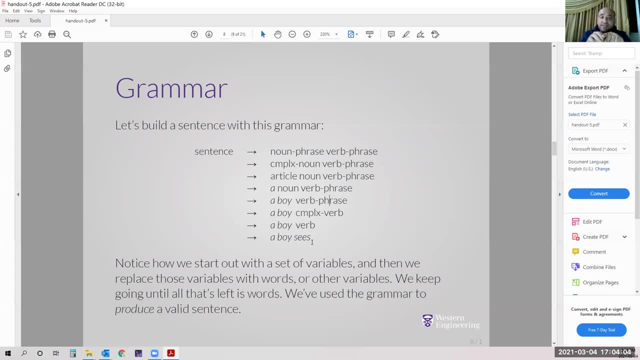 So this is how we follow. As you know, from the first class, we said that the computer is a machine, So we have to give it each simple step that we may do as human in order to do the computational model correctly And we have the correct output. 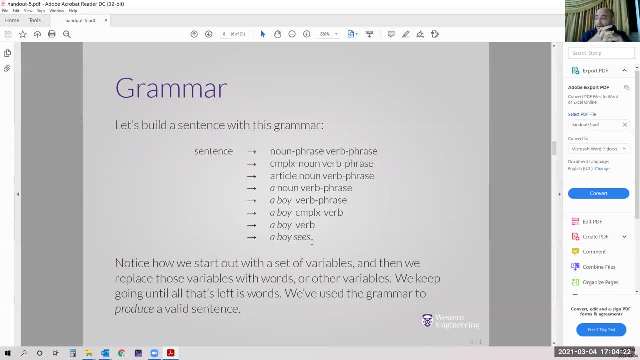 So not How. we start out with a set of variables, We call these variables, and then we replace those variable with the words or other variables. We keep going until that's left. That's left is words. We have used the grammar to produce a valid sentence. 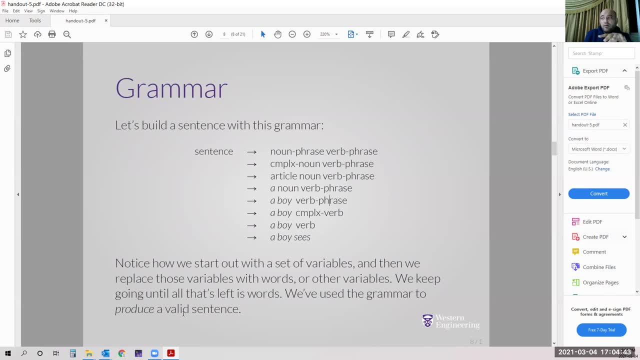 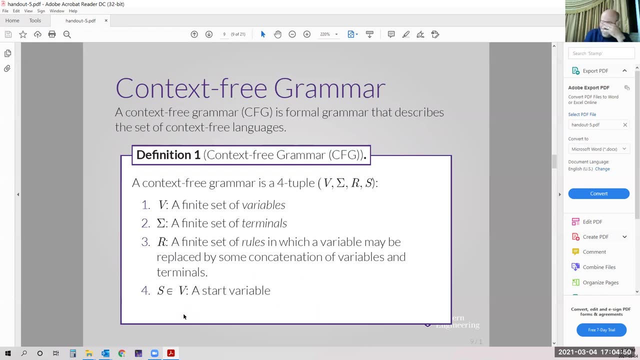 These are the steps, guys. We will see now how. I'll give you a lot of example to let you understand. Okay, One we say about context free grammar and programming languages. What does that mean? A context free grammar, CFG, is a formal grammar that describe the set of context free languages. 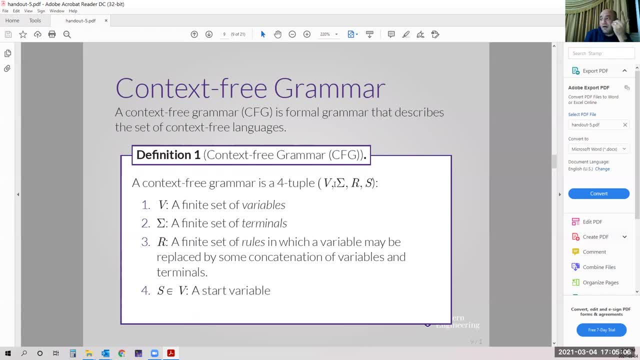 A context free grammar is a four tuple, which is V, Sigma, R and S, V, which is the variable of finite set of variables. If you want to say, It is something, For example, It is something similar to the alphabet with regular expression: Sigma, a finite set of. 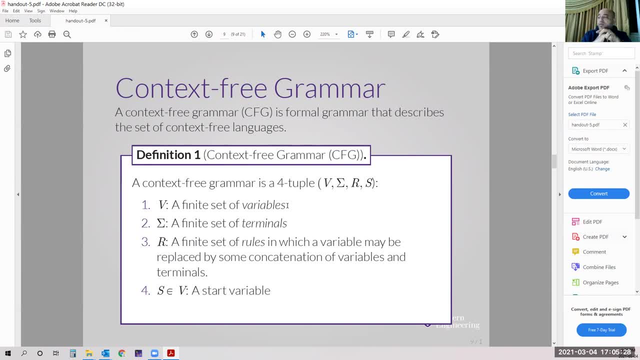 terminals, A finite set of rules are, or what we call it production rule, Which are variable, may be replaced with some concatenation of variables and terminals, The terminals, which is, if you remember, when we said let's L has a string as as belonged. 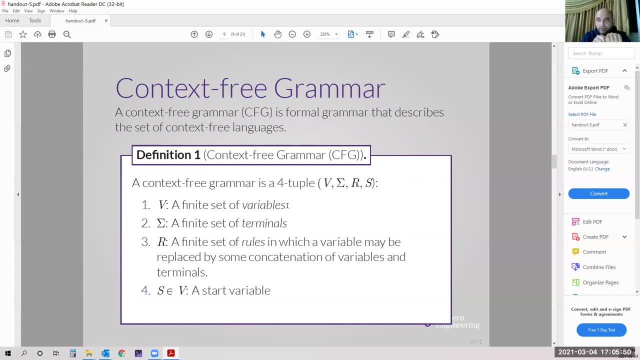 to 01.. So the terminal are 01.. The terminal are 01 as. which is the string, It's the variable, And we have some production rule how to change as to a string and as should belong to the variable. And we said V is a start variable. 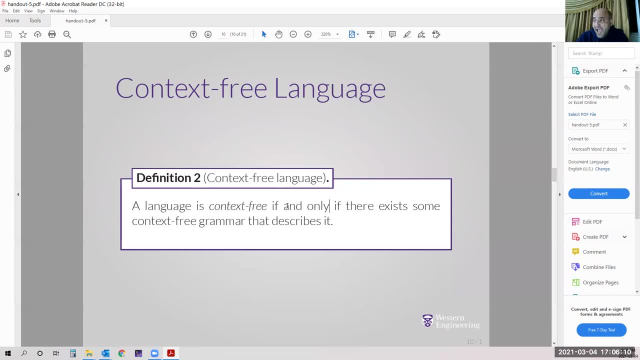 We will see now how A language is context free if, and only if, there is exist some context free grammar that describe it. We have a context free grammar And we have non context free grammar, And we'll use the pumping lima again to prove that this language is not context free grammar. 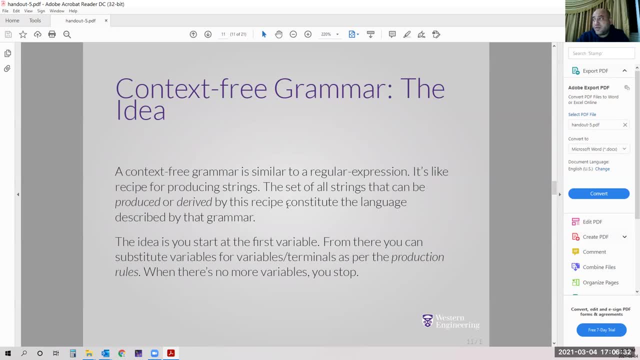 Context free grammar. The idea of context free grammar is similar to a regular expression. It's like receive of for producing strings, Which is some first steps that we have to follow, or some steps that we have to follow to change that grammar, Either. 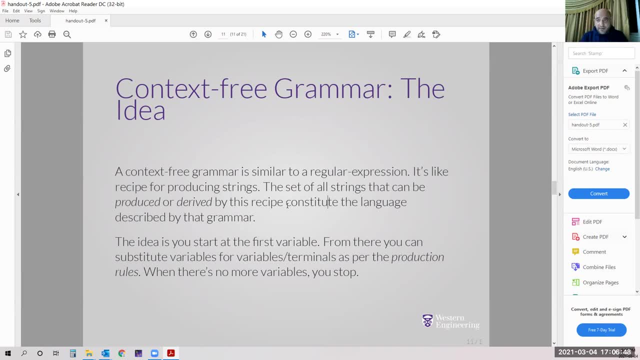 I give you the language and ask you to produce a grammar that describe it as a context free, or I give you this is a context free grammar. Identify the language. Belong to that grammar. The set of all the string that can be produced or derived by this received constitute the. 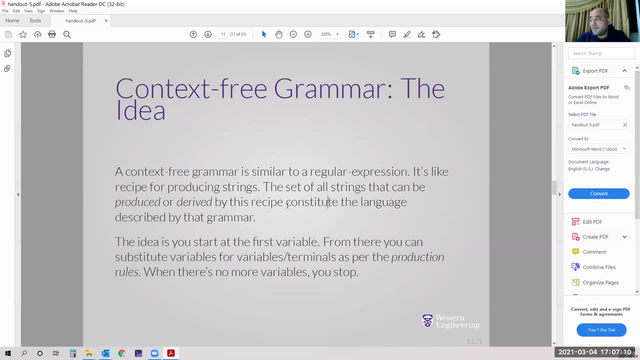 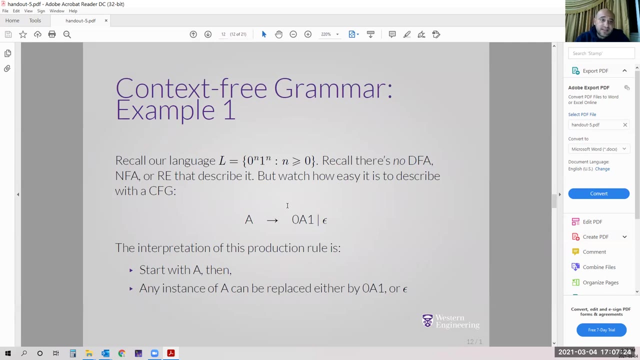 language described by that grammar. The idea is, you start the first variable. from there You can substitute variables As well as pair production rules. when there is no more variables, you stop. You remember what a friend example, First example that we use with pumping lima, that we prove that zero to the power and one. 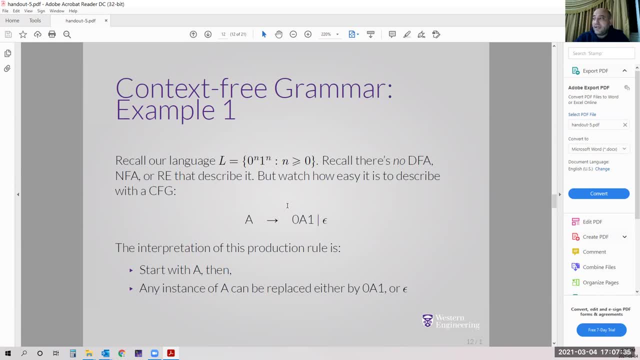 to the power and where, and is greater or equal to zero. It is not regular expression, right, But watch how easy it is to describe With a context: free gram. We have a variable, a. A could be replaced with 01, a or epsilon. 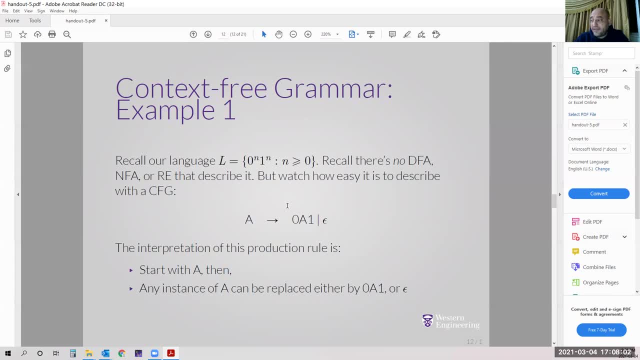 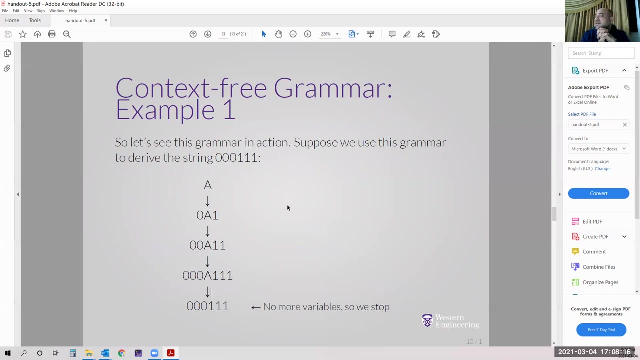 The interpretation of this production rule is start with a, than any instance of a can be replaced either By 01 a or an episode. Let's see, Suppose we use this grammar to derive the string if we wanted to arrive to 00100111.. 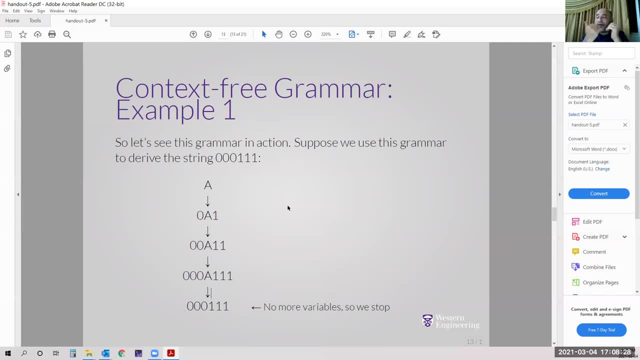 We'll start with a And we replace a with the first rule. We choose the first rule: 01 a. It will be replaced with 01 a. Then we again Choose to replace a with 01 a, which is the first production rule. 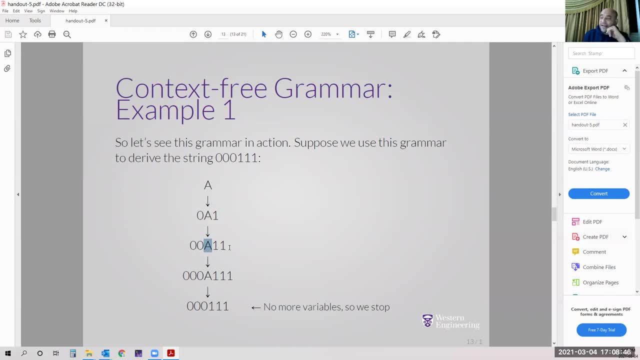 It will be 00 a 11.. Then we decide again to replace it with a 0 a 1 and the front before we have 0011.. Then we decide to replace a with an epsilon, So we'll have 000111.. 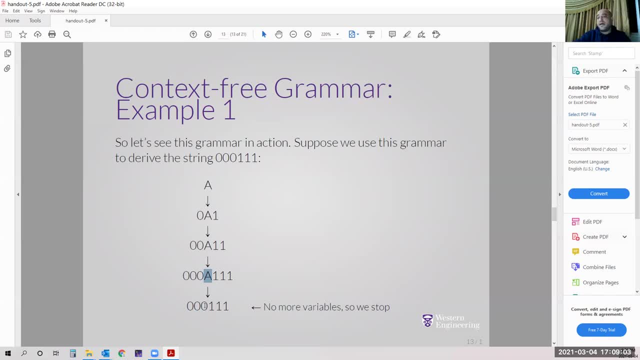 And there is no more variable to be replaced. We stop at this point. Clear to hear Questions Asked by voice. Don't send Chat messages. Sorry, sir, I just have a bit of an unrelated question. I got my final exam schedule and I noticed that there's an exam for this course on that exam schedule. 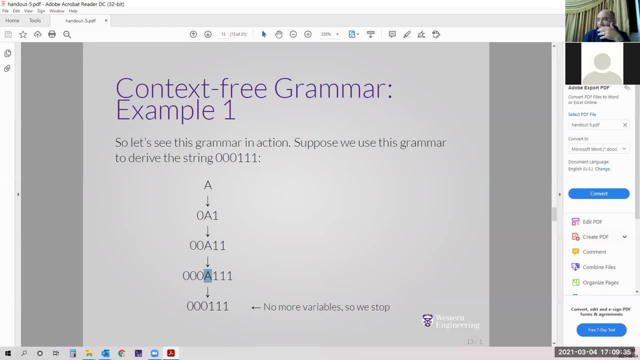 So I just wanted to confirm with you that we don't have a final. We don't have a final. I will email the secretary. I think it's a mistake by The undergraduate secretary or coordinator. I'll send her email telling her there is no final exam for this course. 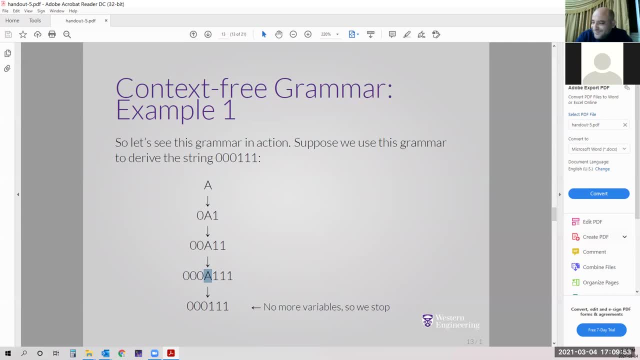 So they will remove it, No worries. Perfect. Thank you so much, sir. You're welcome Guys. So for context, free. like the whole point of the variable is to like maintain, like that memory, I guess, portion of the language. 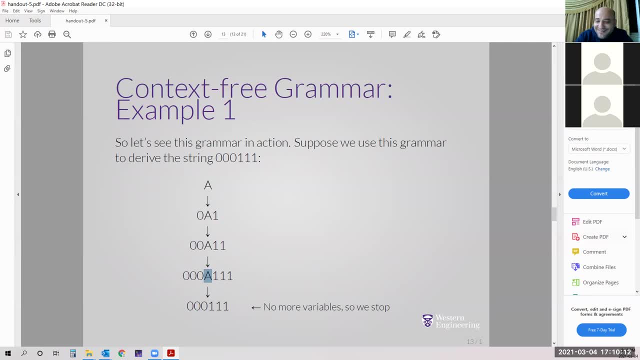 Don't jump to the to hand out Six or seven. Okay, Okay, Yeah, guys, you will see all these computational model We don't use memory yet right, With Turing machine will start to use the memory. Here we have a grammar. 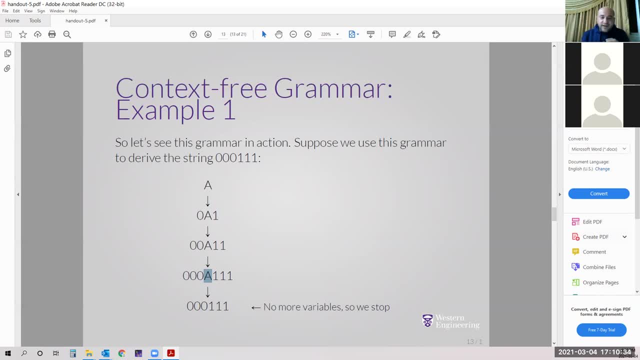 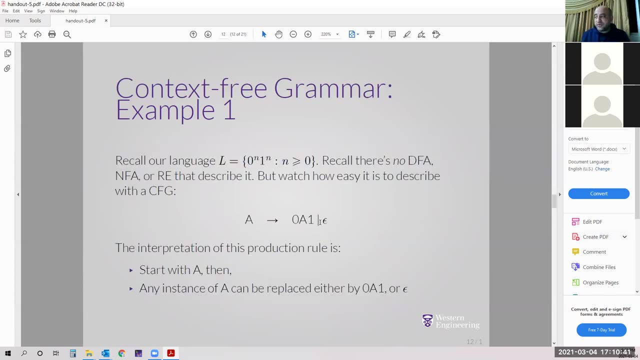 We just do a parse it And either with each variable, we replace it with one of the production rule. Here, for example. for this example, we have two production Rules. Either I replace the variable A. This is the starting variable. 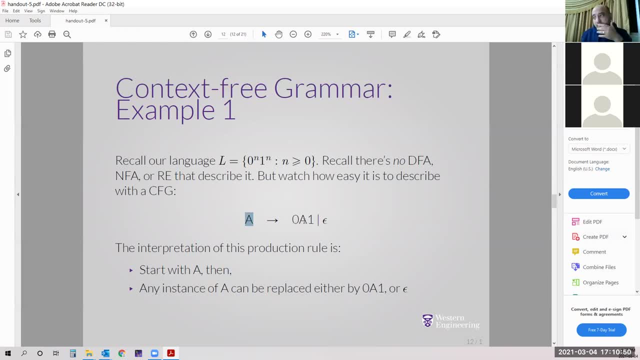 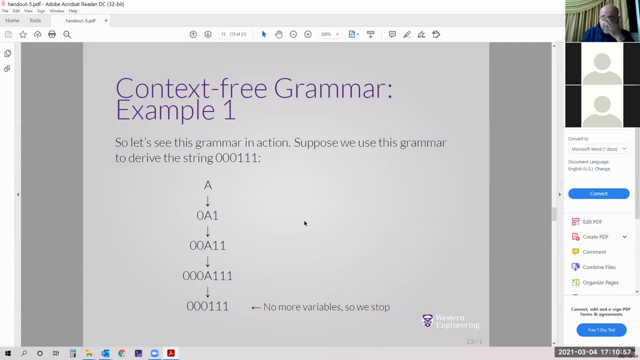 I either I replaced with zero a one or with Epsilon. Okay, But I'll ask a question. I will ask a question. Who can tell me If I give you this example and ask you, give me the language That is accepted by this grammar? 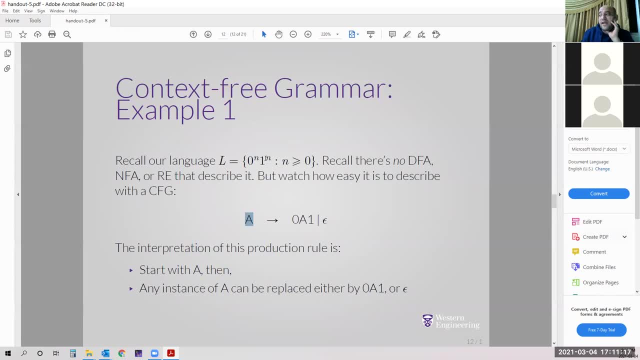 You will write: I'll equal zero to the power and one to the power, and where I'm greater or equal to zero, Or if I give you this language and ask you to build or construct a context of free grammar, you will have to think: 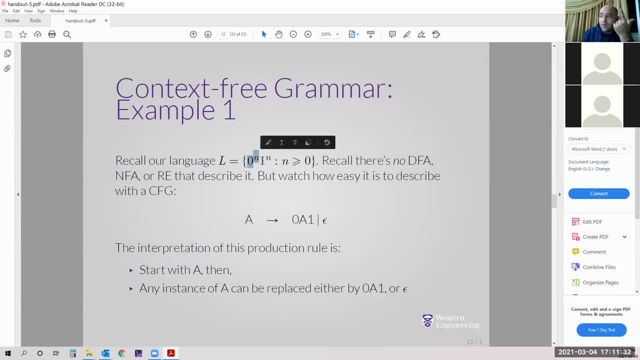 Okay, I share. I should have that equal number of zeros and equal number of ones. So I have at that time, Okay, And if this is the case, then I can replace it with a zero, A one at Which mean: 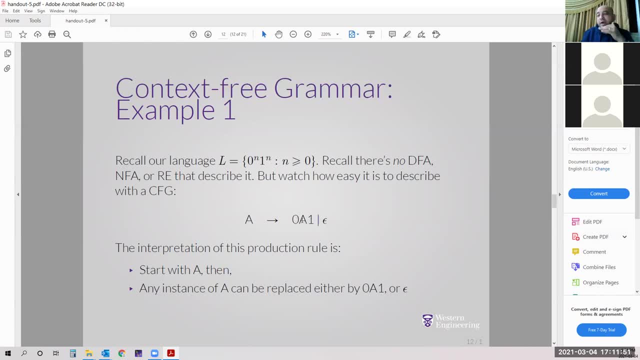 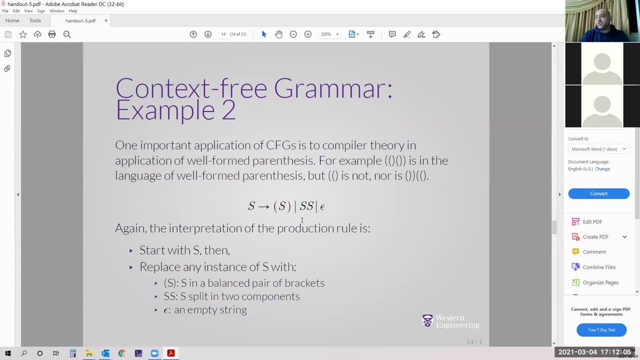 At each zero I have a one to match it. Then I can replace it with another zero, a one or an Epsilon. So I'm giving you a different scenario that you can see. the question We'll see in our examples. Okay, let's take example number two. 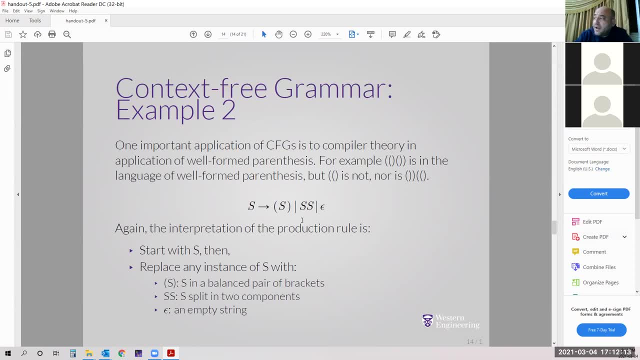 One important application of CFGs is to compiler theory in application of a Wilford parenthesis. So we should have a balanced parenthesis. With each left parenthesis we have the matched right parenthesis. so we don't have the left parenthesis as more we have or assume that we have more parenthesis from the left side. 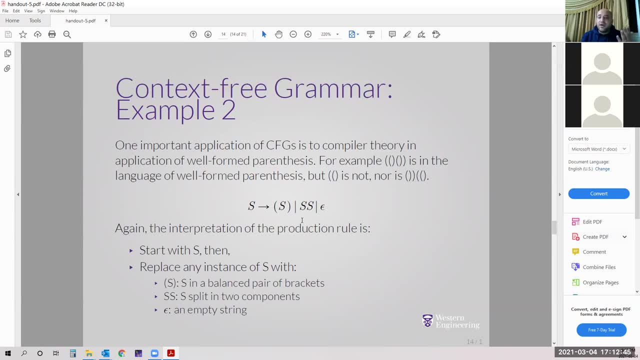 more than the right parenthesis. no, it's not accepted. or I have more right parenthesis than the left parenthesis. also, this is a case that is not accepted. It should be a balanced case, So it's either. I should think about the scenarios. 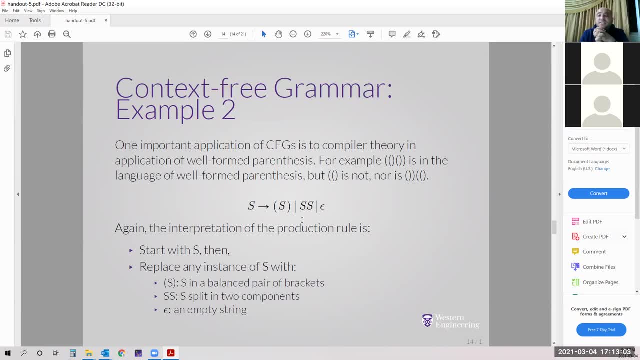 I ask you to put the context-free grammar that described this language, which consists of balanced parenthesis, How we can do that? We have one of two cases: either I have parenthesis inside each other, Or I can have left, right, left, followed by left right. 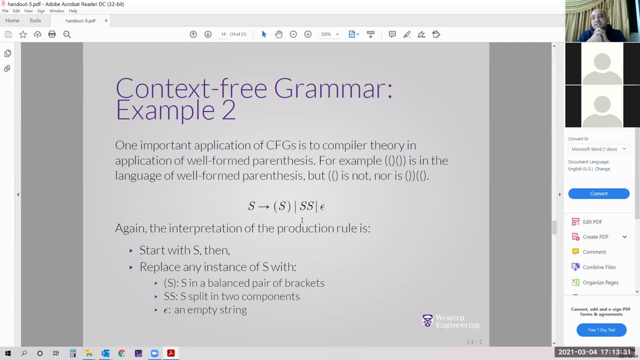 How can I produce this kind of context-free grammar? The first one: if I have parenthesis inside each other, I write parenthesis as parenthesis, But if I have left right, left right, then I can put it as as as beside each other. to 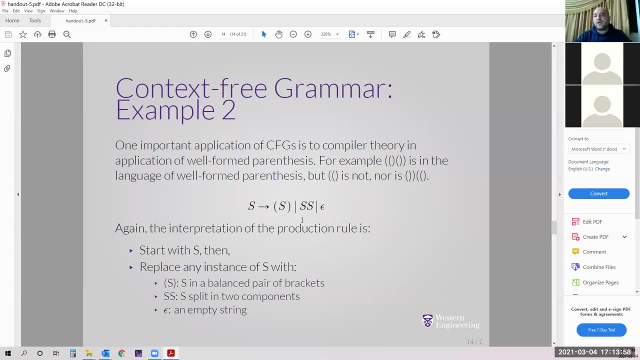 have it So to simulate all scenarios of the parenthesis or epsilon. again, the interpretation of the production rule Is to start with us, then replace any instance or instance of us with left as right parenthesis, in a balanced pair of brackets or in a split into two component. 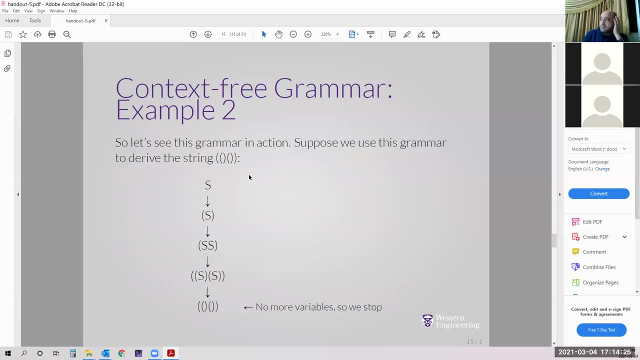 and epsilon, which is the empty string. So assume that we ask you to derive this in the class, not? it's more generic example. So Assume that we'll have this scenario, that we need to do it, then we have to start with. 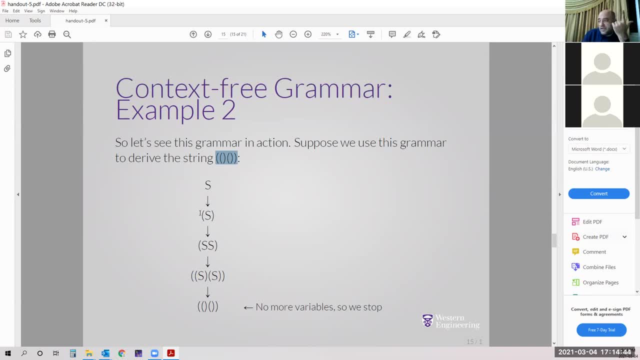 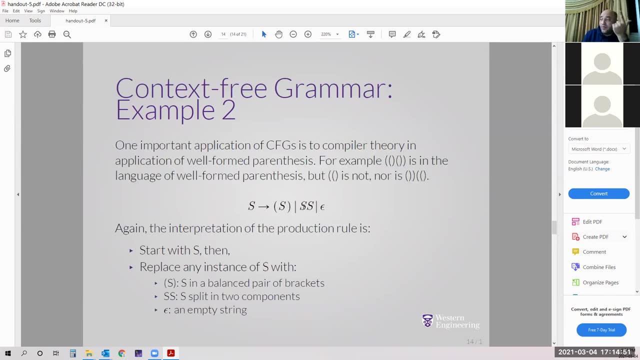 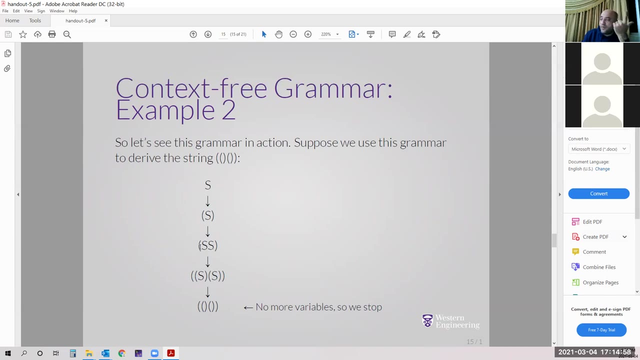 us, Then we'll make us left as right, then left as as right. We replace us here with the second production rule, which is as us, Then we'll make we change those one with first, each of them with first production rule. 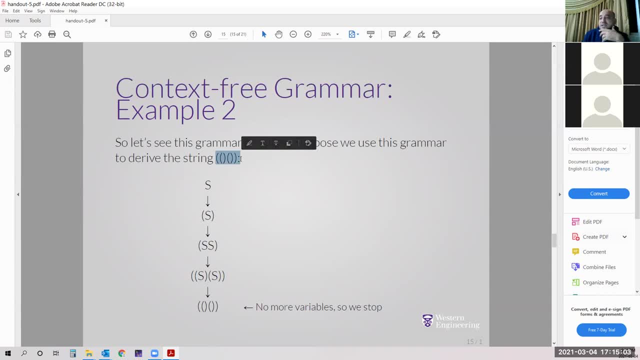 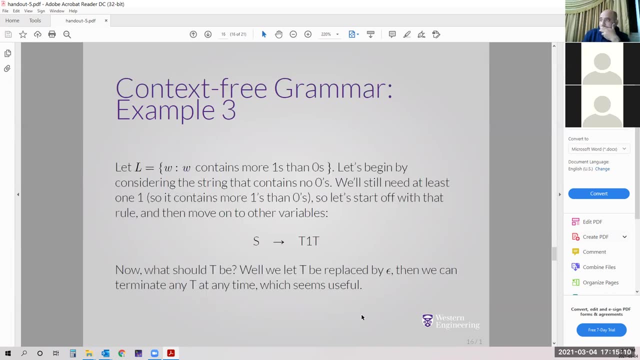 Then we replace them with epsilon and we have the scenario that we ask to derive. So no more that variable, no more variables. though we stop Just to just give me a sec, guys, And working from home, Okay, Okay, Okay. 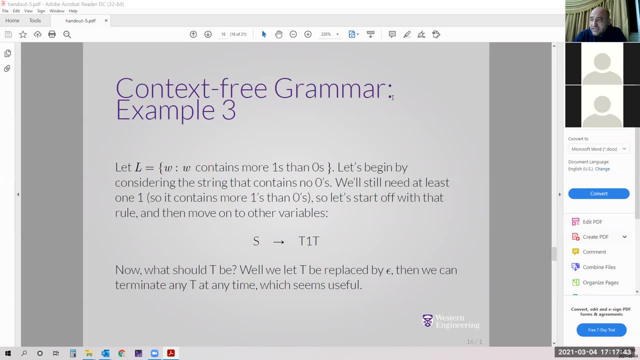 Okay, Now let's have another example. Let L equal W. W contains more zeros than ones. How we can simulate this one? No spider, I'm not scared River. Okay, Let's continue. She think that she saw a spider. 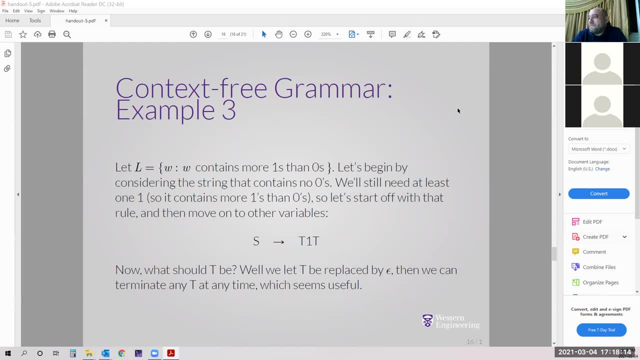 There is no spider, but she think that. Okay, So That our string W that it has to- contains more ones than zeros. Let's begin considering. the string that contain no zeros will still need at least one, So it contain more ones than zeros. 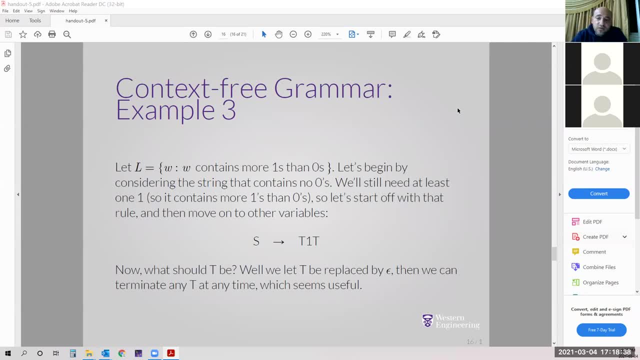 So let's start off that rule. So this is the first rule. I have to think about it. So I'll make s equal T, one team. You can use V equal s- one s, But no that I would not accept any variable in a small letter or lower case. 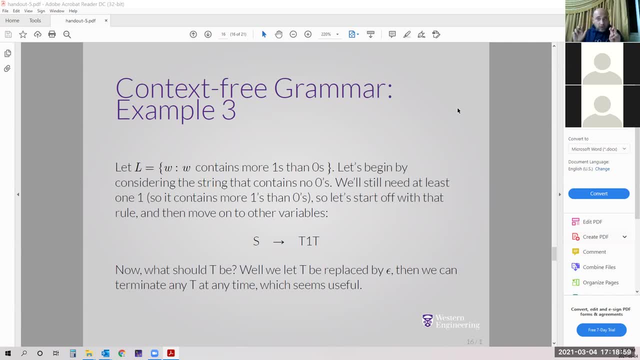 All variable. It's a rule. All variables should be written in an upper case. I put it in the class, Not for you. I put it in the class, Not for you. Okay, I wrote that in the class, not for you. 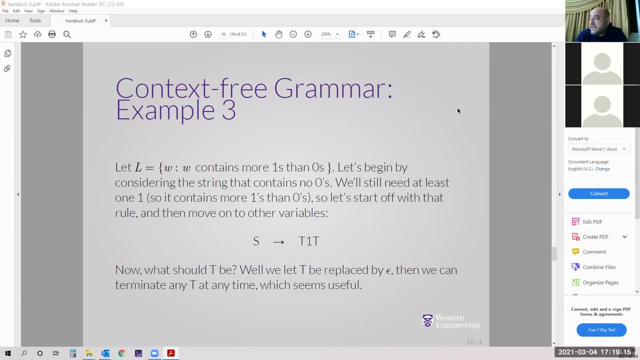 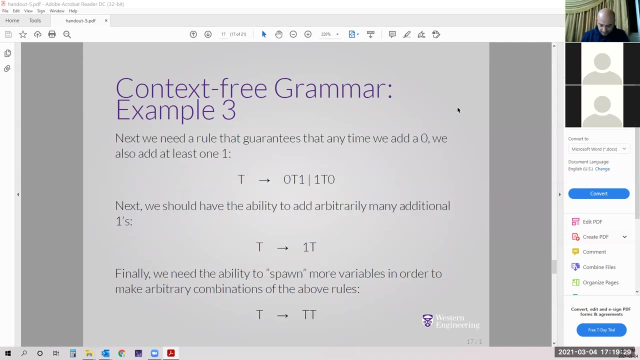 Now, what should T be? Will let T to be replaced by epsilon. then we can terminate any T at any time, which is seem useful. It is useful, but it's not cover all scenarios. What about zeros? So next, we need a rule that guarantees that at any time we add a zero, we also add at least one. 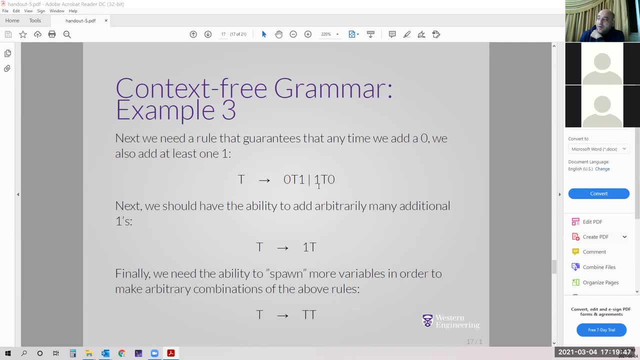 So T, it could be either zero, T1 or one T0.. So when we add any zero, there is a one, and at the beginning we have a one added. Also, we need a rule that guarantees that at any time we add a zero, we also add at least one. 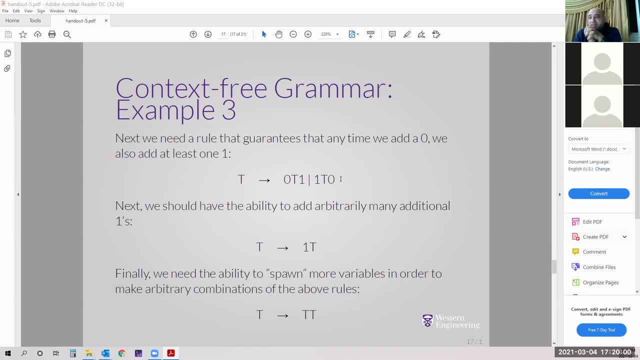 So what about only ones? to add more ones than zeros? So we should consider another production rule that contains one only. So we said T will produce one T. Finally, we need the ability to spawn more variables in order to make arbitrary combination of these above rules. 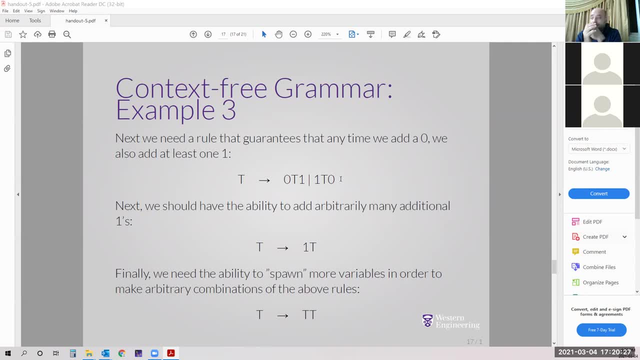 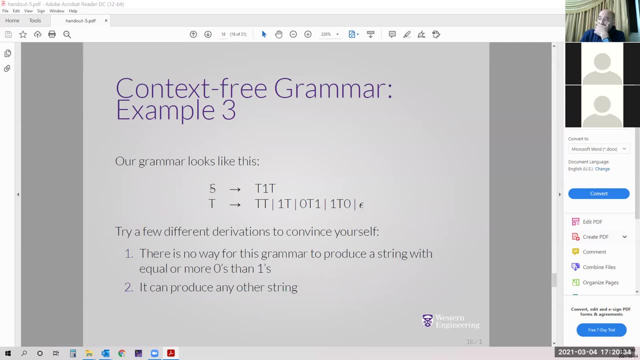 Then we can say: T can produce T2.. T is for two T, which could be either this one or this one or the first rule. So S will give T1, T and T could be either TT or 1T or zero T1, or one T0 or epsilon. 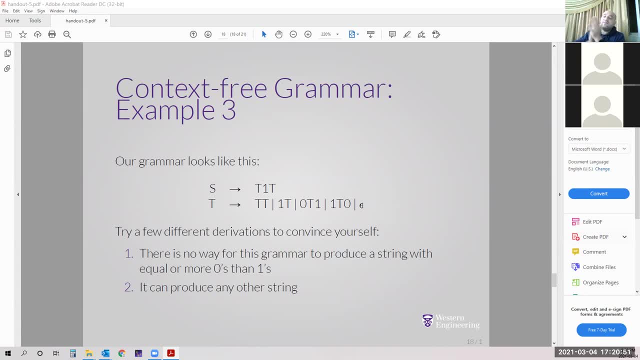 So here we take all scenarios that will give me that the number of zeros is less than the number of ones. Try a few different derivations to convince yourself. There is no way for this grammar to produce a string with equal or more zeros than ones. 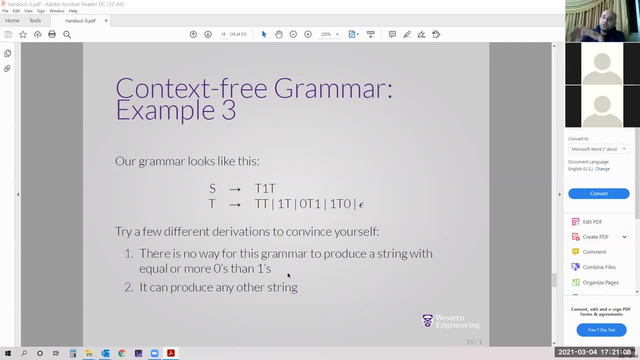 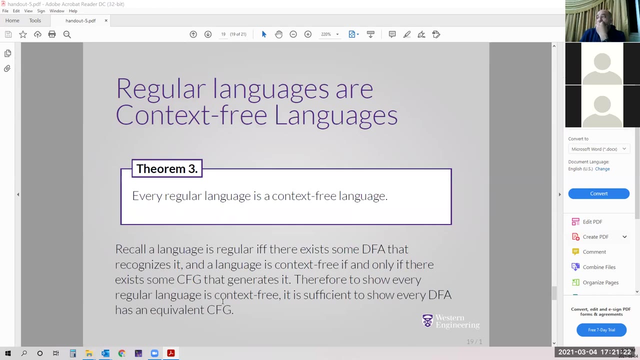 Here we make sure that the number of ones at least more than the zeros. even with one instance It can't produce any other string. Regular languages are context-free languages. So you'll ask me, we talk from the beginning of the class about non-regular languages. 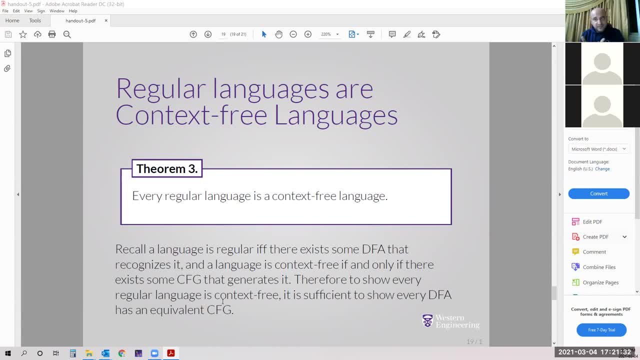 What about regular languages? It is a part or a subset of context-free languages. So there is a theory that every regular language is a context-free language. Recall: a language is a regular if there exists some difference between them. There is a DFA that recognizes it, and the language is context-free if, and only if, there exists some context-free grammar that generates it. 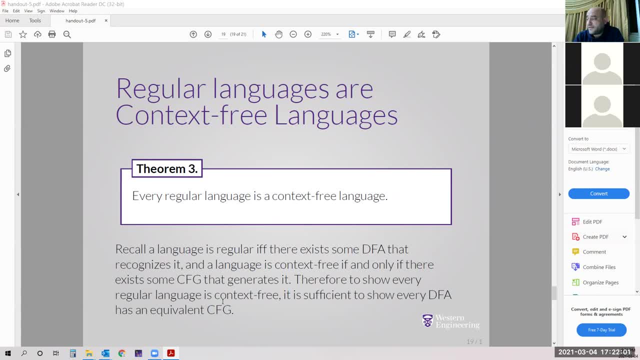 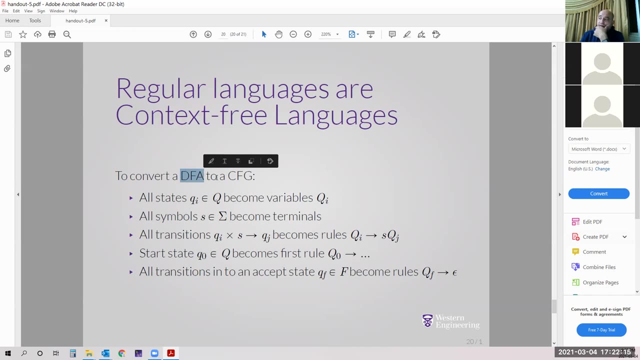 Therefore, to show every regular language is context-free, it is sufficient to show every DFA has an equivalent CFG. So I'll give you some example about the DFA has equivalent CFG. To convert the DFA, a deterministic finite automata, to a CFG: 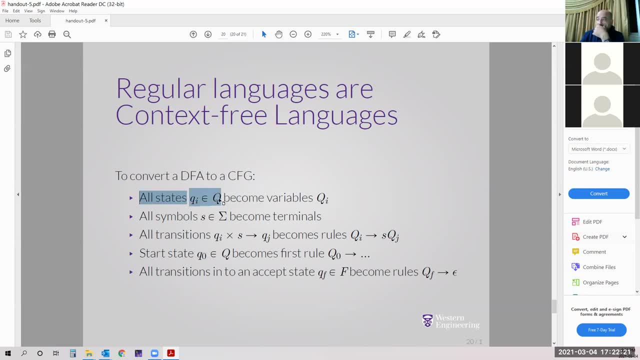 we said All state qi belong to q, become variables. we call it qi. All symbols s in the strings before belong to sigma, which is the alphabet, become terminals. All transition rho or delta, small delta qi times s will give me a qj. a new state becomes rules, qi to sqj. 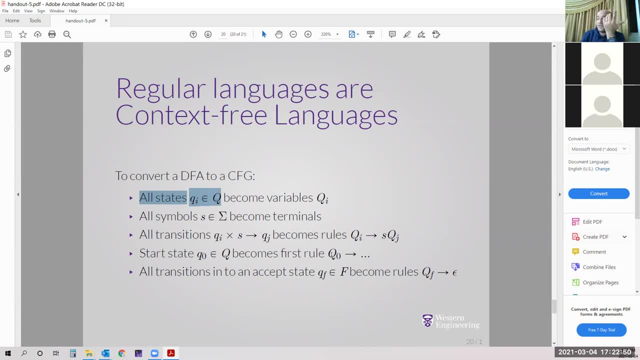 Start state q0 will become 2q. Start state q0 will become 2q. First rule is q0.. All transition into an accepted state qf belong to f become rules, And then one of the qf will take us to the epsilon to stop that conversion. 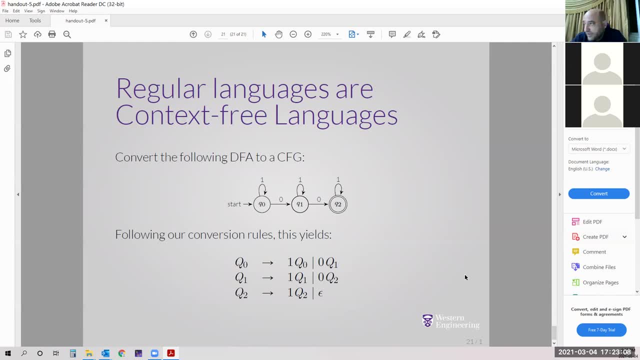 For example, if you receive a question, convert the following DFA to a CFG: The DFA that we have, q0, if we receive one, will stay at q0.. If we receive zero, we'll go to q1.. Then, if we receive a one, we'll stay at q1. 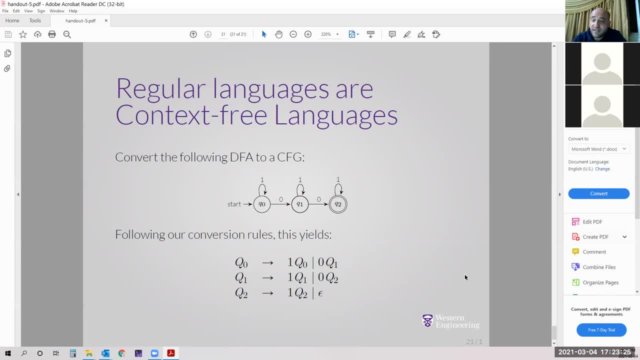 If we receive a zero, we'll go to q2, which is an accepted state. Then if we receive a one, it will be an accepted state at the end. So, following our conversion rules, this yields to q0 will give me 1q0 or 0q1, right. 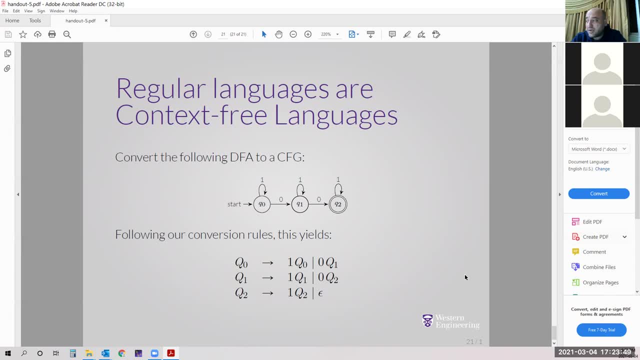 And the q1 will give me 1q1 or 0q2.. q2 will give me 1q2.. And if I receive a zero or whatever, it will take me to epsilon. These are the conversion rules, Great guys. 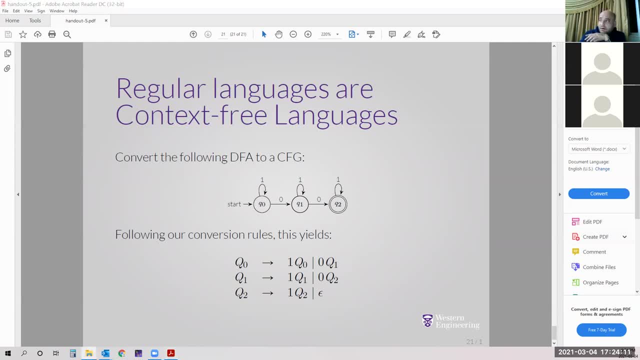 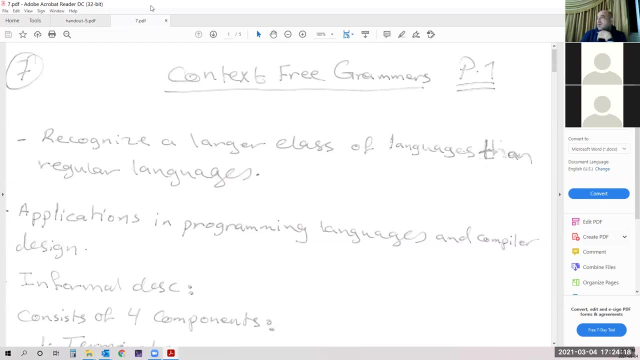 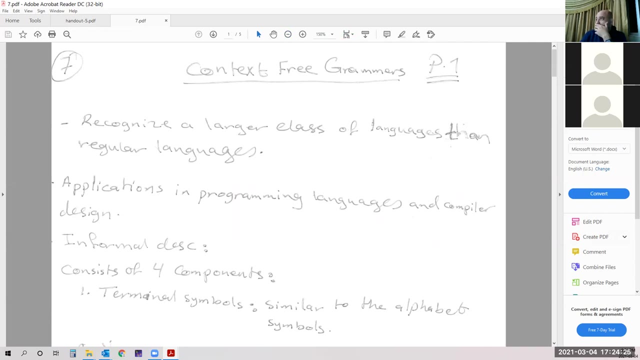 So now we will move to our class notes For this class. Can you see it? Can you see the class notes? Yes, sir, Okay, So again, we will repeat the handout in a simpler way And assume that I'm writing this in the board. 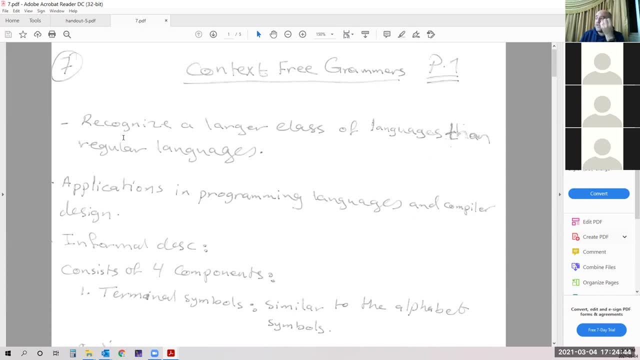 So we are recognizing a larger Class of languages than regular languages. We go wider, As I said in the beginning: Application and programming languages and compiler design. We use these things in Building the compilers Under the programming languages Informal description. 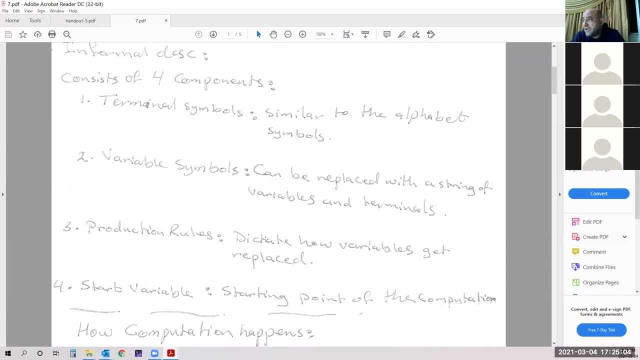 We have the formal description taken in the handout. So here how we will solve the questions. This is the most important thing for you guys: to get marks. So We have a terminal symbol Which is similar to the alphabet: Simple zero or one ABC or whatever we have in that language. 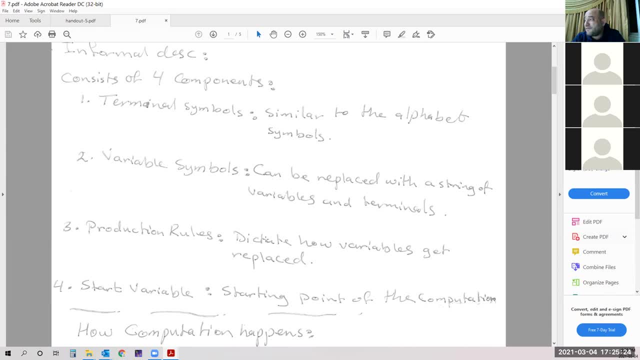 Variable symbol can be replaced with a string of variables and terminals. Both Production rules Dictate how variables get replaced. We'll give a rule how we can replace the variable, Then the start variable, Which is the starting point of the computation. 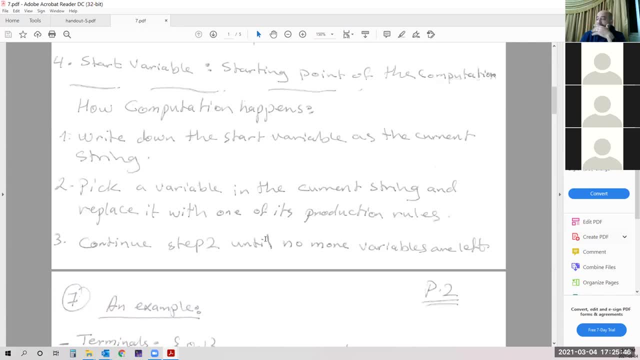 How computation happens. We have three steps. Write down the start variable as the current strength. Pick a variable in the current strength and replace it with one of its production rules. Continuous tip to until no more variables are left. These are the three steps that you need to solve any question. 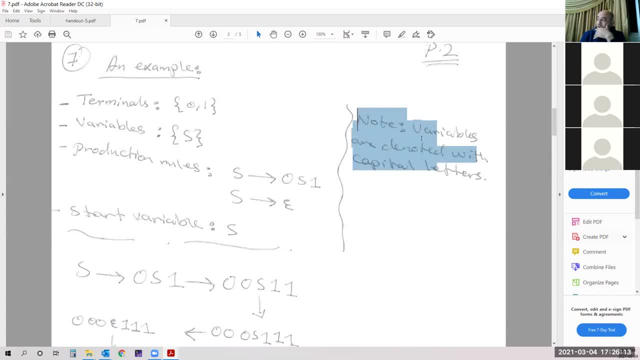 Here I put, for you know what variables are. Variables are denoted with capital letters. only Don't put it in the exam in small letters. Okay, Terminals. This is an example we have, which is the first example that we have. 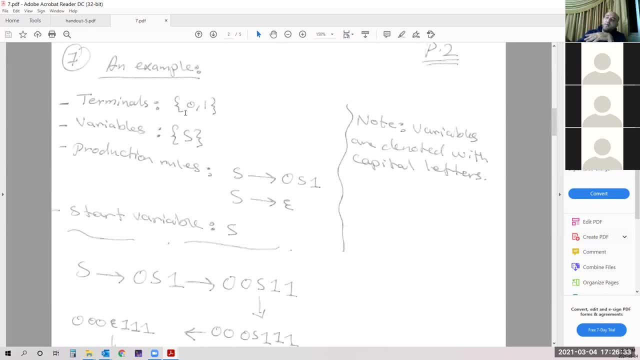 But here I make it vice versa. If you receive it, If we have the following CFG, What is the language that is describe it? Okay, So we have this production rule. The variables are as As could be zero, As one or could be an epsilon. 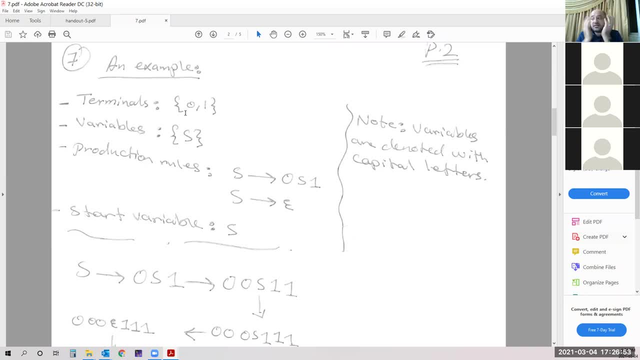 Start variable is as: so. Okay, I'll start with us. I replaced it with first production rule. I am not going to epsilon from the beginning, So it will be zero as one. Then I replaced this as with zero As one again. 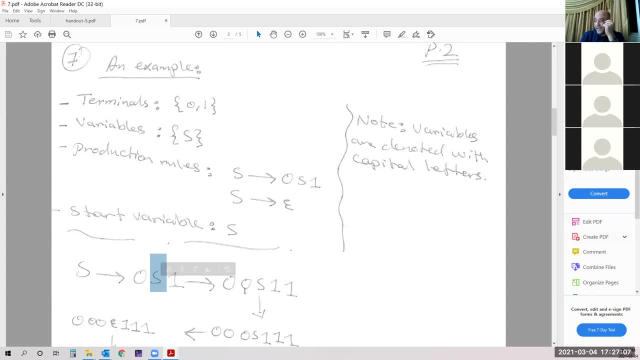 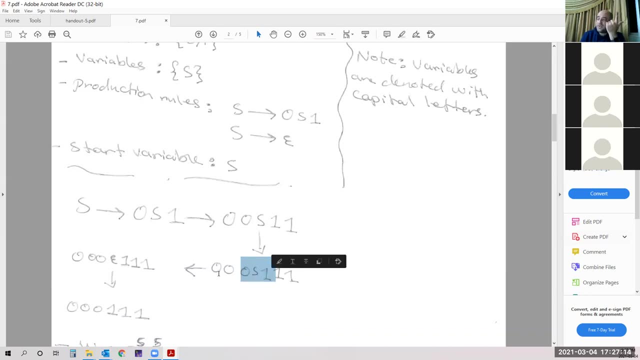 So we'll have zero, zero as one one, Then we'll go to the next one, And then we'll go to the next one, Then we'll go to zero, zero again. We replace it with zero as one. So we'll have three zeros as three ones. 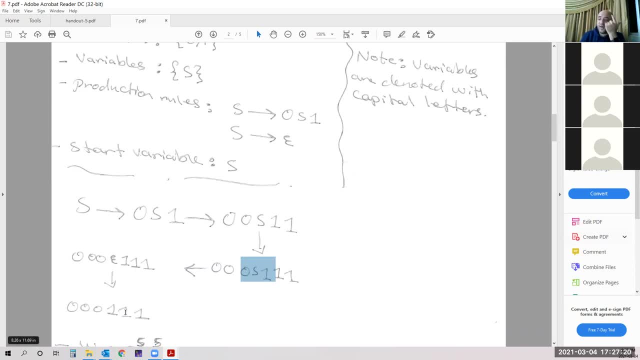 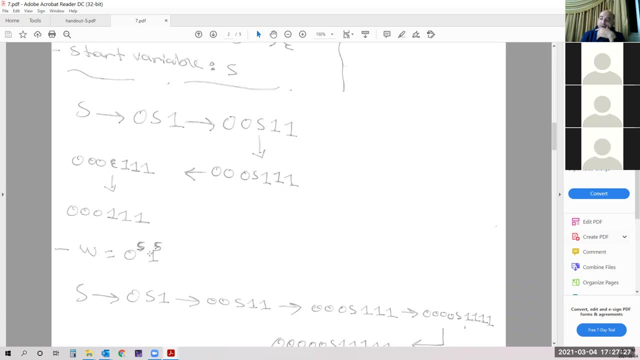 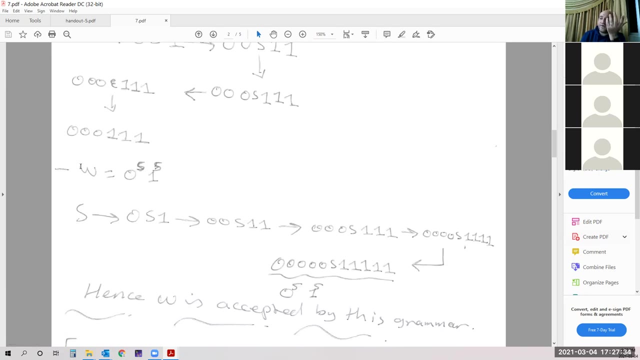 Then we change it with epsilon, So we'll have zero, zero, zero, one, one, one. Assume that I give you W zero, five, Zero to the power of five, one to the power of five. Okay, So I'll ask you, is this: 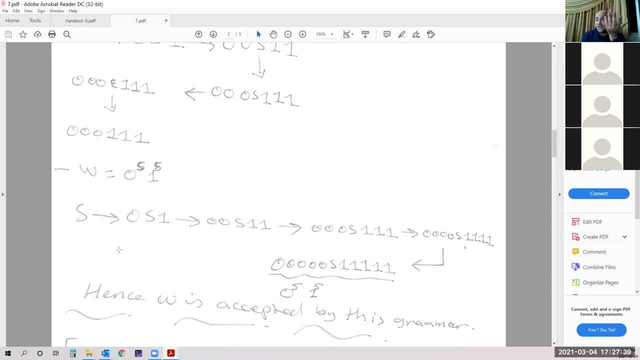 String accepted by The CFG. You, I will check As equal: zero as one, Then zero zero as one one, Then the three zeros three ones, Then four zeros as four ones, Then Five zeros as five ones. 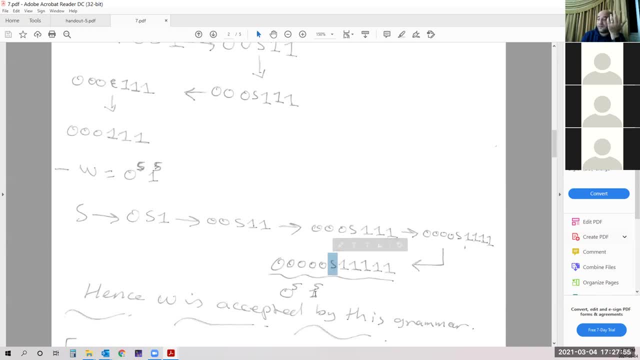 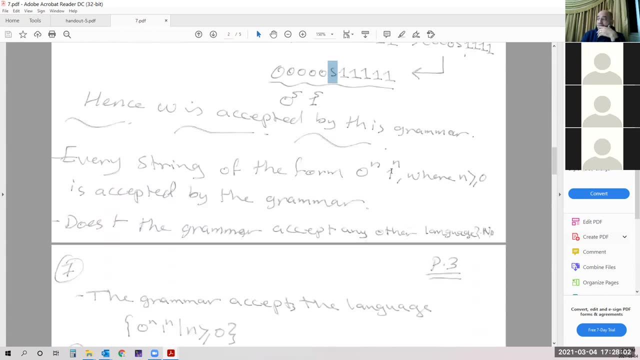 Then we'll change this one with the epsilon, So we have zero to the power of five, one to the power of five. Hence W is accepted by that. This is a grammar, Every string of the form zero to the power And one to the power. 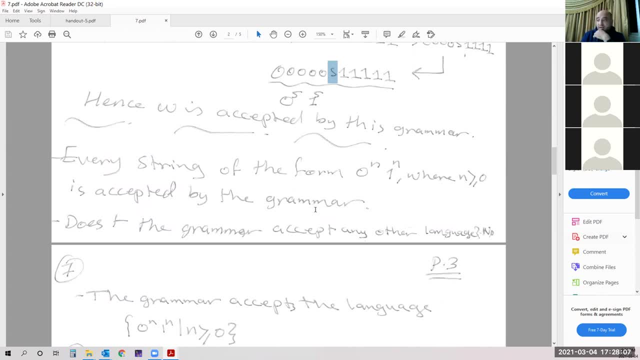 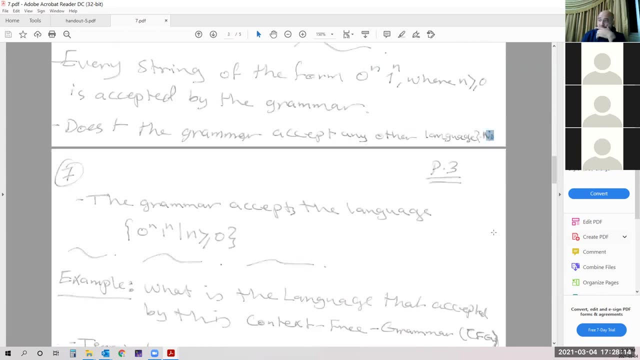 And where, and is a greater than zero Is accepted by this grammar. Does the grammar accept Any other language? The answer is no, So this grammar will accept the language zero to the power And one to the power And is a greater or equal zero. 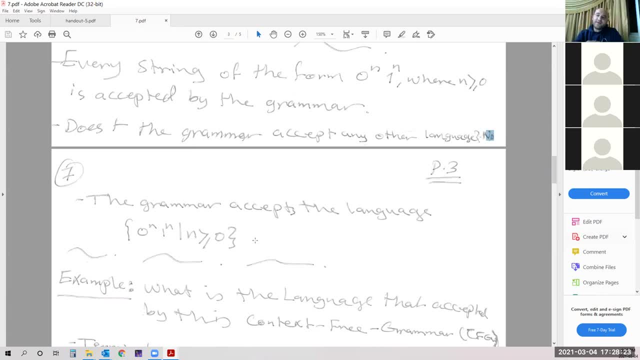 So here's the first example that we took in the handout, But I do it In the other way. If we have this, What is the language that is accepting, Accepted by this grammar? So the question can come in two way. 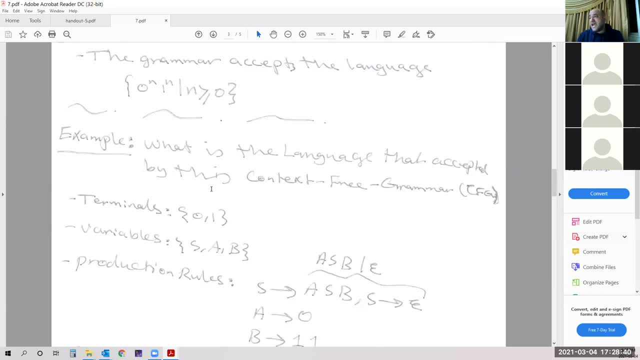 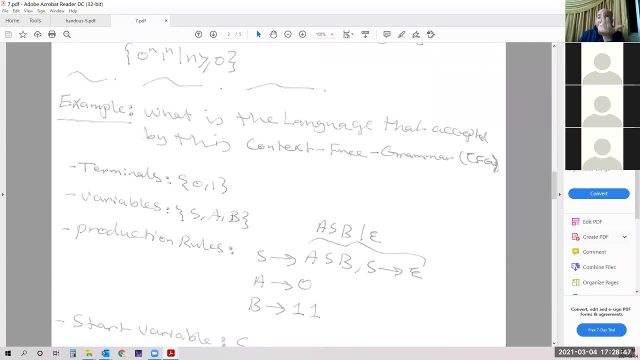 Okay, What is the language Accepted by this context? free grammar, If we have terminals, are zeros and ones. The variable S, a and B Production rules As S, Which is we'll send Amy As B Or S To epsilon. 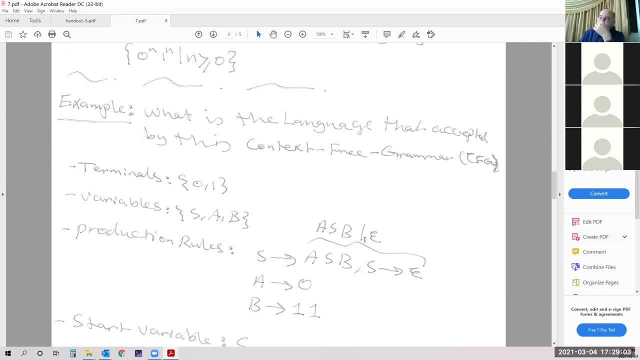 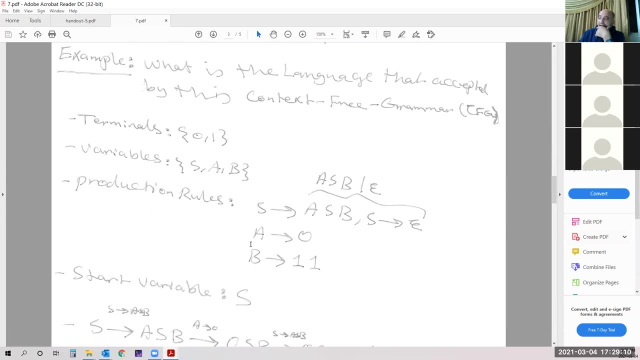 How we do not this. We write it And we put the column to replace or or the comma. So this is the formal way that we describe The grammar. A will take me to a zero, Then B will take me to a one one. 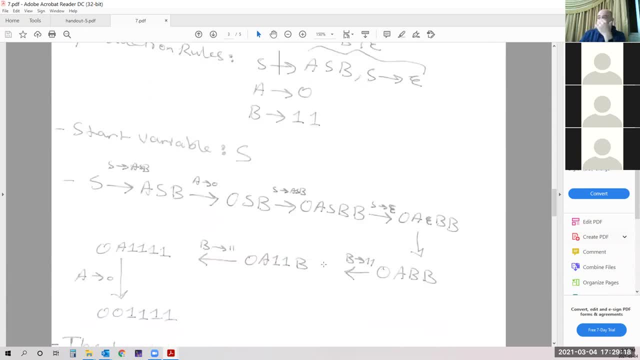 Start variable is us. Now we are zero choices To find the language. So, as here, I put in the top what we replace it with, To understand what we are talking about. As we replace it with ISB, Then we replace it with zero. 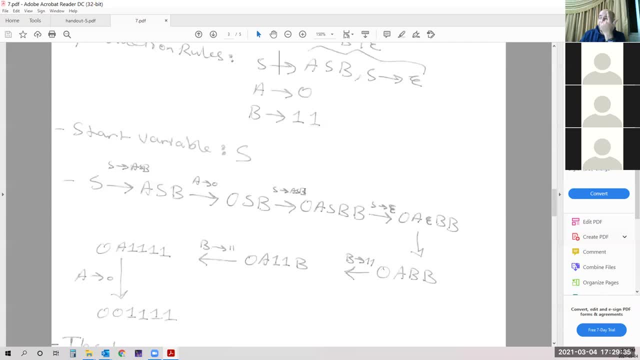 It's become zero SB. Then we replace it again with first production rule, which is As me. So it's become zero A SBB. Then we replace us with epsilon, So it's become zero A epsilon BB. Then it's become zero ABB. 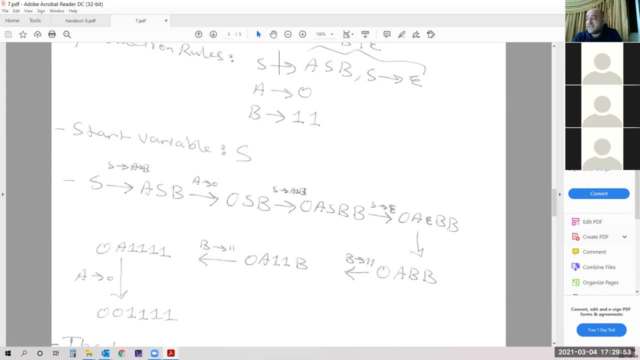 We replace the first B with one one, Then we replace the second B with another one one, Then we replace the air with zero. So we have zero, zero, one, one, one one. So I think it's a clear that the number of zeros is half number of one. 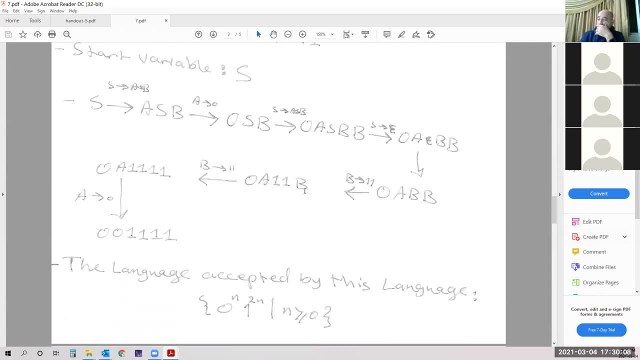 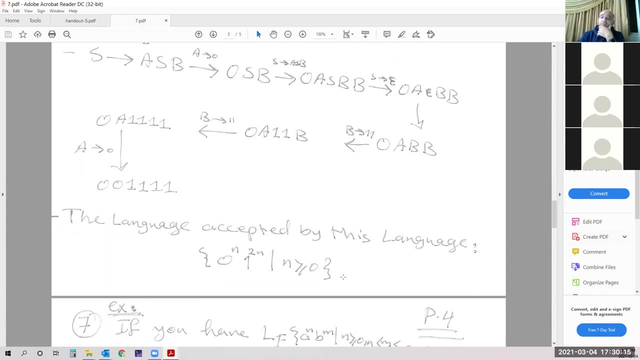 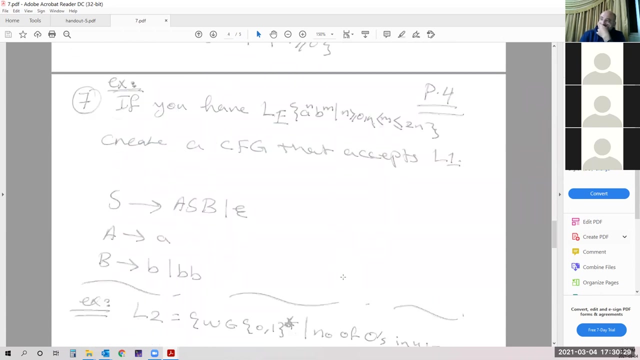 Okay, So how we describe this language? The language accepted by this language is zero to the power And one to the power. two Where an is greater or equal to zero. Clear Questions. Okay, Let's take another example, If I give you the language. 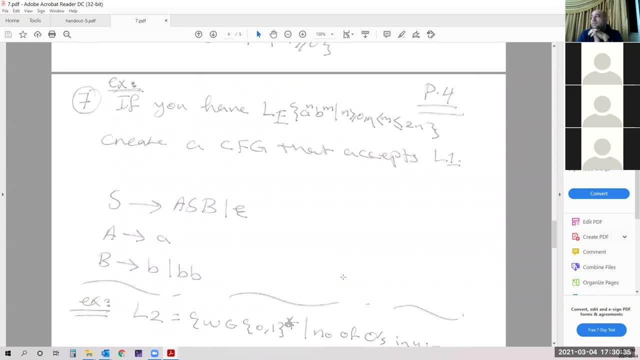 One Equal A to the power and B to the power, Where an Is a greater or equal to zero And an Is a great, is less or equal to M, And Where M is less than two, and which mean That: 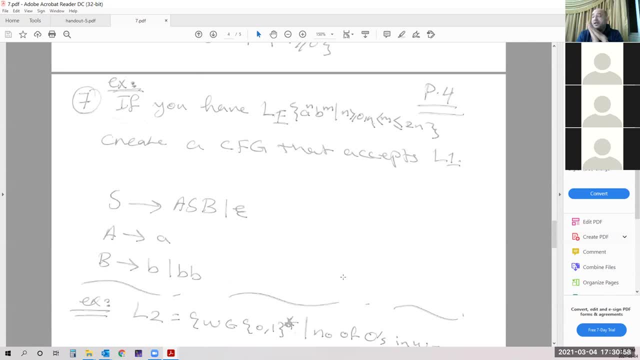 The number of zeros is less than the number of Of A's is less than the number of bees. As maximum, The number of bees should be double number of Ace. But it could be less How we can do this one. So we make it a SB and epsilon. 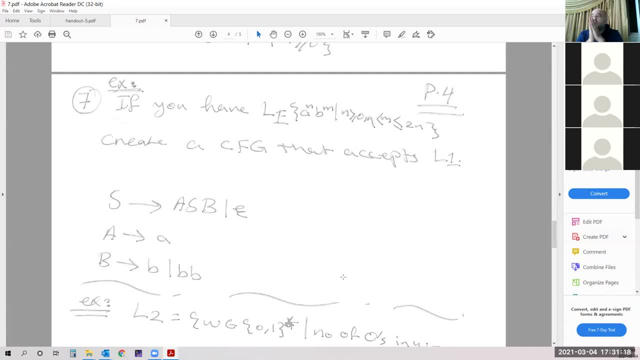 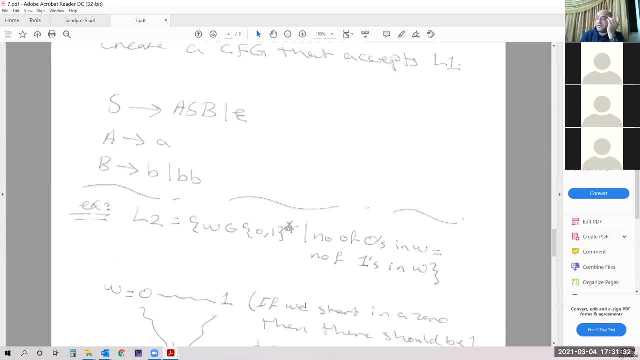 It could be a and B If it is equal. If it is equal to the same number As minimum, So it will be B, Or if it will be as maximum BB, then we'll change it to BB. So we take all scenarios. 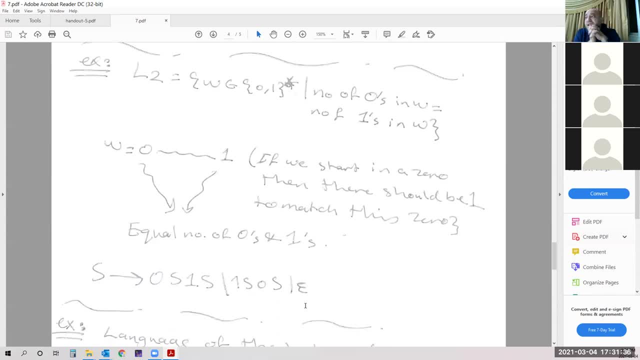 Now, if I ask you to do The second example, if we have L2.. That consists of a string W, W belong to zero, one star. Number of zeros in W equal to number of ones in W. So Here is the same example of zero to the one, zero to the power, and and one to the power. 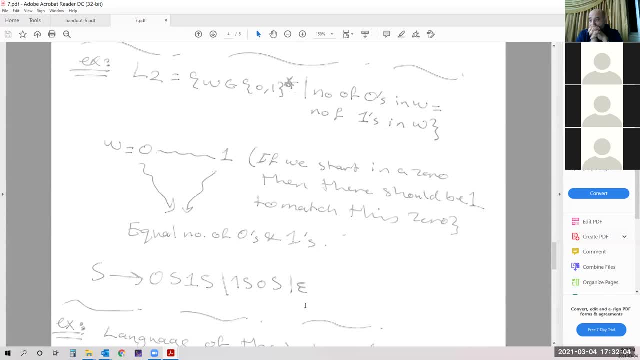 So Equal number of zeros. So, as could be Here what we see With each zero, we should have match number of one, equal number of zeros and one. If we start with a zero, then there is should be one somewhere. 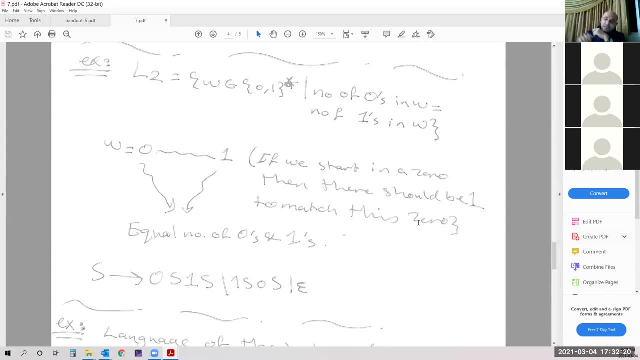 To match the zero, like the same example of parenthesis. So we put that The production rule as zero, as one, as One as zero, As if we start with zero, Or we start the string with one, Then epsilon, Then we can change any one of them. 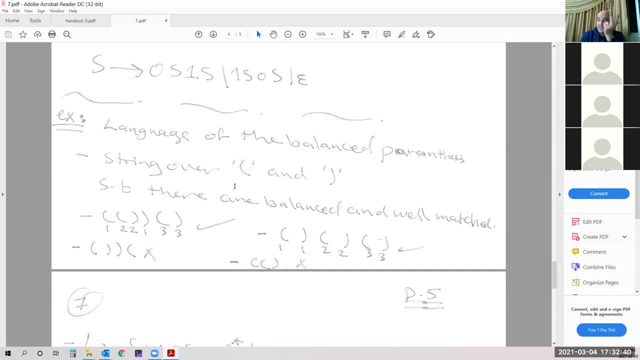 Okay, The language of balanced parenthesis, The same one. We take it a string over Left and right parenthesis, such there are balanced and will match. So this one is accepted. This case is accepted with a separate one or split one. This one is not accepted and this one is not accept. 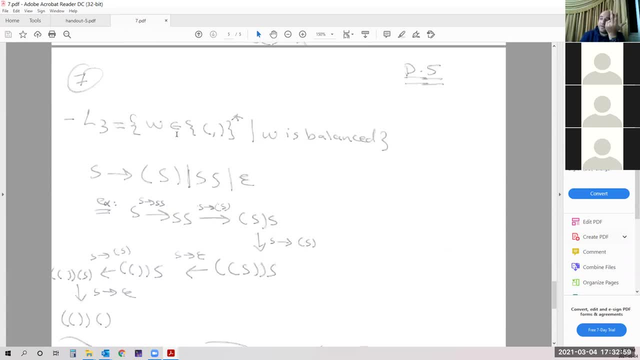 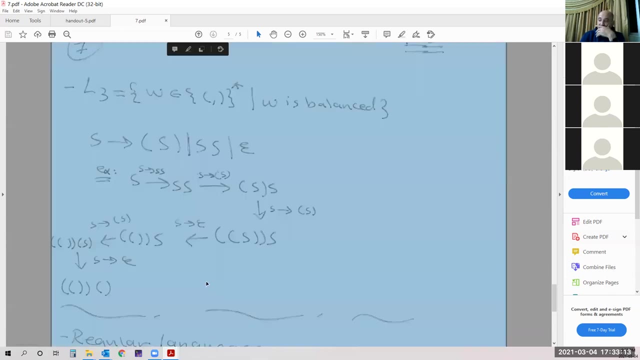 So here how we write it: All three W equal, Left and right, parenthesis star W is balanced As equal, Or as, as or epsilon. We took the same example And here how we move in between them And we have this example: 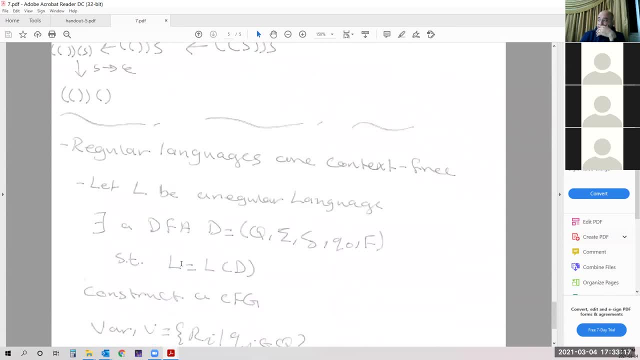 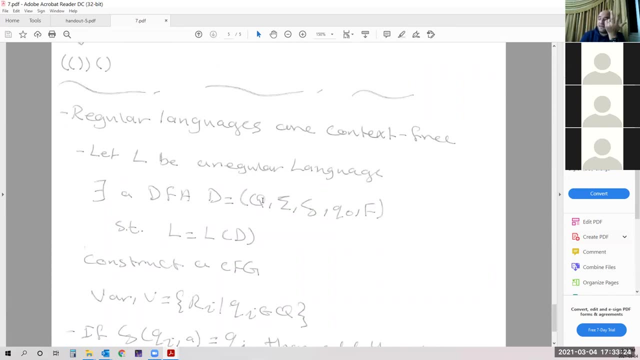 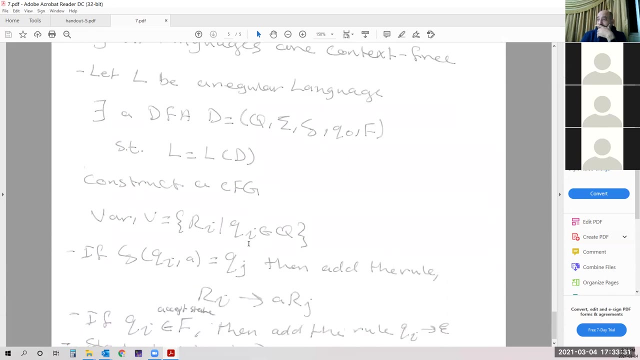 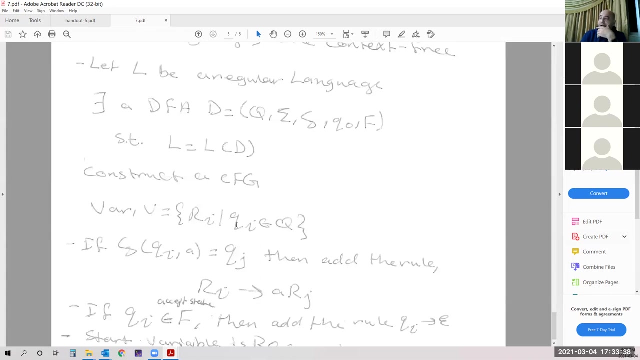 So regular languages are context free grammar. So let L be a regular language. Then there is a DFAD with these tuples such that L equal L of that DFA Construct a CFG. Then we write variable Or V, Which equal RI where QI belongs to Q. 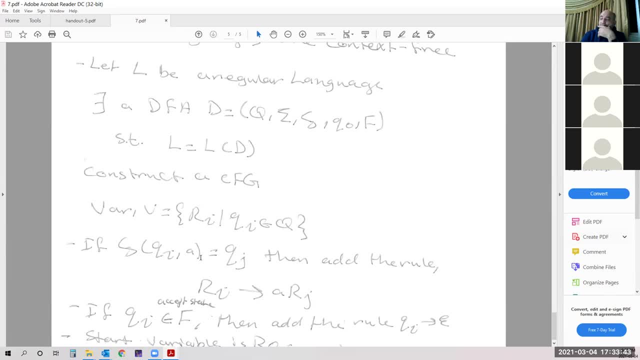 If Delta QI send me to A, Then it will go and I receive an A, Then I will go to QJ. Then add the rule RJ to ARJ. If QI belongs to F, Accept the state This mean. 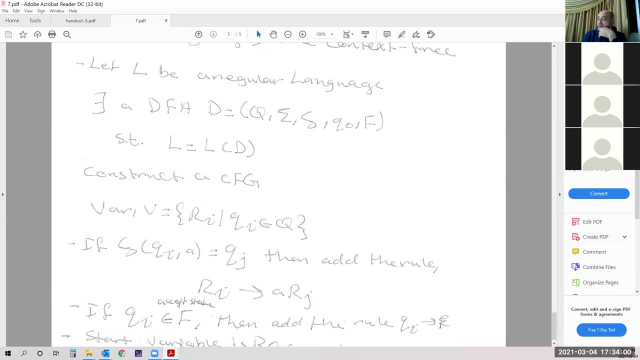 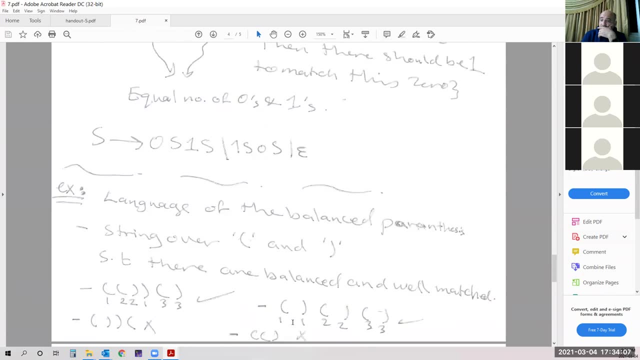 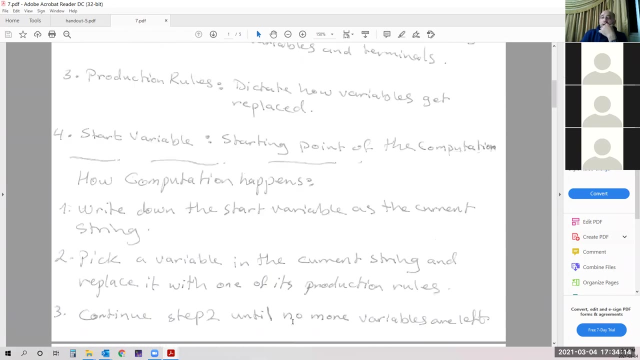 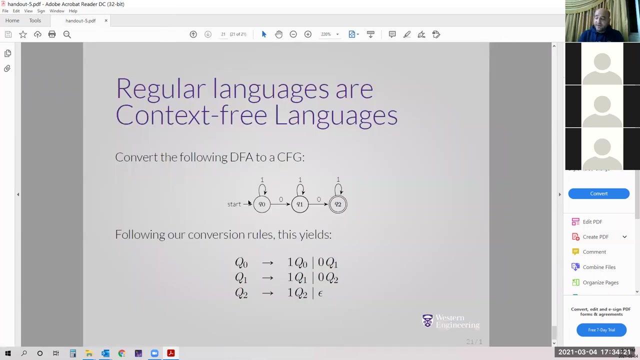 Then add the Rule where QI belong to Sigma, Start variable is R0.. So here We are done With The Hand out five And we talk about context free grammar And how we can convert a DFA to context free grammar. 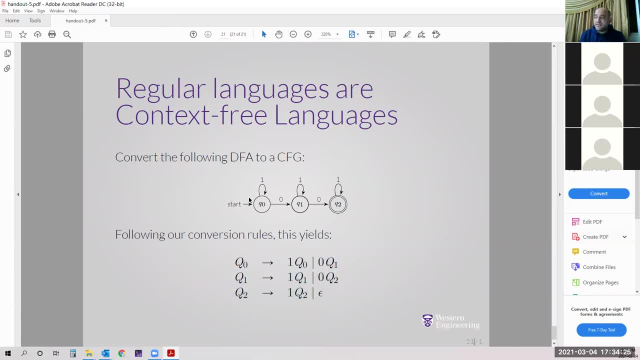 And these are the rules that I need, Based on this diagram And how those Could be Changed. And any Regular Language Is a context free language And non-regular language Also a context free language- Some Okay. 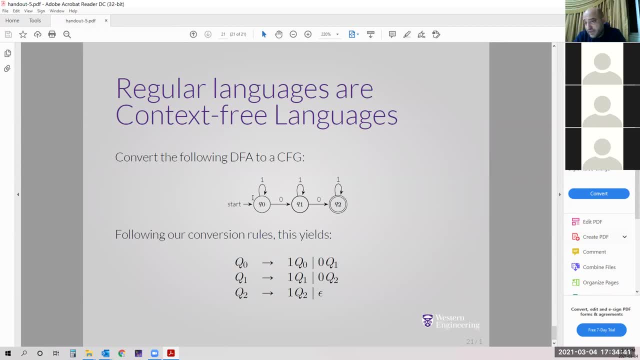 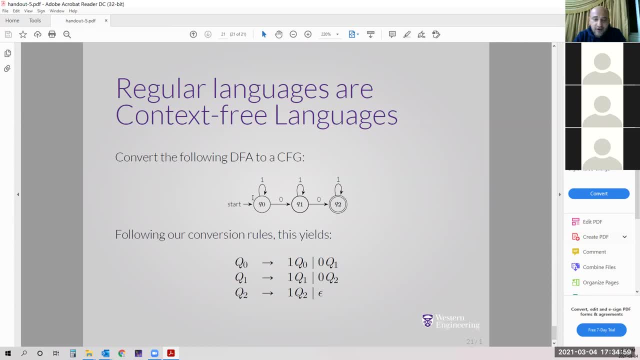 Okay, Okay, Okay, 10 minutes. Okay, Thank you, Okay, Thank you, Okay, Okay, 10 minutes. Okay, Rachel, Go ahead. So you have a 10 minute break, guys. See, after 10 minutes we will start with handouts. 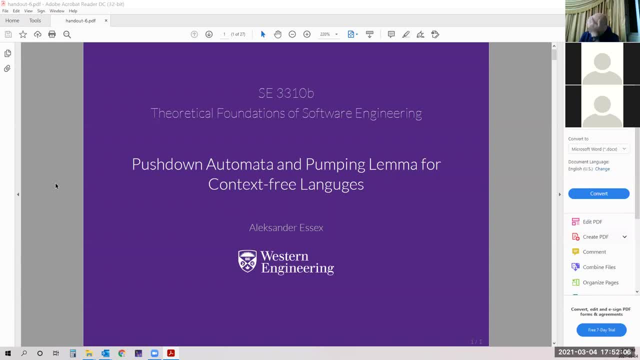 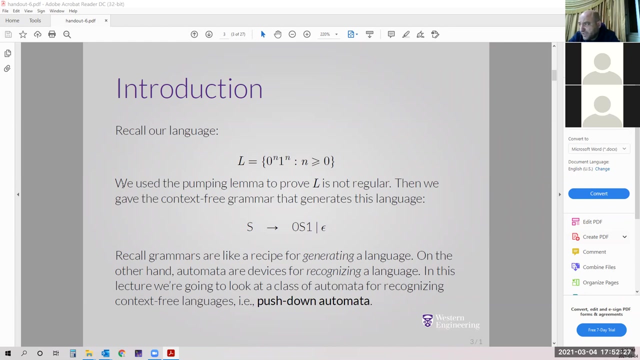 With Six. Okay Okay, We'll start with him. Score: Okay, Okay, Okay, Okay. Do recording. Okay Okay, We'll start with home out six grammar for context-free languages. Our standard example: the language that consists of zeros and ones, and they have. 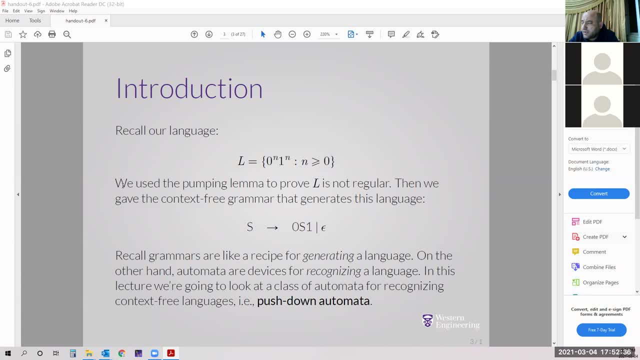 the same number of zeros and ones where n equal, greater or equal to zero. We use the pumping lemma to prove l is not regular. Then we gave the context-free grammar that generate this language, which is 0 as one. epsilon or epsilon Recalling grammar are like a receipt of generating a language. 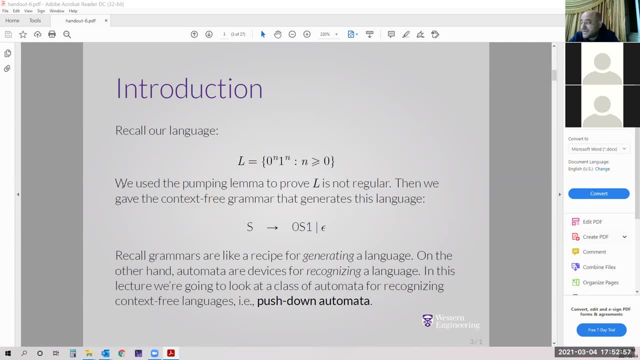 On the other hand, automata are devices for recognizing a language. In this lecture we're going to look at the class of automata for recognizing the context-free languages. push down automata And if you remember in the figure that at the table that we have in the 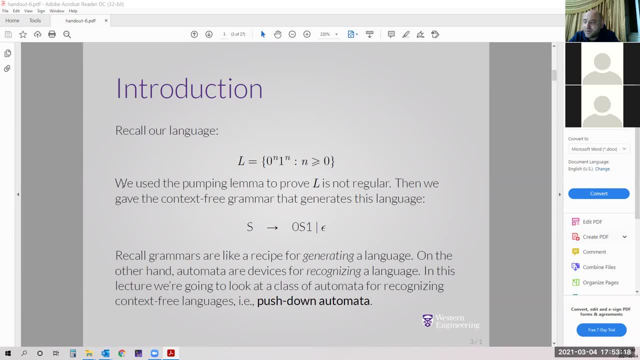 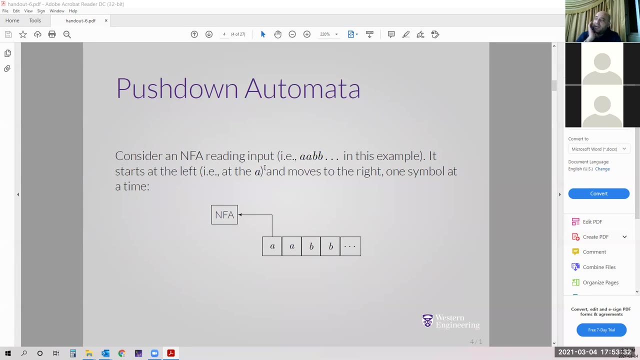 previous handout we said that the context-free grammar. if we talk about automata or automaton, we will talk about push down automata, which is a connected topic to what we were talking about in the previous handout. What is the push down automata? Consider an NFA. 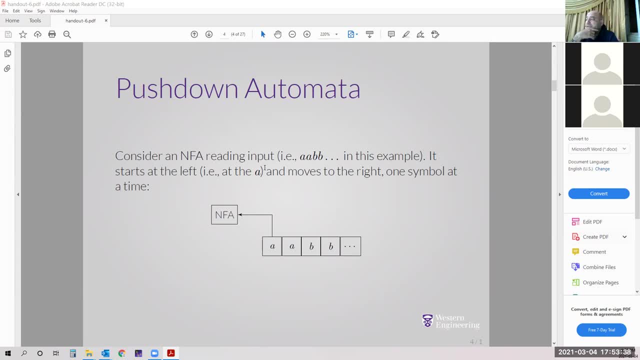 non-deterministic finite automata reading input AABB. In this example it starts at the left, at the A, and moves to the right, one symbol at a time. Assume that we have guys- I don't know if you remember the normal tape recording tape. 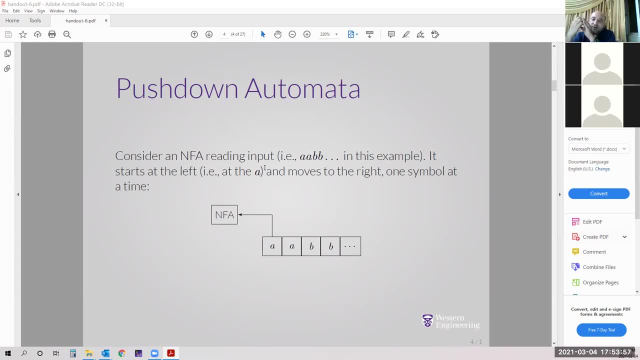 do you remember that? Assume that we have a recorder using the normal tape, that's two circles and it has just only forward. we don't have backward. If we have the backward, we'll talk about Turing machine, which is the next topic that we will cover. 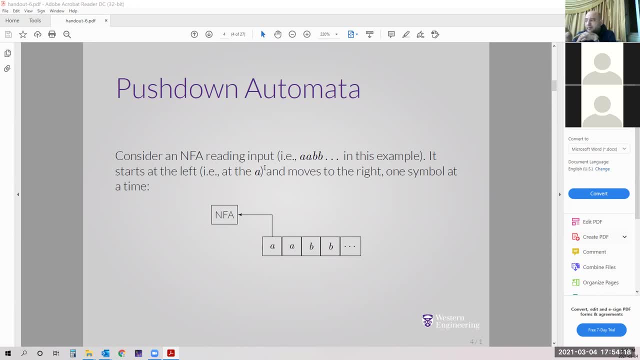 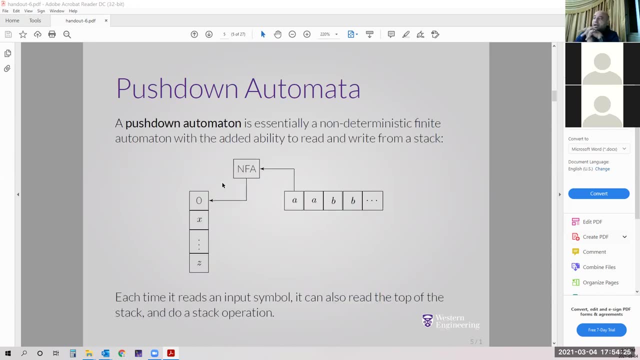 So here we'll push down automata: Push A, then we'll push another A, then B, then another B, et cetera. Okay, a push down automata is essentially a non-deterministic finite automata with added ability to read and write from a stack. 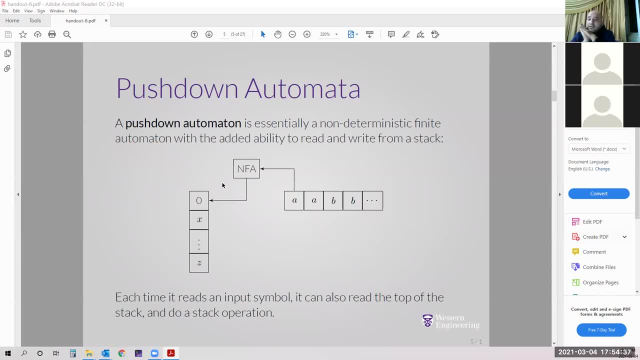 You know the principle of the stack. We will add symbols and once we pop a symbol, which will be the last symbol in the stack, each time it reads input symbol, it also reads the top of the stack and do stack operation. What do we mean by stack operation? 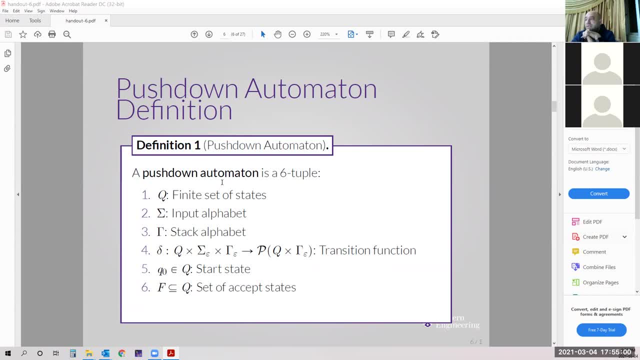 We'll see now. Push down automaton definition. It is a six-tubel which consists of Q, sigma, Rau or tau, some of them call it- which is delta Q node, and F- Q is the number of the stack. 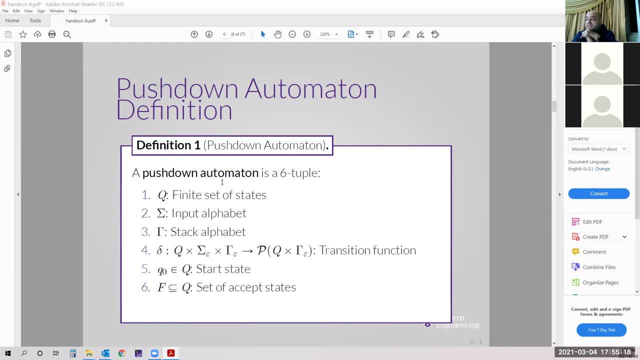 It is the number of the stack. Q is a finite set of states. Alpha is input alphabet, Then tau is a stack alphabet. Delta is Q by sigma epsilon or tau. epsilon will give me a new transition function, P, which will be the Q times the Rau epsilon. 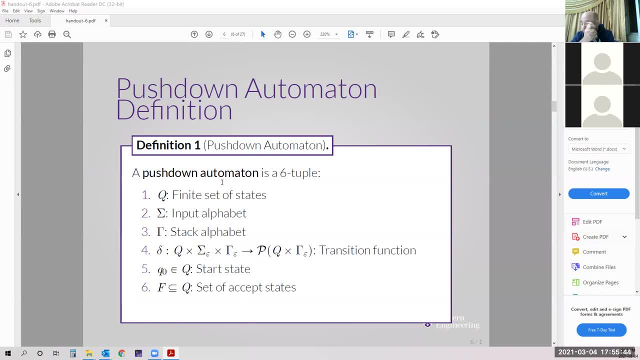 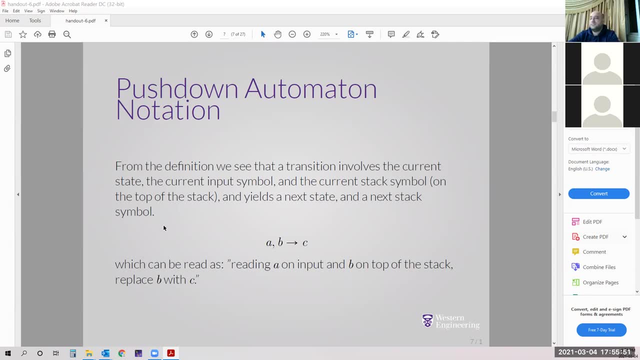 Q naught is a start state and F is the accept state. If you want to see ourringe with a start state, if the referenceclecer is clear, you can read the whole Next class with explanation and example. you'll understand everything. 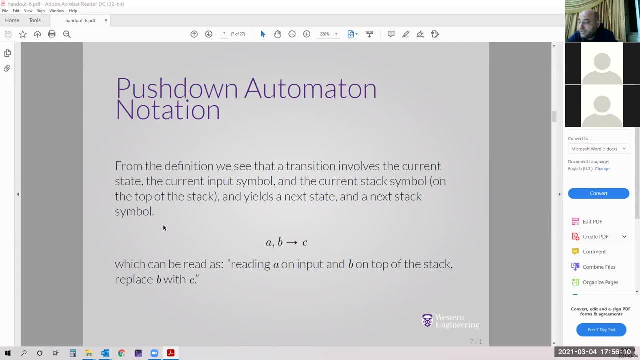 From the deformation we see that the transition involves the current state, the current input symbol and the current stack symbol in the top of the stack And yield a next state And next stack symbol. A and B will have the C, which can be read as reading x if to make the summon space. 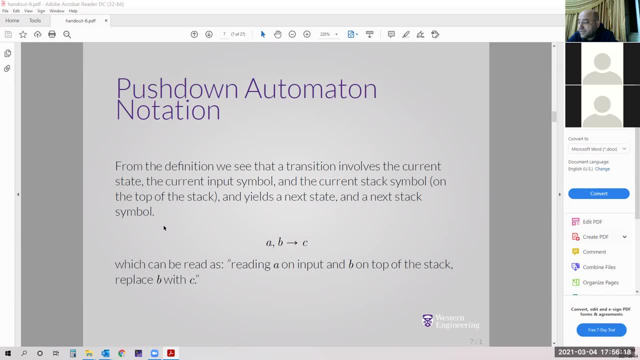 Remember SS stole mean, as an example, for a certain A on input and B on top of the stack. then will be replaced B with C Again, guys, what do we mean by this If I read A and B at the top symbol of the stack? 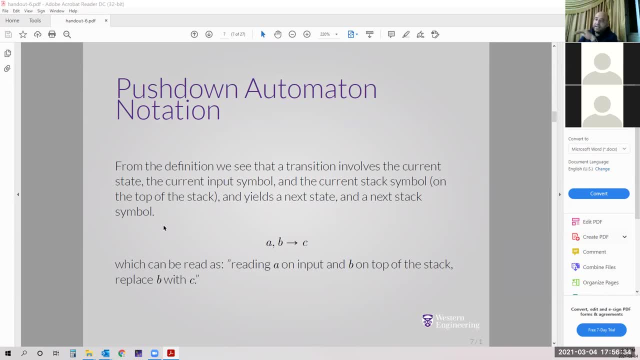 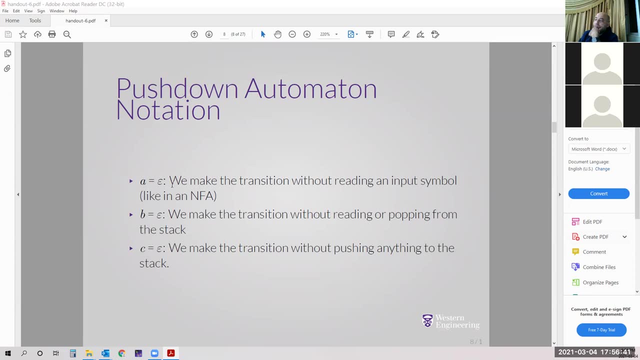 we replace B with C Because we are stacking symbols- A equal epsilon. we make a transition without reading an input symbol like an F, A B equal epsilon. we make the transition without reading or popping from the stack, Because the stack has two main operations: pop or push. 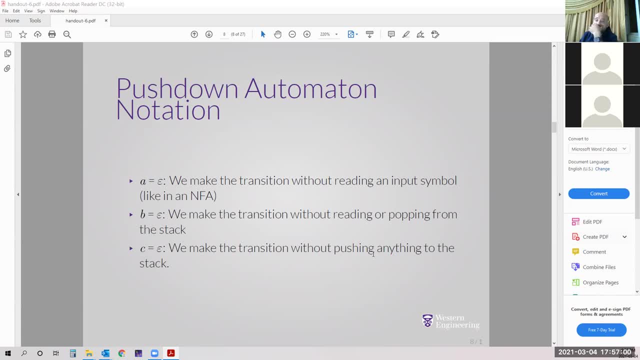 C equal epsilon, we make the transition without pushing anything to the stack. So these are the rules. If A is epsilon, we'll do the transition without input symbol. If B equal epsilon, we'll do the transition without popping any symbol from the stack. 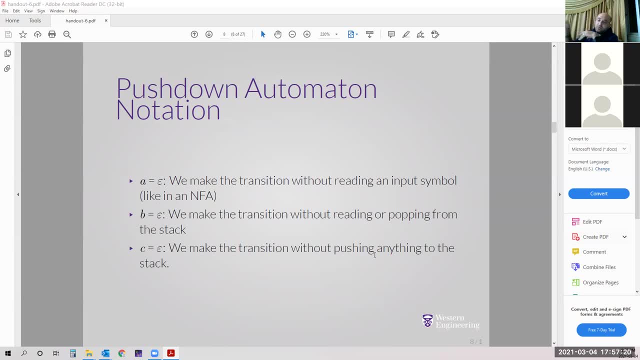 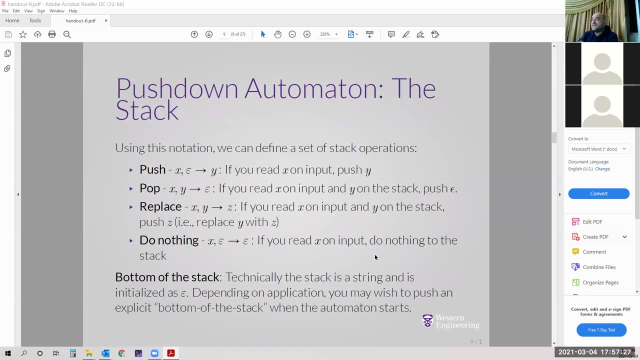 If C itself is the epsilon, we'll do the transition and we'll not push any new symbol to the stack, To the top of the stack. Using this notation we can define a set of stack operation: Push X, epsilon Y. If you read X on input, push Y immediately. 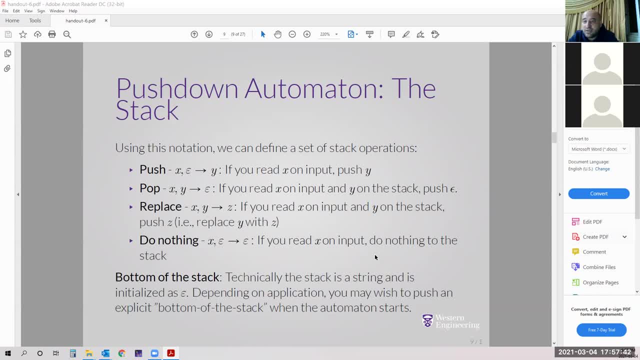 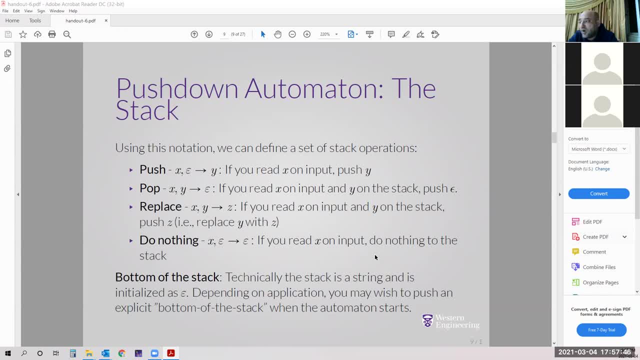 This is like the translation of what we said before. If we pop X and Y, if you read X on input and Y on the stack, push epsilon, which is literally push nothing. Replace X, Y, Z. If you read X on input and Y, 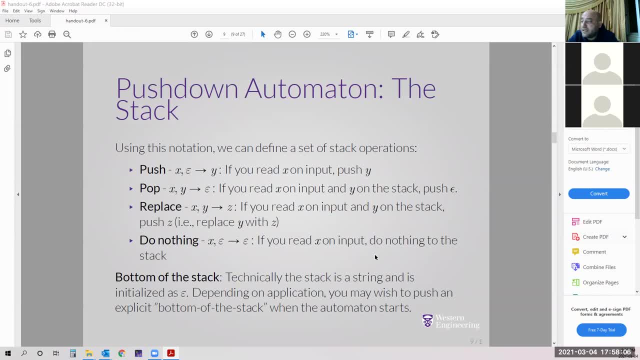 on the stack. push Z, Replace Y with Z, Do nothing. if X epsilon, then epsilon. If you read X on input, do nothing to the stack. bottom of the stack. technically the stack is a string is initialized as epsilon, so the 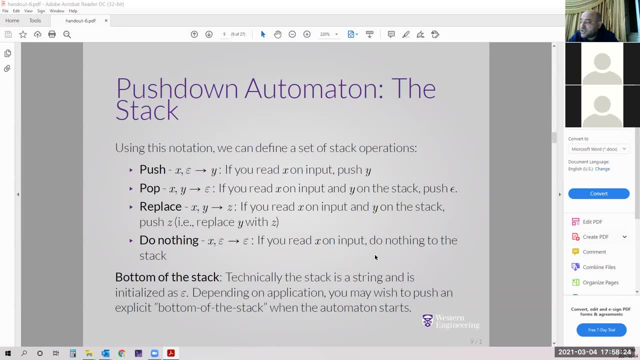 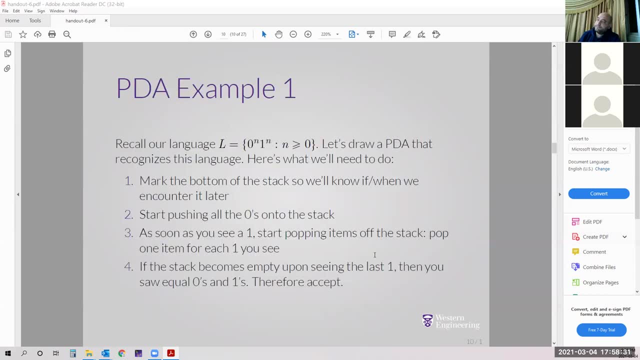 first symbol we push to the stack is epsilon. depending on application, you may wish to push an explicit bottom of the stack when automaton style push down automata. example one: recall our language: zero to the power n, one to the power n where n is greater or equal to zero. let's draw a PDA that recognize this language here. what we will need: 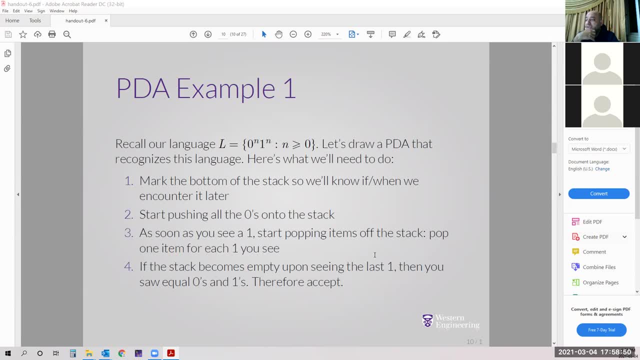 to do: mark the bottom of the stack so we'll know if, when we encounter it later, start pushing all the zeros onto the stack as soon you see a one, start popping items of the stack. pop one at the time for each one. you see. if the stack become empty upon seeing last one, then you 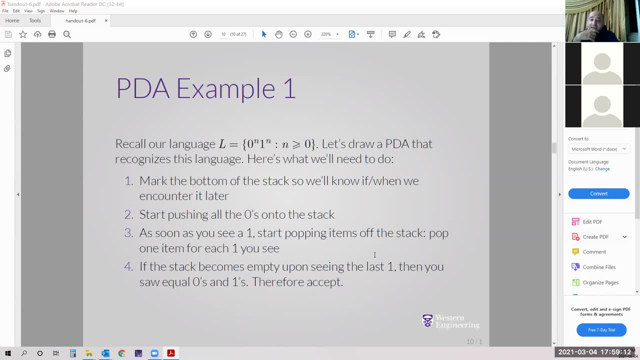 so equal number of zeros and number of one. then accept, what do we mean by this? in this example we push the zeros once we see now with each time, because the language consists of zeros first, then once we don't say zero, one star. it's different example here that our string or 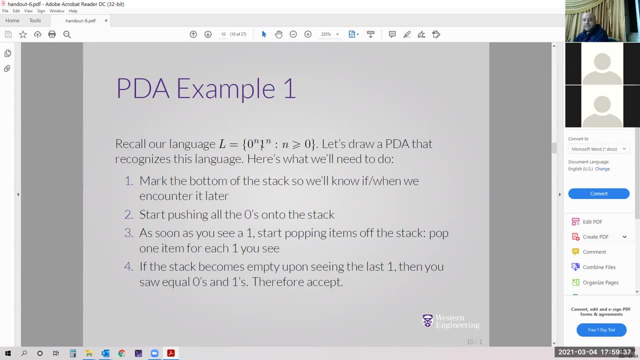 the language consists of zeros at the beginning, then once equal number. how i can accept this state? we will use the stack at each time. the push down automata will push zeros. once we see the first one will pop first zero, then second one will pop another zero. if we end at empty string, then 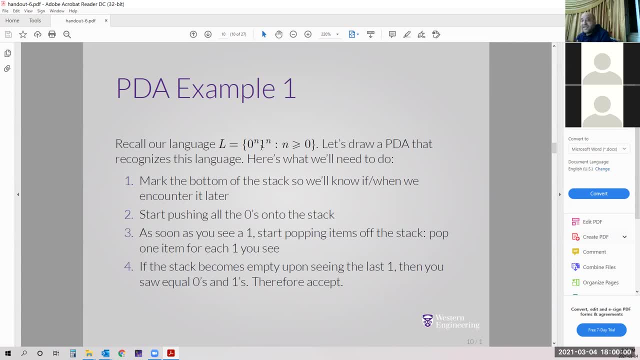 we'll accept which means that the number of zeros equal to the number of ones. if we still have remains ones or we still have remaining zeros in the stack that mean the number of zeros is not equal to the number of one, then we will reject that language. 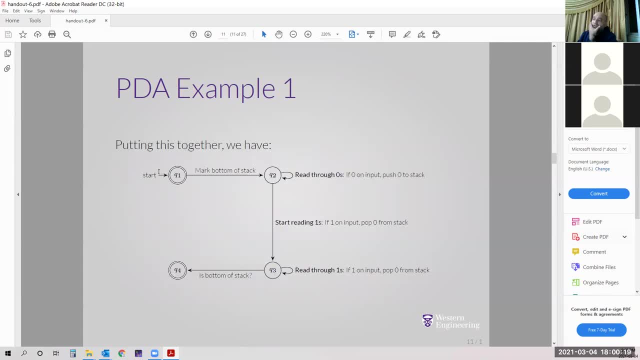 putting this together, we have start: q1- mark bottom of the stack with epsilon that this is the bottom of the stack. q2: read through zeros. if zeros on input puts zeros to the bottom two of zeros to the stack, Start reading ones If one on input. 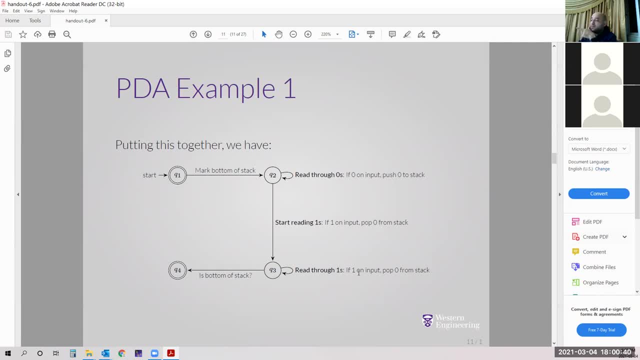 pop zero from the stack. Read through ones. If one on input pop zero from the stack, Is it the bottom of the stack? Yes, Accept, No, Reject. Clear guys, Clear, Okay, Okay R. rewritten in our transition notation. 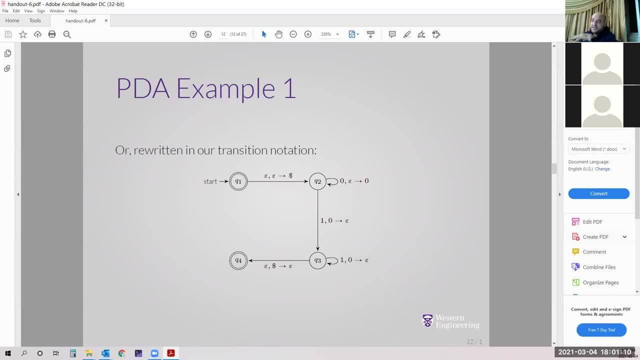 Y, Y- This is the first thing We push Y to the stack- or this sign which show me that this is the bottom of the stack. You said I don't want to put Y at the bottom of the stack You put: 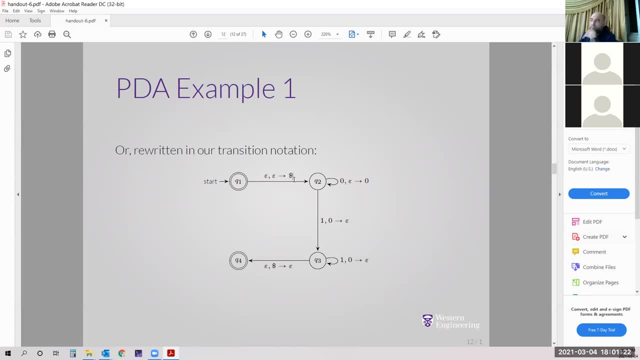 any other symbol to let the language know that this is the bottom of the stack. Then, if we receive a zero, push zero. Once we read one, pop zero and replace it with epsilon, which means make the cell empty. Then we read one also, pop another zero. 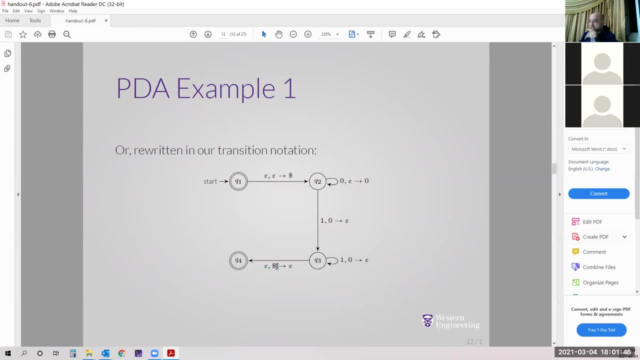 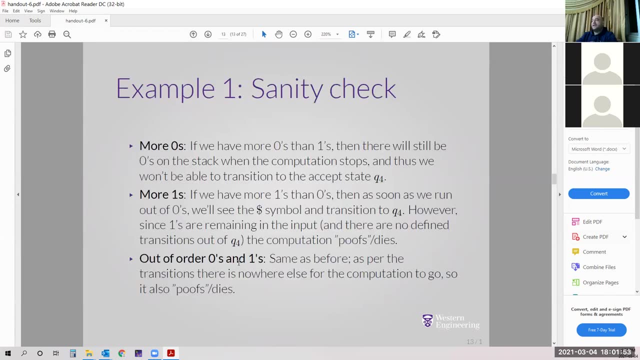 Is here. We reach to the state epsilon with this symbol and we replace it with epsilon. If yes, accept, Okay, More zeros. If we have more zeros than one, then there will still be zeros on the stack. This is what I 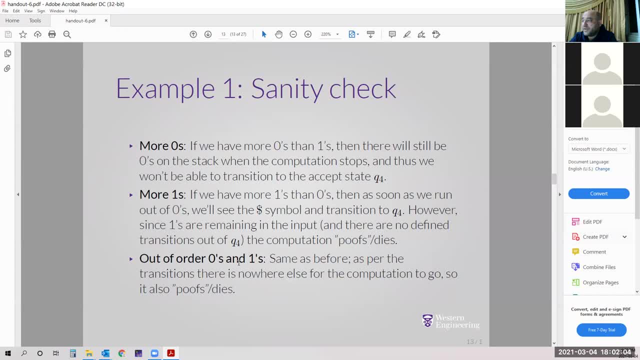 said before, When the computation is stopped and thus we won't be able to transition to the accepted state Q4. More ones. if we have more ones than zeros, then as soon as we run out of zeros, we'll see that a symbol and 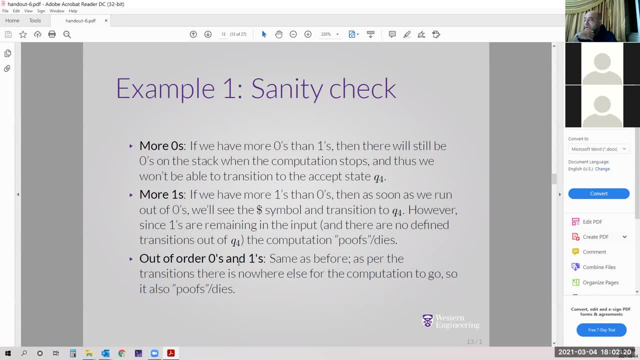 the transition to Q4.. However, since ones are remaining in the endpoint and not define the transition of Q4, the computational proof dies Out of order. zeros and one, same as before. As per the transition, there is now where else for the computation to. 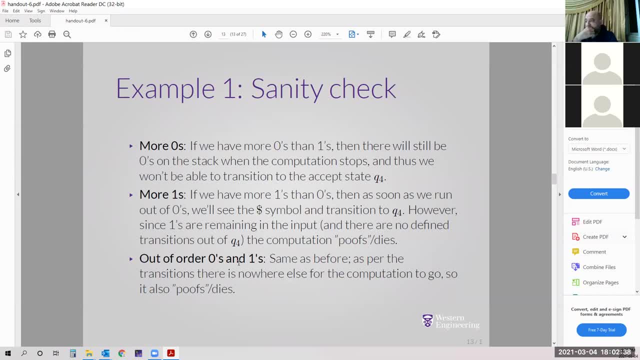 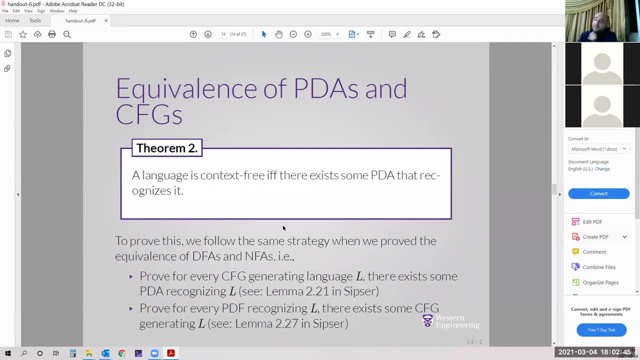 go, so it also proves dies or proofs. Now, equivalence of pushdown automators and context-free grammar. A language is a context-free grammar if there exists some pushdown automator that recognizes it To prove this. we will follow the same strategy when we 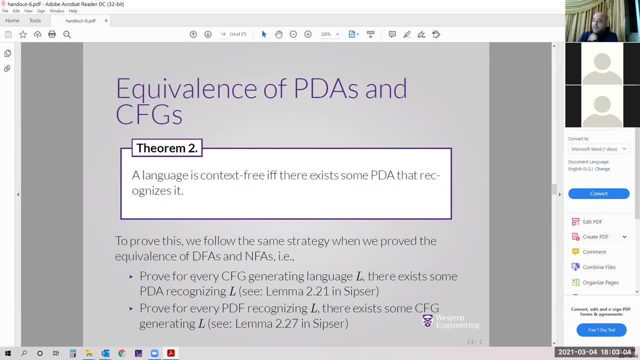 prove that the equivalence of DFA and NFA. Prove that every CFG generating the language L, there exists some. PDA recognized L C, lemma 2.2 in our textbook spicer, A proof for every PDF recognizing L, there exists some. 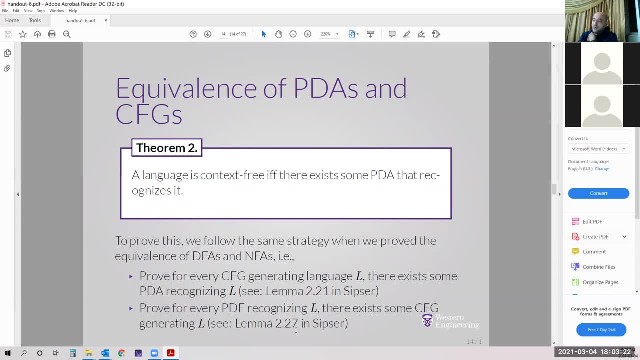 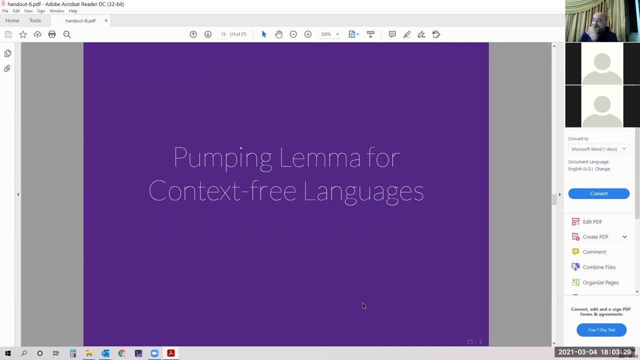 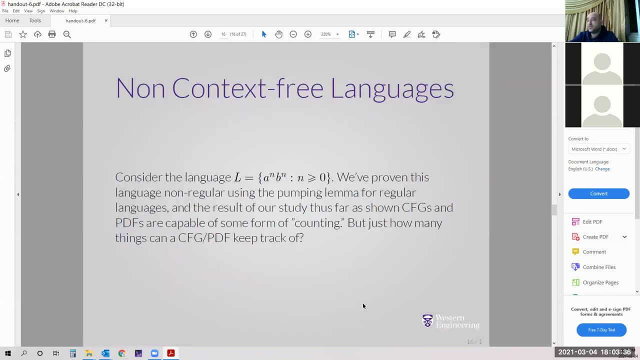 CFG generating L C lemma 2.27 in spicer Or spicer Pumping lemma for context-free grammar. You love pumping lemma right. Non-context-free language. Consider the language A to the power n, B to the power n where n is greater. 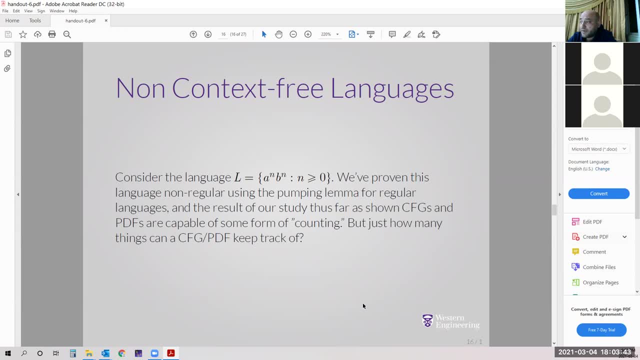 than zero. We prove in this language is non-regular using the pumping lemma for regular language and the result of our study thus far, as shown as CFG and PDF are capable of some form of counting. But just how many things can CFG or pushdown? 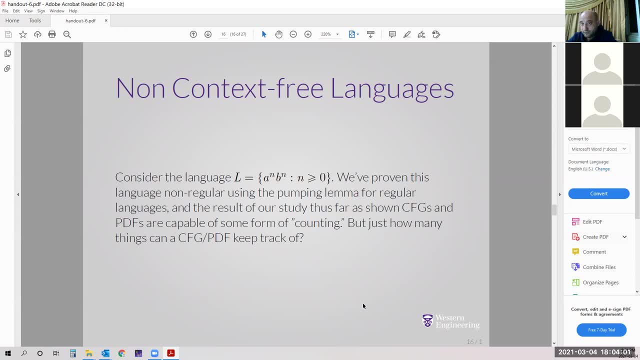 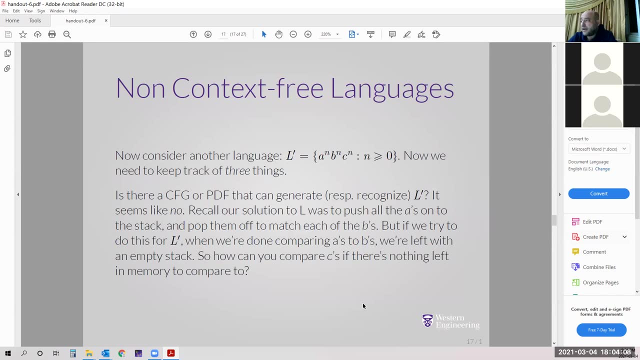 keep track of? Can we consider all situation? Of course not Now. consider another language: L prime A to the power n, B to the power n C to the power n n greater or equal to zero. Now we need to keep track of three things. 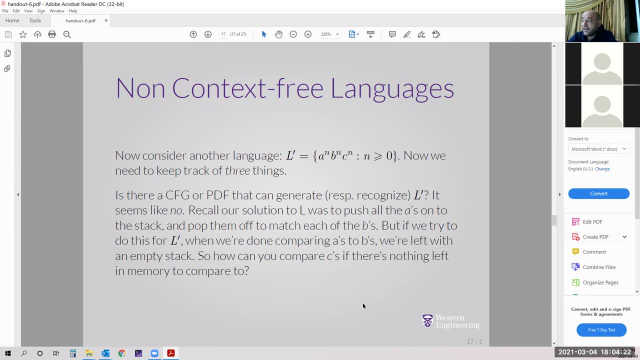 Is there a CFG or a PDF that can generate or recognize L prime? It seems like no Recognize L prime. It seems like no Recognize L prime While we're talking about L or ainte Staffunes. How can we compare C's? 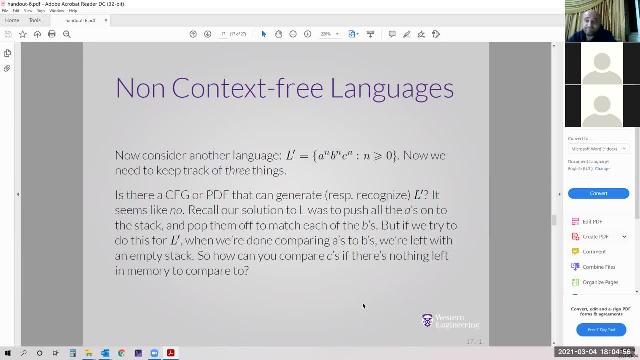 If there is nothing left in memory to compare to. So if we compare two thing, can't do it in a stack. But if I compare three things, first I will compare A's and B's, then how I can compare them with C's. 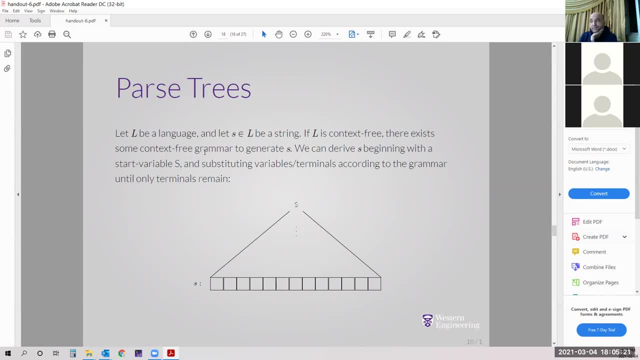 Parsetry. Here we'll have that, what we call parsetry. Let L be language and let S be belong to that string. If L is a context-free, there exists some context-free grammar to generate S. We can derive S beginning with a start variable. 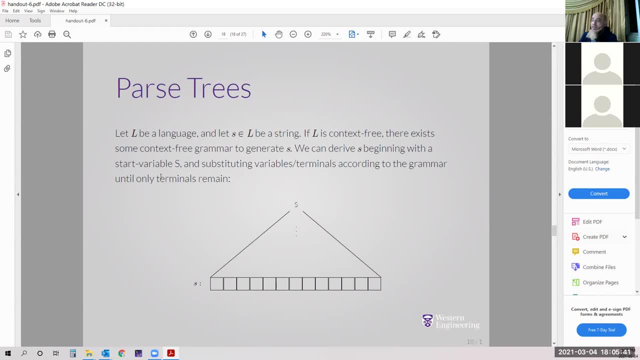 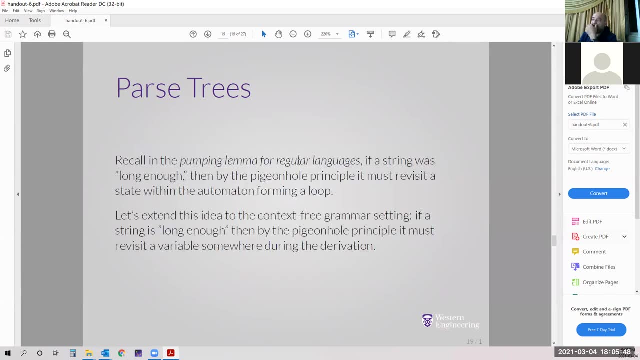 S and substituting variables or terminals according to the grammar, until only terminals remain. Recall in the pumping lemma for regular language: If a string was long enough, then by the pigeonhole principle it must be a string. It must be a string. 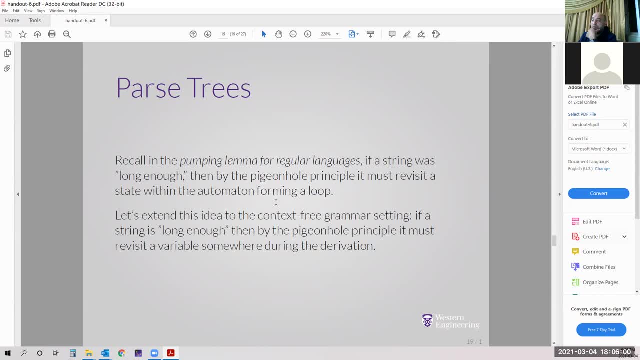 It must revisit a state within the automaton forming a loop. Let's extend this idea to the context-free grammar stating: if a string is long enough, then by the pigeonhole principle it must revisit a variable somewhere during the derivation. Same principle. Consider the following grammar: 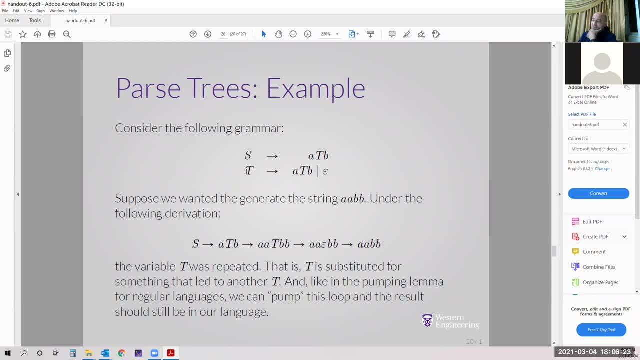 If we have S A T B T, either could be A T B T, either could be A T B T, either could be A and then B or epsilon. Suppose we want to generate the string AABB. 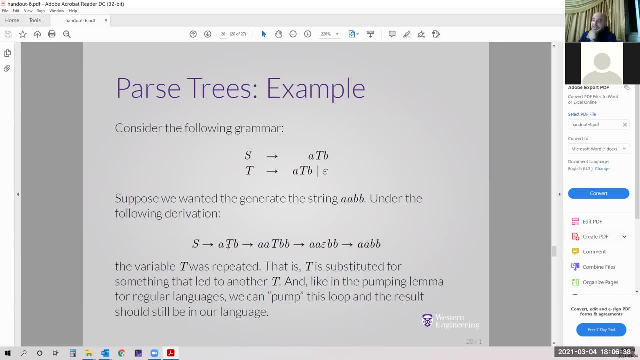 under the following derivation: S will give me ATB, then a, A, T, B, B, Then we replace the T with epsilon, Then it will be AABB. The variability was repeated, that is, T is substituted for something that led to another T. 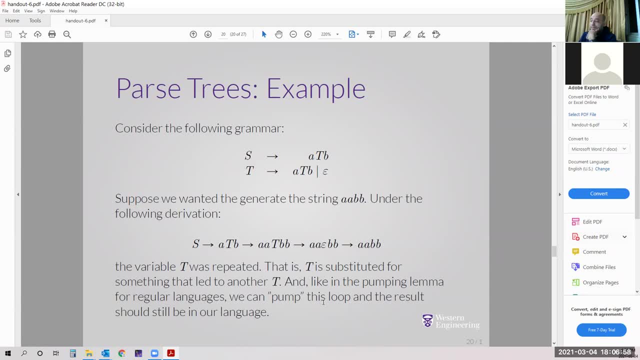 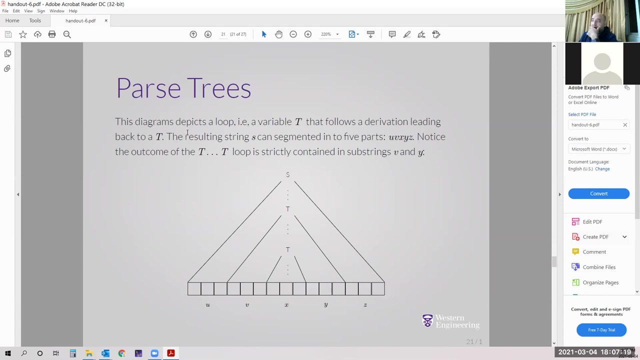 And like in the pumping lemma for regular language, we can pump this loop and the result should still be in our language. but with regular language we use, with pumping lemma, x, y, z. here we'll use five symbols. we'll see the diagram depicts a loop, a variable t that follows a derivation leading. 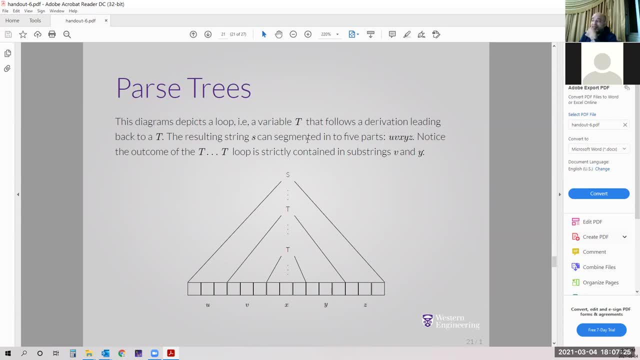 back to a t. the resulting string s can be segmented into five parts: u, v, x, y and z. u, v, x, y and z. this is what we know before. here we add a, u, v, another two parts. notice that outcome of t to t loop is strictly continue, contained in substring v and u. so here we have s, t, t. 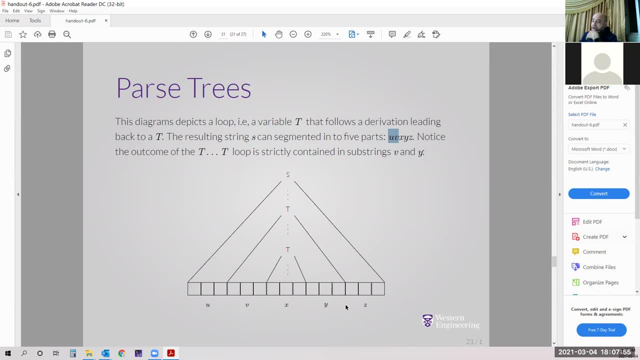 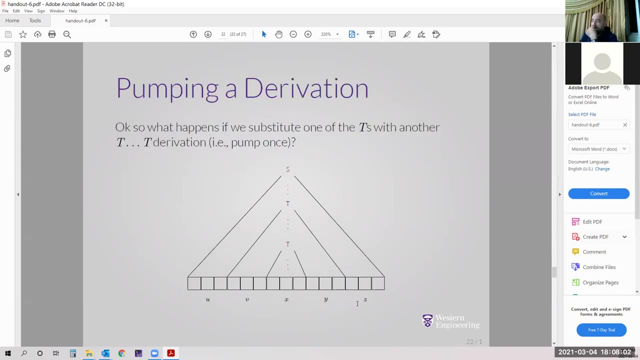 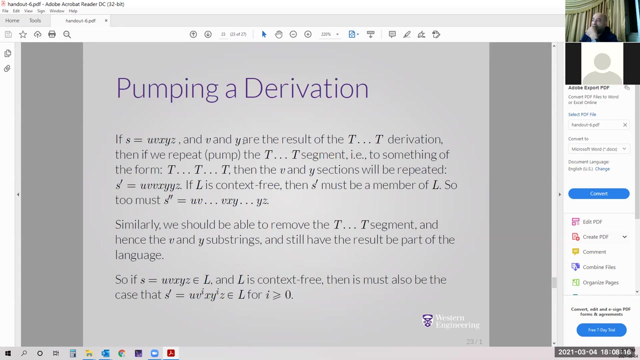 here we can call it u, v, x, y and z in the parse tree: pumping derivation. okay, so what happened if we substitute one of the t's with another t to t derivation, we pump it one if s equal u, v, x, y and z and v and y are the result of t to t derivation. then if we repeat: 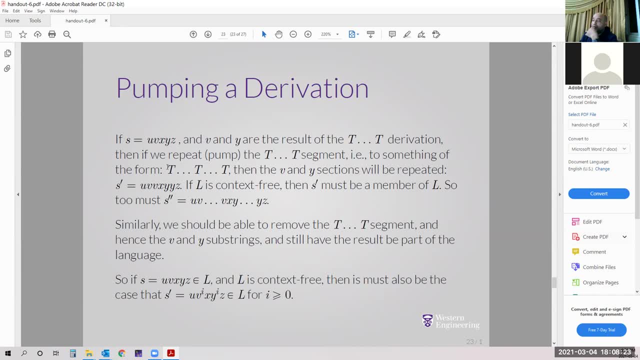 pump the t, t segment to something of the form of t, t, t, then v, y section will be repeated and we'll have here u v, v, x, y, y, z. if l is a context free, then s prime must be a member of l. so two more, that s double prime: u v. 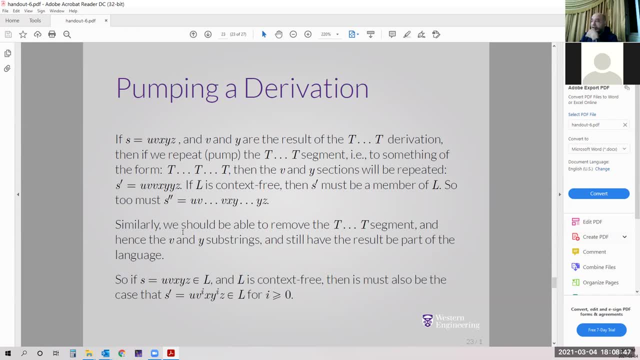 to v, x, y, then y, z. similarly, we should be able to remove t to t segment and hence v and y segmented string, and still have the result be a part of the language. so if s, u, v, x, y, z belongs to l and l is a, 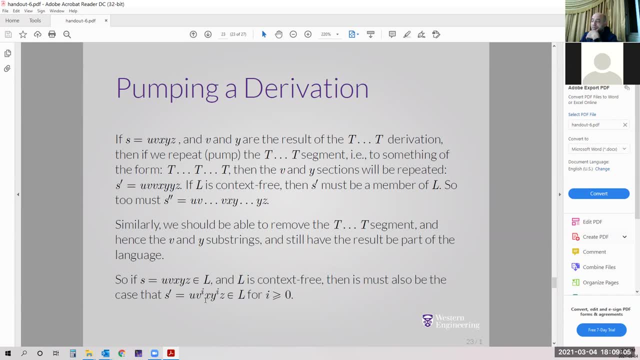 context free, then it must be also a case as a prime that u, v to the power i, x, y to the power i, z. if you remember, before we use these three here we add u v. i belongs to l for all i greater or equal to zero. 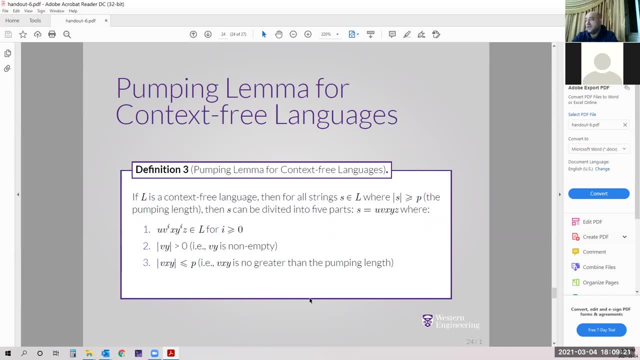 we will solve a lot of questions, don't worry. so here: what is the rule of pumping lemma l? if l is a context-free language, then for all strings l s belongs to l. where the length of s greater than the pumping length p, then s can be divided into five parts: s, u, v, x, y and z. where u, v, i, x, y to the power. 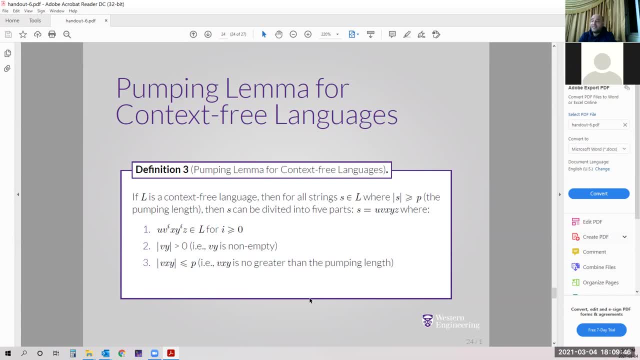 belongs to l for all i belong. greater or equal zero the length of v- y greater or equal to zero mass, so it's not empty. it's not empty, not only greater than zero, it couldn't be a zero. and v x- y less or equal the length of it, the p, which is the pumping length, so is no greater than. 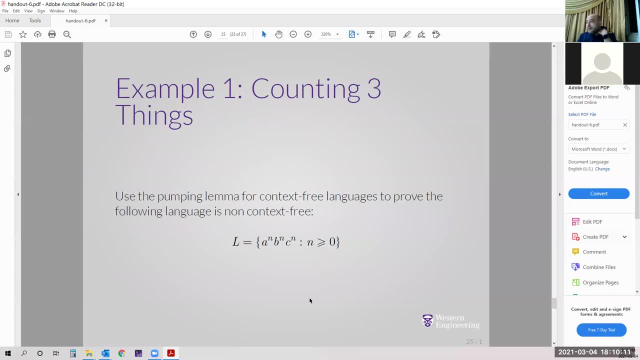 pumping length. so this is our example that we talk about: a to the power n, b to the power n and c to the power n is greater or equal to zero. example two: we will- that we will have next class- use the pumping lemma for context, free language to prove. 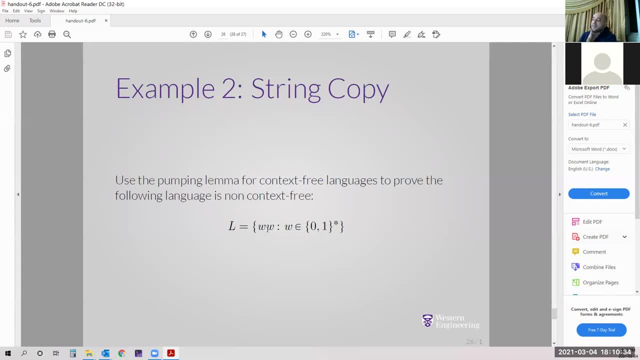 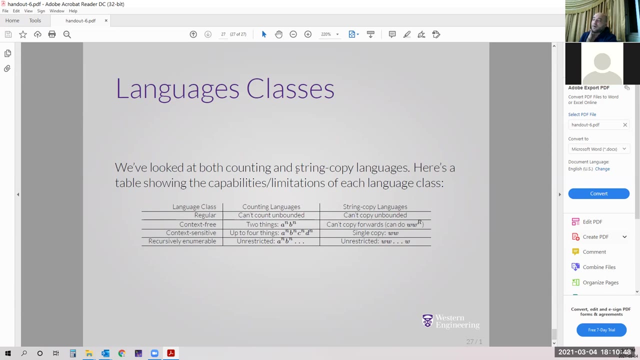 that the following language is not context free: w. w where w belong to zero one star, so we will prove this also. is not context free language. now, language is classes. we have looked at both continuing the counting and the string copy languages. here is table showing the capabilities and limitation. 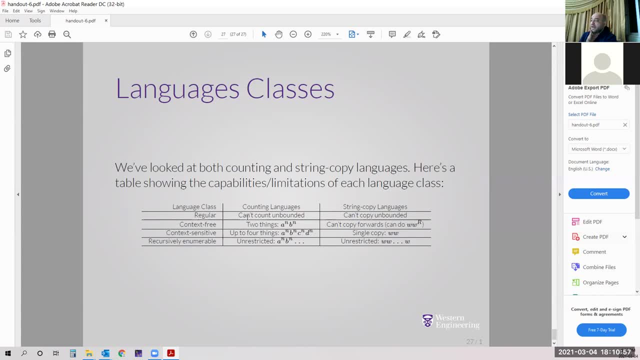 of each language class. if we have a regular cannot count or unbounded we don't cannot do counting with dfa and nfa and regular expression, also with the string copy languages. we cannot context free two things. we can do it, but we cannot copy forward like w? w to the power r context sensitive. 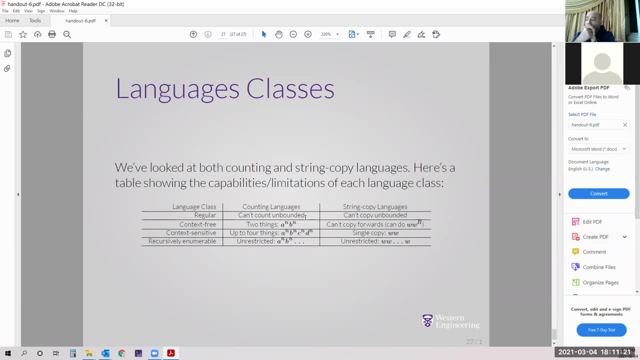 context-sensitive, even even beforehand, and different. it will be solved also with the recursively enumerable. but also this other part with the string copy languages is outside of our course of scopes. so So those two things, This one and this one, is not part of our course. 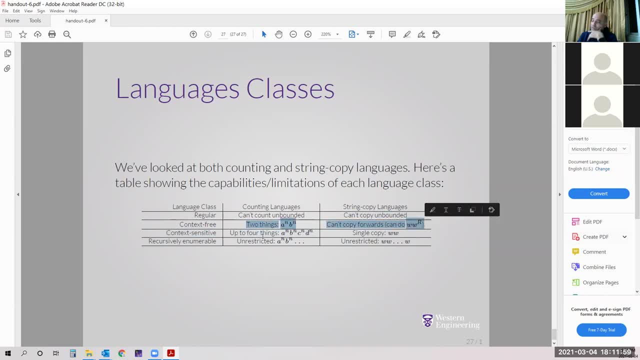 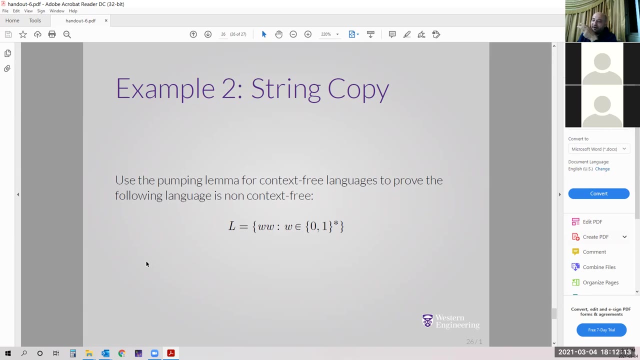 So Tomorrow we'll have those and we'll talk about Turing machines. OK, I'll stop here And I'll not, because we still have only 15 minutes of the class, Or literally eight minutes, because each hour equal to 15 minutes and 10 minutes break. 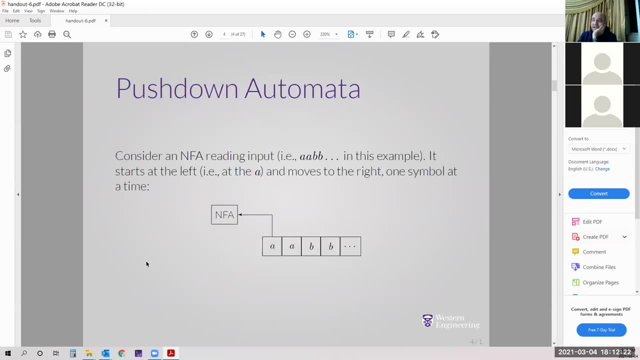 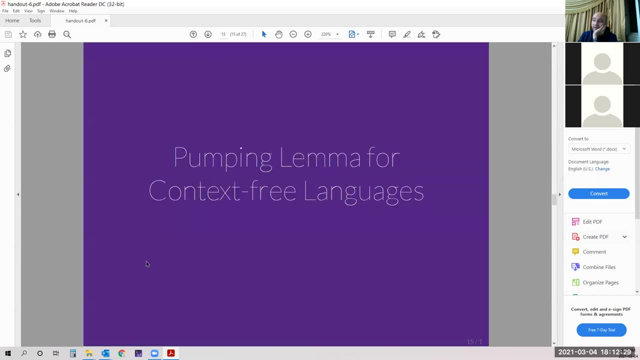 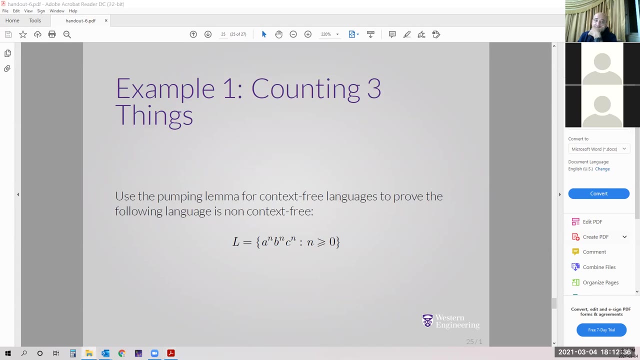 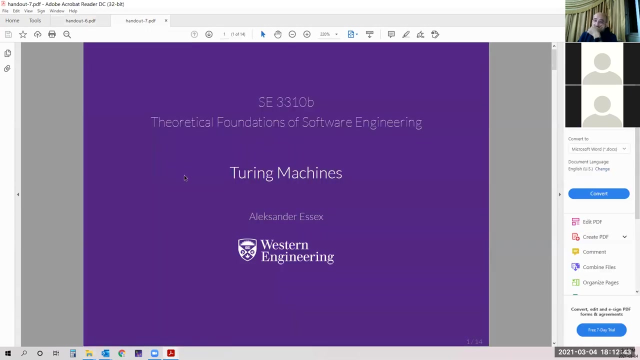 So I don't have enough time to start with class, not seven. that will solve all these things, with example for push down automata, Then we'll have a couple of example about pumping lima, Then we'll move to hand out seven tomorrow, Which is the Turing machines. 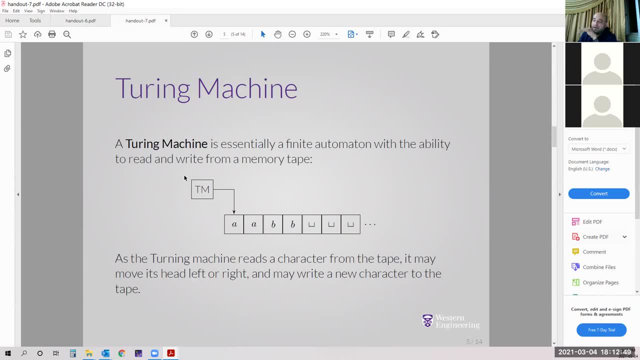 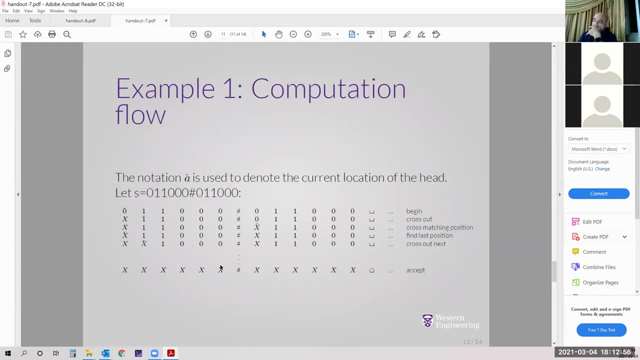 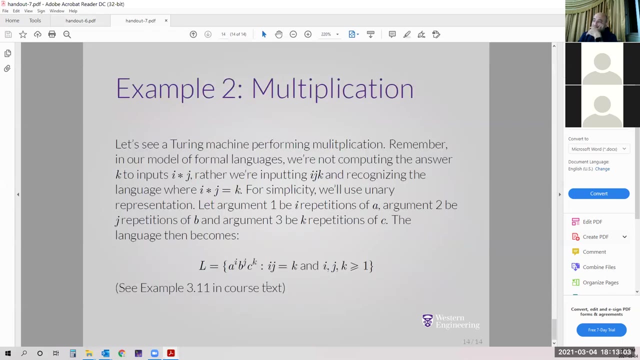 In Turing machine we have some Memory places and we can move left and right, which will solve something different. But- And we'll have here some examples, Under the state of transition, with all these things- and we will See example of it, to the poor IB, to the port JC, to the park, a, this example of multiplication of these things could be happen using Turing machine. 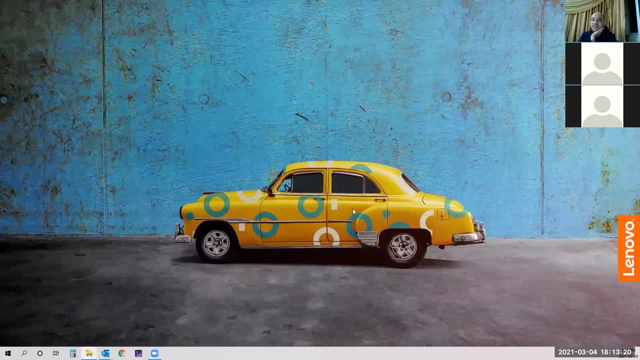 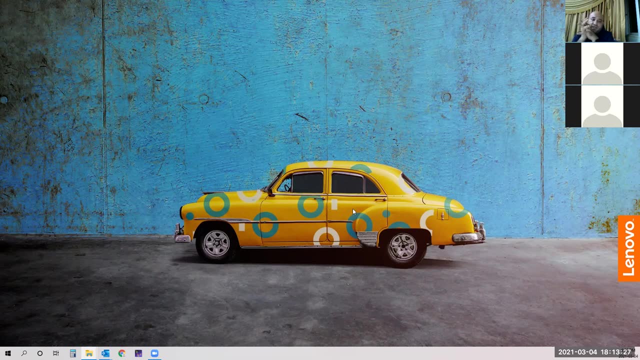 And by end of tomorrow Or Saturday we will release assignment three And we'll be On The queue And we'll still have like eight, nine, 10 and 11 and 12, but they are short hand out and simple handouts. 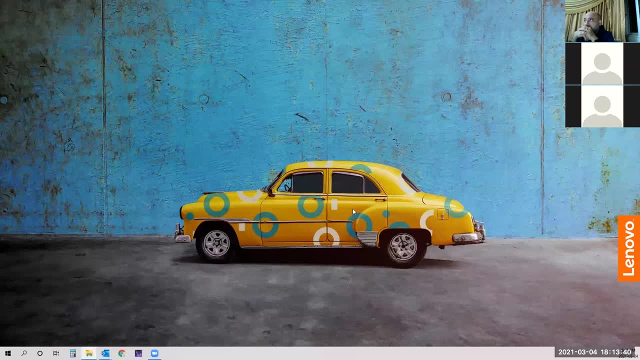 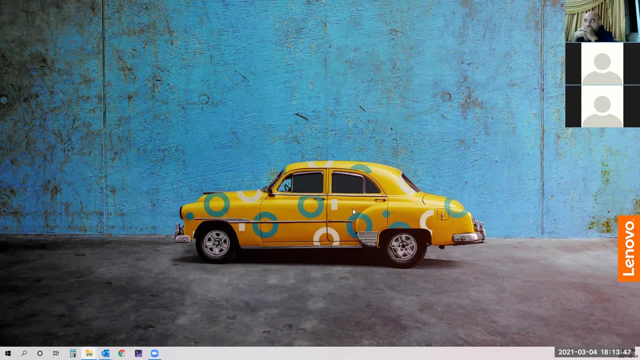 See you tomorrow. guys, Have a great night. If there is any question, you can stay, If you don't have a question, you can leave, And we'll see you tomorrow. And we'll see you tomorrow. Bye, Bye. 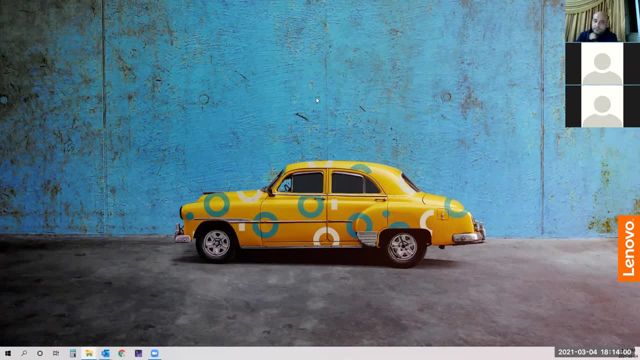 Bye, Hi, I have a question, Yep. Um, it was related to One of the slides you had up Not that long ago where you're saying: How can we make the state model for A language Like if it was a to the end, B to NC to the end? 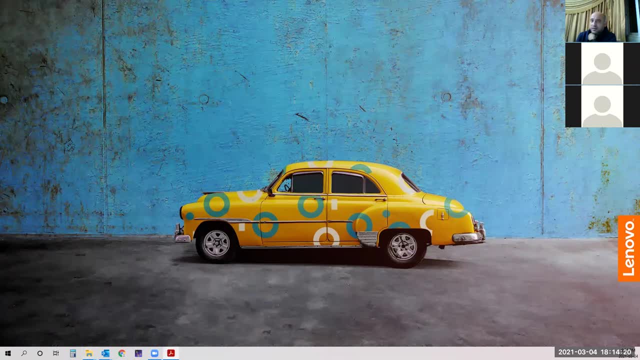 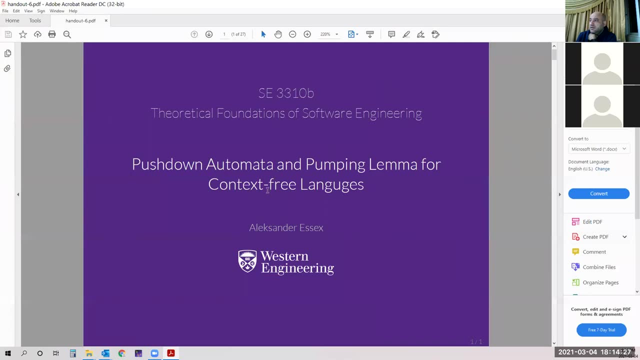 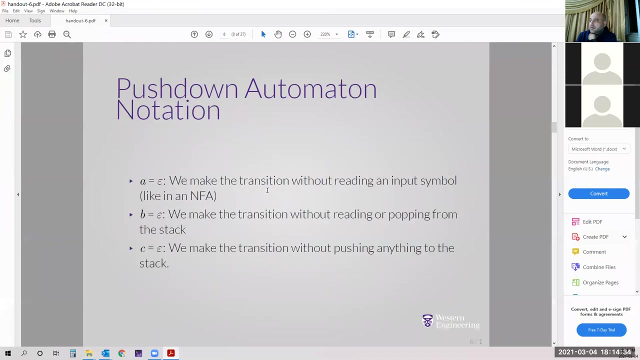 And You can't Just Just Set that up, Can you see? Yeah, Yeah, Yeah. Next one: It was Yeah, So this one, Oh yeah, Could you go back there? So for this one we had. 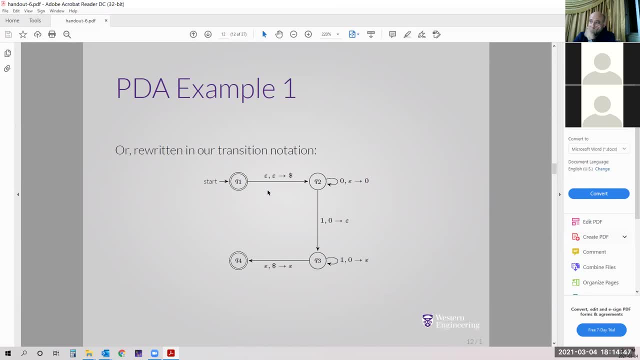 Is basically just a and B And making sure that the two Were there The same size, Yeah, But in the transition between Q2 and Q3. You put the Empty string onto the stack and that kind of Well that empties the stack. 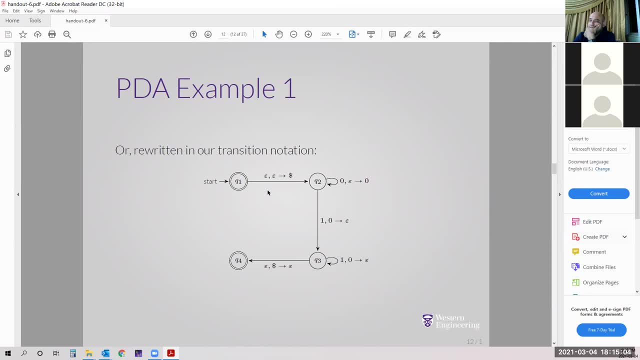 But so what if, instead of that empty string, you put in The input Into the stack, So then You could kind of keep Count of that one. So if it was A to the A to the end, B to the end, C to the end? 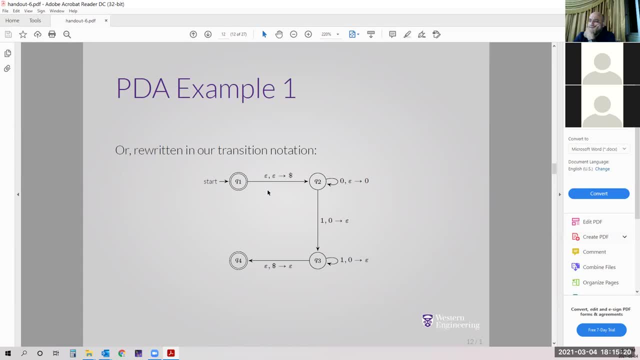 Then you put A onto the stack And then make sure that A and B are the same Number And then, while you're doing that, you push B onto the stack. How you can do that, Can you tell me How you can? 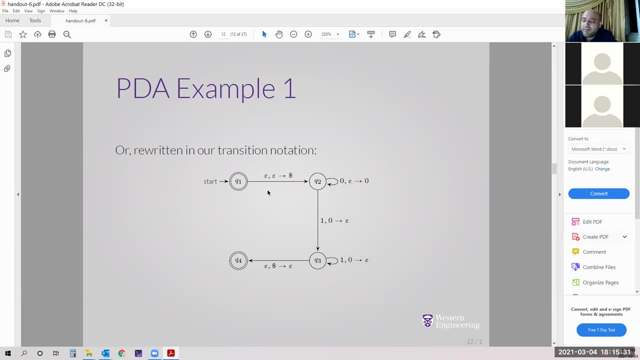 Three numbers Or three components They are. So I was thinking: Okay, Well, could you, You can, Yeah, Okay, Because, Okay, So So, So, So, So So So, Because I think 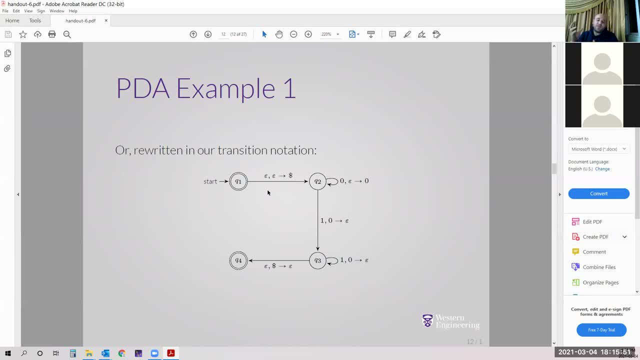 I'm right. But if you cannot go left and right because you know the stack First and last serve, So how I can put a, B or C and I count, And I can't how I can do two. If you can do two pops in the stack with one. 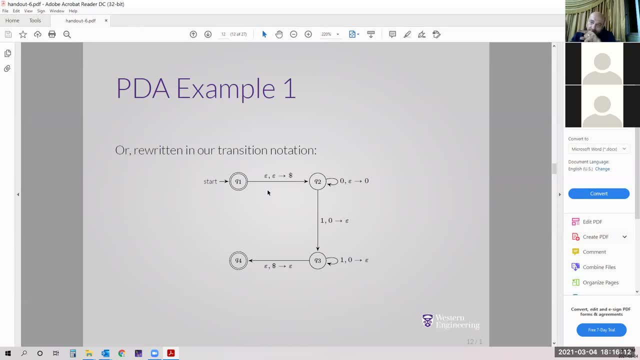 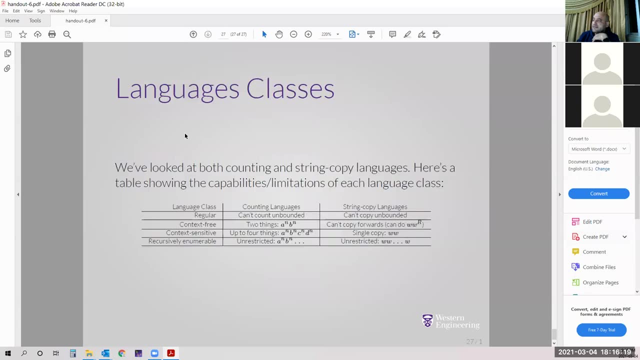 But how do you make sure that they are after each another? you cannot. so that's why I told you in handout 6 that with this model I can't compare because I'm using stack. I can't compare two components, so I think I go to Quintex sensitive. 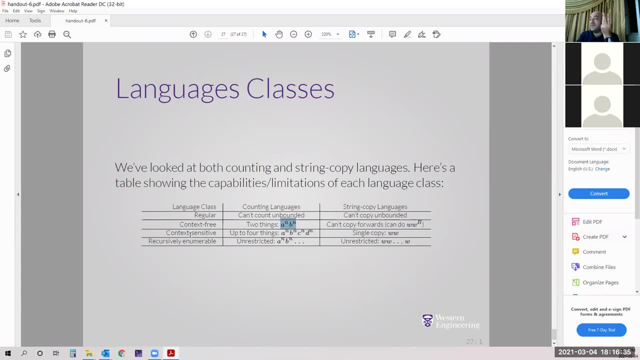 I have a memory, I have a counter here. I just have a counter, two counters, okay, okay. so, yeah, I have multiple counters, so I can't solve it. it's solved computationally, it's solved and what you're saying is correct, but not with the stack structure. 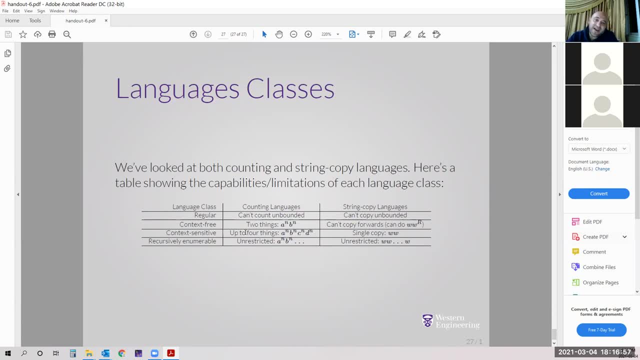 okay with random memory structure. yes, yeah, what about with each symbol? I save the address of it and I check with the list of addresses I have, with the list of memory addresses I have in hexadecimals that I have this symbol. then I can make and. 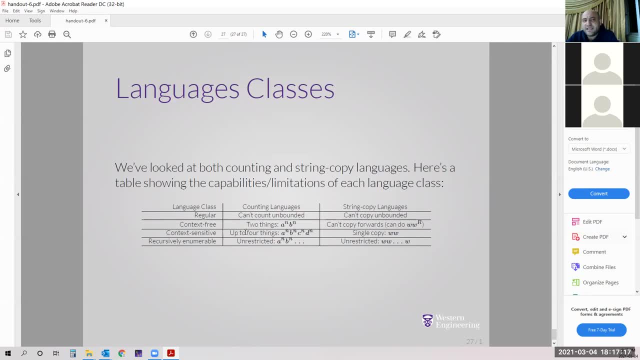 I can make, like you know, in in C++, if you said, let's C equals zero, A equals zero and B equals zero, and every time you read an A and B you add your counter and each time you pop A or B or you at the end you can check. 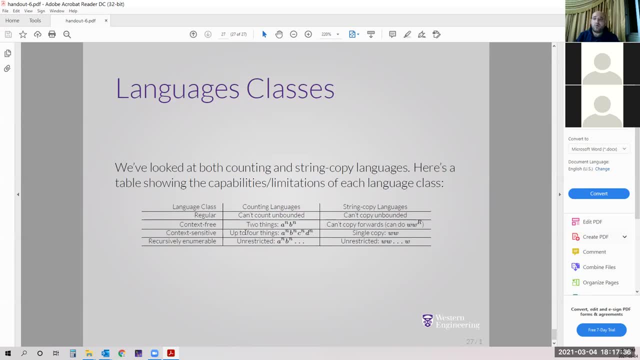 is the number of A equal the number of B or equal the number of C? yes or no? yeah, okay, okay, yeah, I think, yeah, that makes sense. and so with random memory access I can't do it, but with stack structure I cannot, okay, and so then what about in the 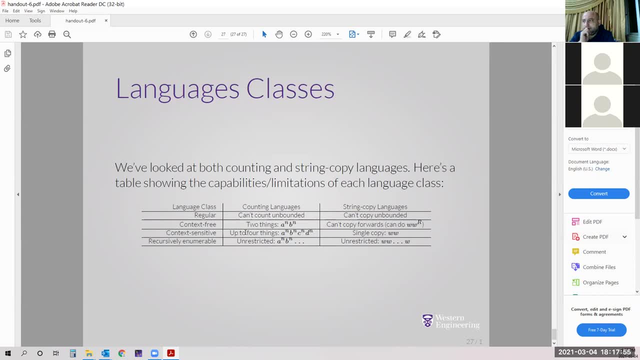 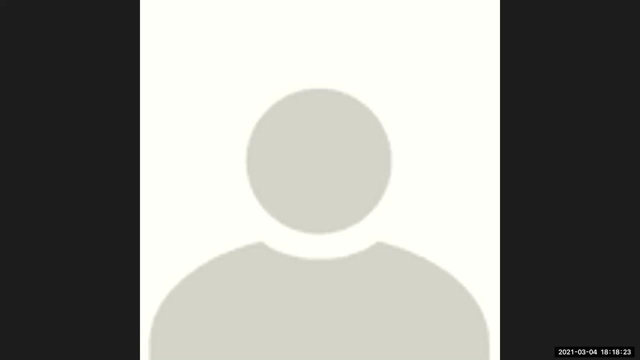 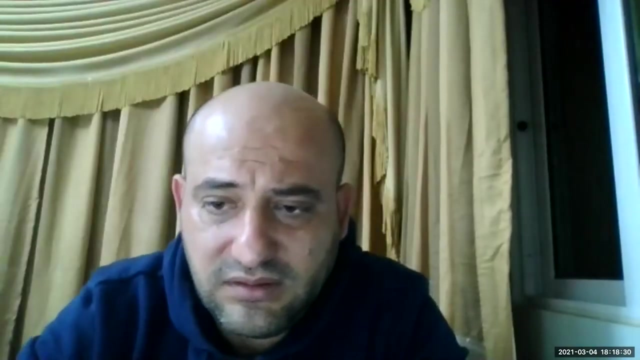 recursively enumerable. could you do the same thing if you had A to the N and then B to the M, for example? we will see tomorrow, okay, okay, thanks, okay, have a good day. okay for today. okay, Danielle, go ahead. hi, I submitted an SRA for the quiz one. 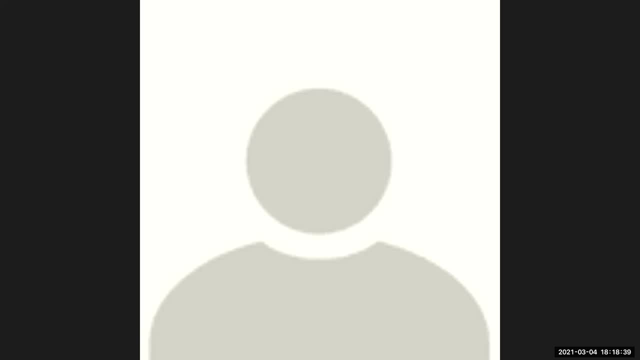 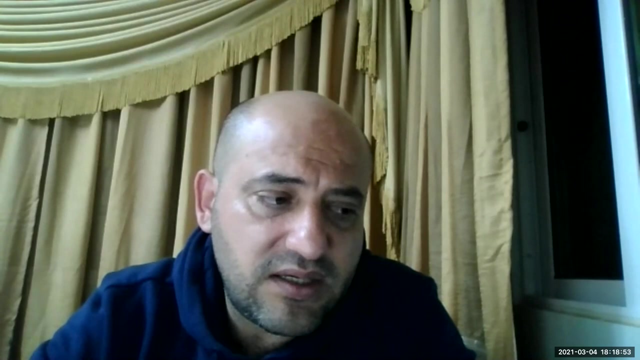 is there makeup for that? or would there just be a shift in the percentage? what do you mean? uh, the self-reported absence? i submitted one for. yeah, for those self-reported absence there is no shift for the marks. i will assign a time slot, but i was waiting the students because they 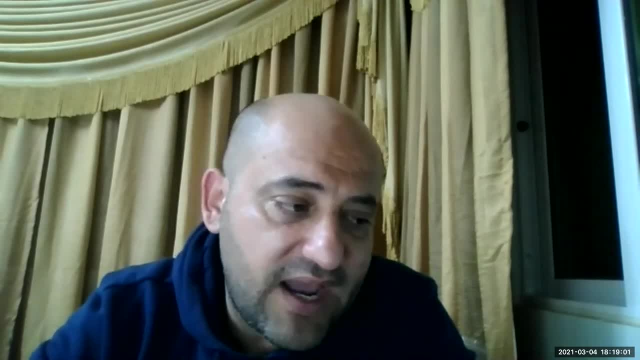 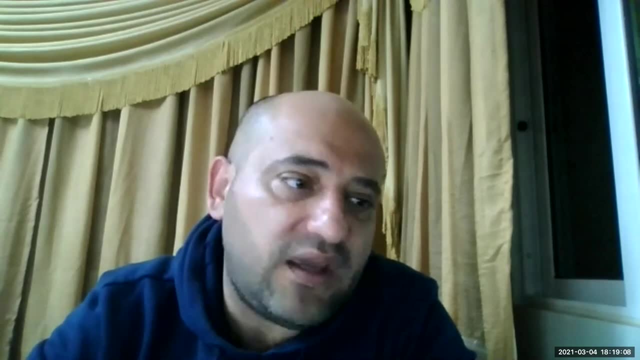 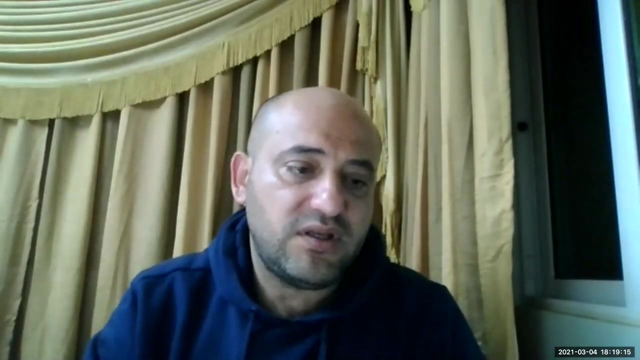 give them like 48 hours to report their absent and they have 48 hours to contact the instructors. you know, and if you consider, if we consider the weekend, i don't want it to be, you know, very strict with my students, so i consider saturday and sunday are not part of those. so today is the end. 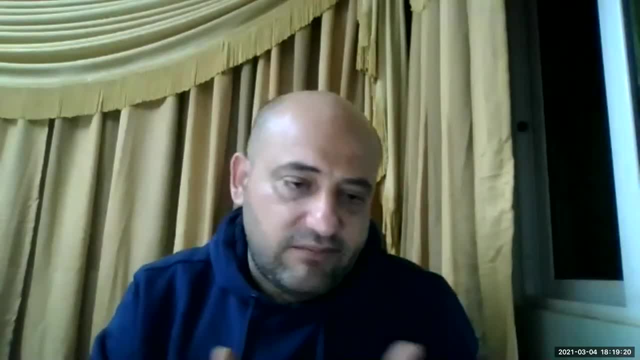 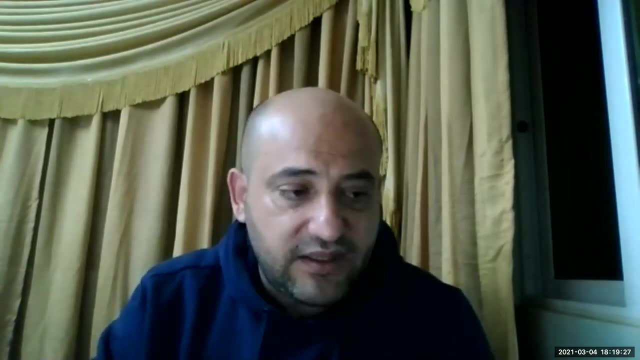 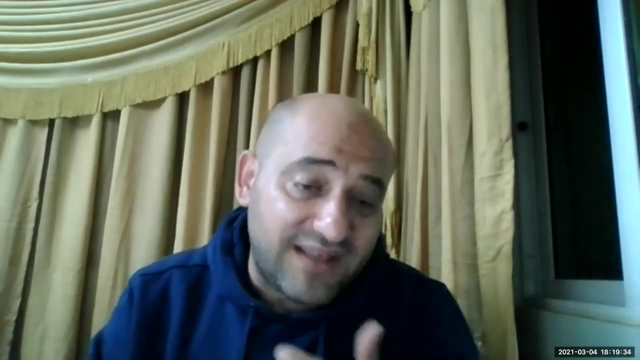 of the 40, the second 48 hours i like, if they like it wasn't a friday. so if they did report the absence on a tuesday, because the first 48 hours end in a tuesday, then they have the 48 hours to contact me. so they have till end of today. so by tomorrow i will make the full thing. then i will. 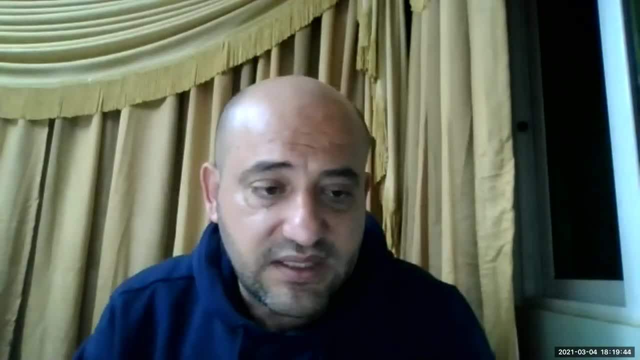 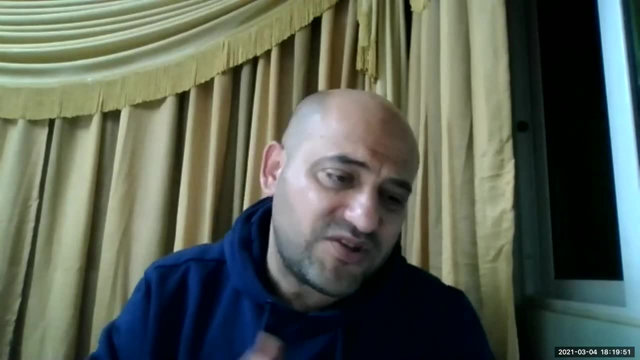 send an email for you, those who have the self-reported absence, or for those who have certain situation or medical leave and they use this leave instead of self-reported absence, because you know you have two chance of self-reported absence. some student will make it for something, not the quiz, maybe something better.